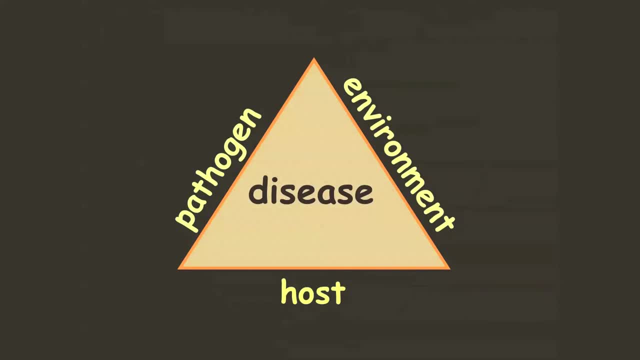 Coming back to the sort of the old, everyone who's had any plant pathology will remember the disease triangle, and I want to point this out in the context of the soil environment and soil health. To have a disease, you have to have the pathogen. 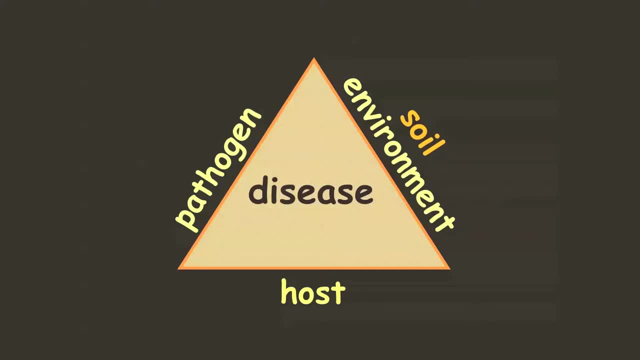 You have to have the pathogen present. you have to have the pathogen present- sorry, the host present and a susceptible host- And you have to have the environment that's conducive to that disease. The more pathogen that's present, the more susceptible the host and the more conducive that environment. 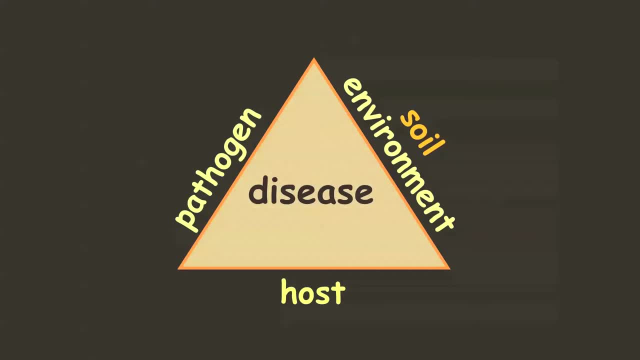 the greater the size of that triangle. So the length of each side represents the amount of that factor that contributes towards the size of that triangle. If you can reduce the favorability of that environment, for example by improving your soil health, you make a smaller triangle. 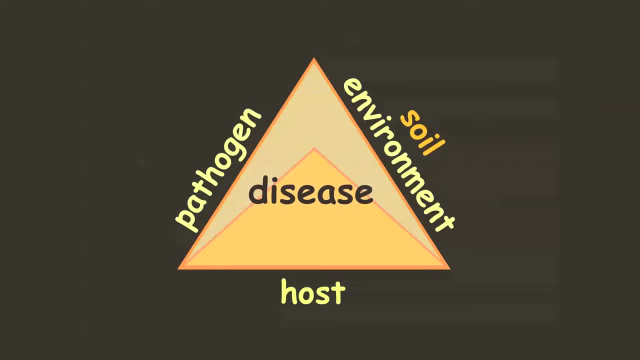 Which means represents smaller disease, less disease. If you can reduce the susceptibility of that host by selecting a cultivar, you reduce that size of the triangle. you get a smaller triangle. So that's the concept of the disease triangle In the context of soil health we're looking at in particular, trying to adjust. 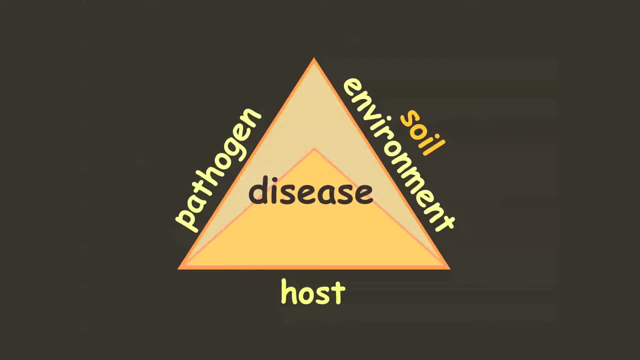 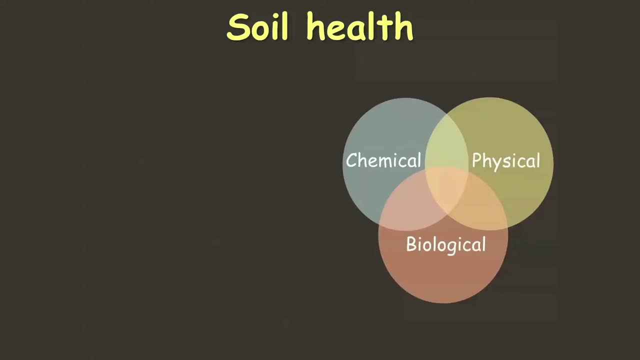 get the cursor up here- the soil environment, to get that side of the triangle smaller and create a smaller triangle, which means less disease and higher yield, hopefully. So let's go back to this concept of the various complexities of that contribute towards soil health. 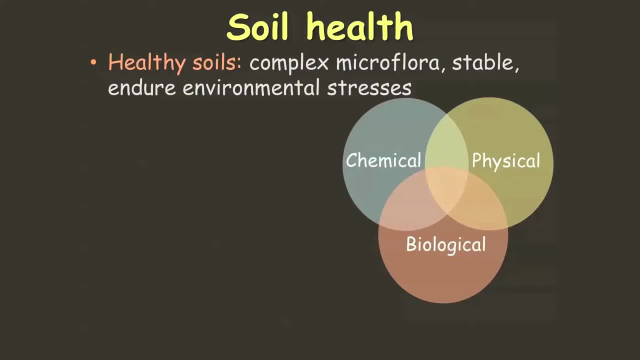 It is complex And in healthy soils it tends to be quite a diverse set of microflora. They tend to be in a fairly stable but fluctuating state, that is, can endure environmental stresses, whether they be moisture stress, heat stress, nutritional stress. 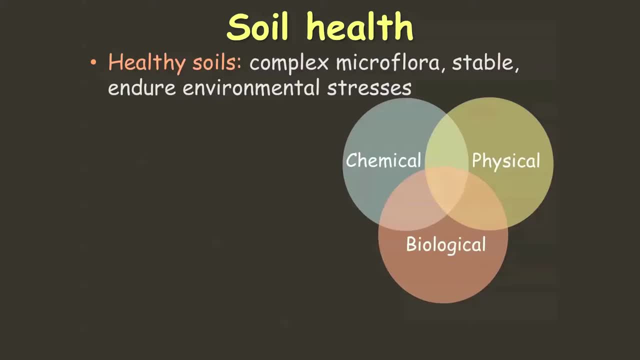 Healthy soils have a greater robustness And that's important because that conveys to the ability of the plant to withstand these kinds of stresses and, in particular, diseases. Unfortunately, it's just by nature of the game: agriculture basically interacts and in some degree messes up that robustness and stability. 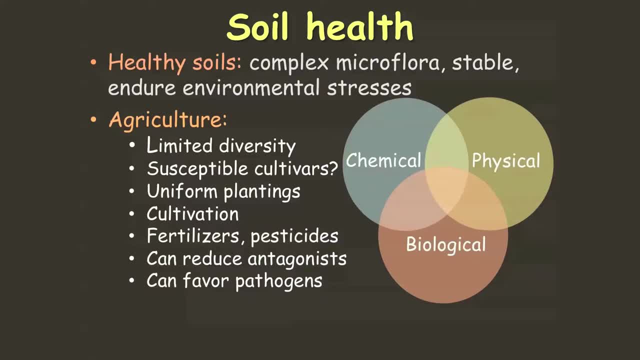 because we are cultivating, We are putting in fertilizers or pesticides And all of these things. whether it be the limited diversity that goes on in a particular field, it's one species. usually it may be a very susceptible cultivar if there isn't resistance to particular diseases of concern. 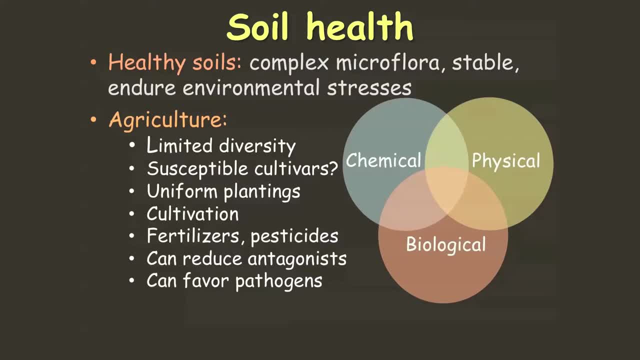 the wide scale of some of these crops, the degree of cultivation that disturbs the soil, the addition of synthetic fertilizers- sometimes they can shift the balance of microbes in that soil- the use of pesticides: that also will shift those microbes. Many of these practices can reduce the population of what we call antagonists. 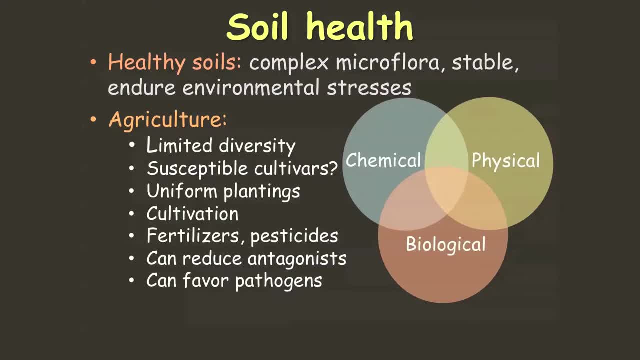 so beneficial microflora in the soil and favor the development of these pathogens, because you are interfering in that robust, complex, stable relationship that a healthy soil typically has, And that's just the nature of the game. If we want to go back to hunting and gathering, that's one extreme. 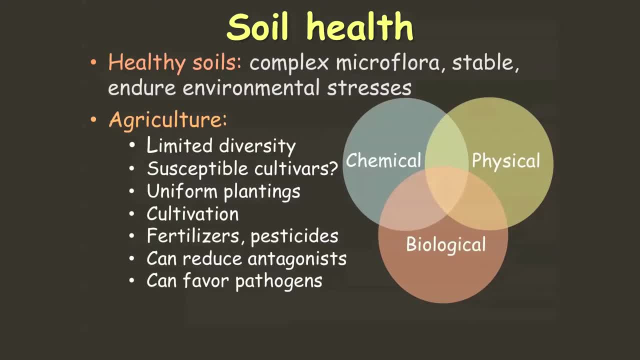 We have to deal with food production, So let's see what we can do within this context of recognizing those relationships. And so this brings up the title I was asked to speak about: is soil health for disease suppression? And so I'm going to use some examples from research we've done in my program. 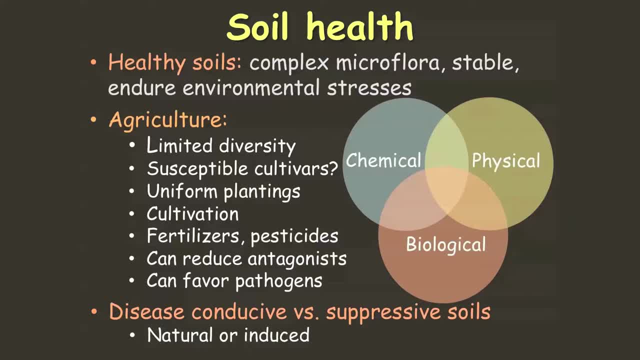 looking at soils that are very conducive to certain diseases just by the nature of the soil type in this area, and how we can maybe change some of those highly conducive soils to be less conducive. I don't want to say we were able to achieve complete control. 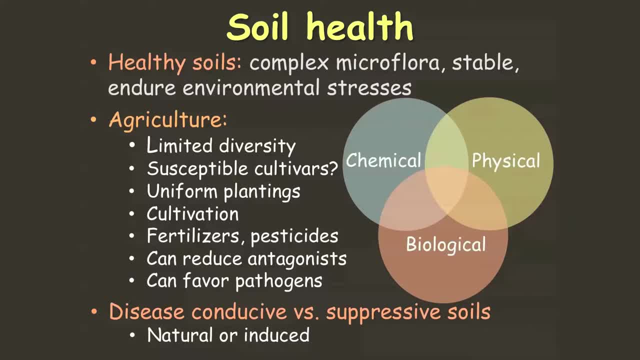 We have to do a conversion to totally suppressive soils. Suppressive soils are ones in which, even when you introduce the pathogen, the disease doesn't develop or doesn't develop very much, doesn't have much impact, And usually that suppression is very biological in nature. 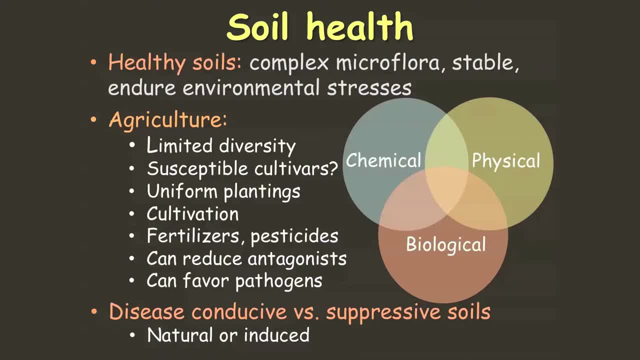 There's usually a very intense biological aspect that keeps that disease at bay and prevents it from causing severe losses, And so we'll talk about some of the methods we've looked at trying to shift a soil from being highly conducive towards being less conducive towards the spectrum of suppressive soils. 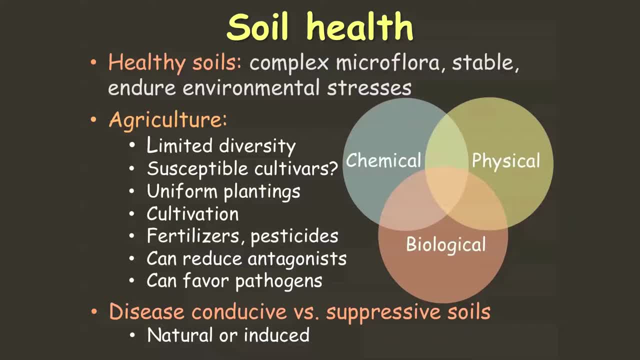 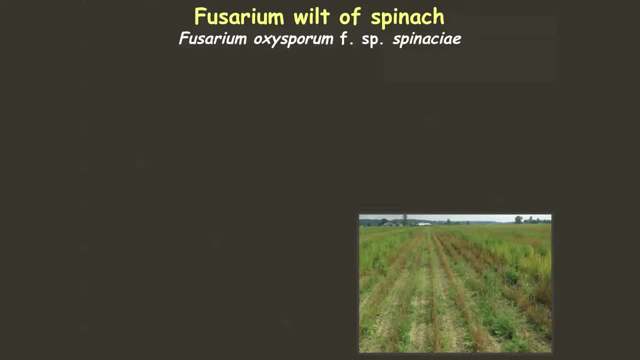 And these are illustrations of how, in agriculture, we can try to use that aspect of disease suppression in relation to soil health. I'm going to use an example and I apologize. I know most of you are from this side of the mountains. I do work both sides of the Cascades. 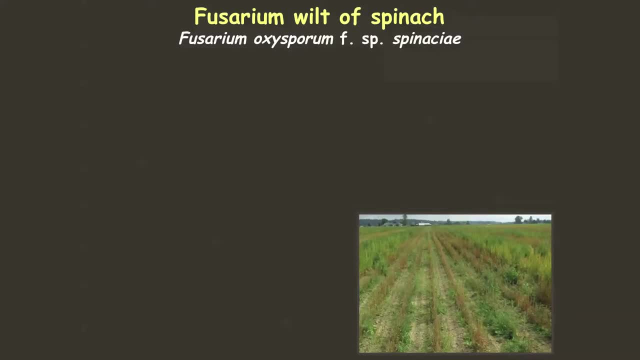 But it's a really good illustration of trying to work with a soil that's highly conducive and shifted towards something more suppressive, And hopefully the principles are relevant to you, But I work a lot in spinach seed production. Some of you may not be aware. 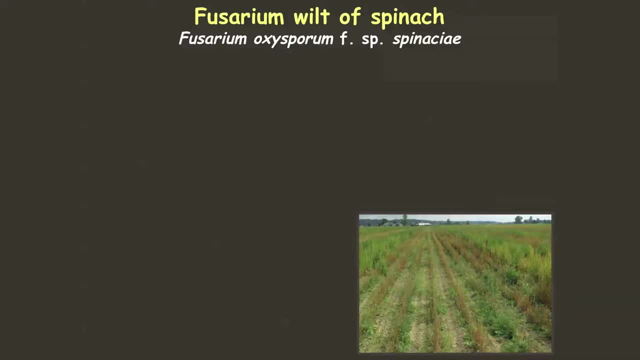 but western Washington and western Oregon are the only areas of the US you can grow spinach seed. because of their climatic requirements. You have to have long day lengths, cool summers and dry summers, And there's no other place in the US that has those combinations. 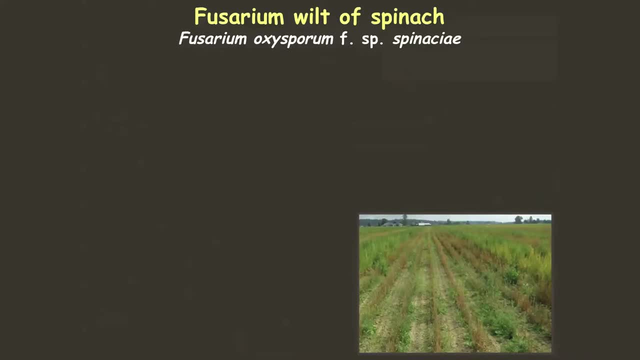 So those two areas are the only parts in the US we grow spinach seed And unfortunately, our soils are very acid on that side of the mountains because of the high rainfall, which makes them very, very conducive to fusarium wilt spinach fusarium wilt pathogens. 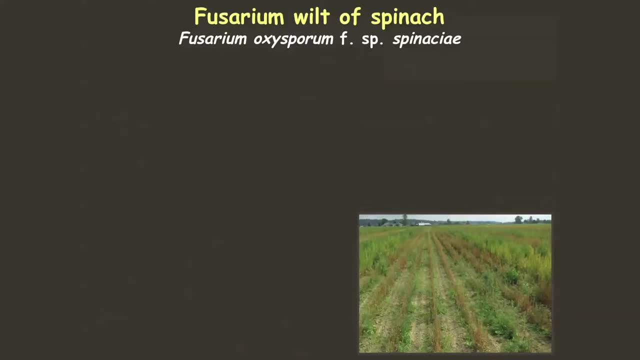 So, even though that is the only area of the US that you can grow significant amount of spinach seed on an economic, commercial scale, it's also very conducive to a disease that, as a result of this disease, spinach seed growers are on a 15-year rotation once they plant a spinach seed crop in a field. 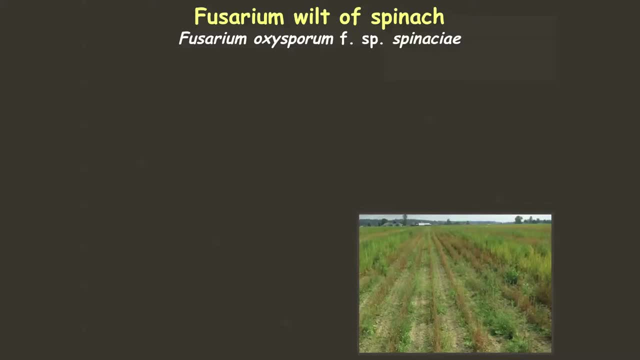 If they know they have really good partial resistance in the parent lines and that's all dependent on what contracts they get from the company- they can maybe get that down to 10 years. But that's still a long rotation period And our objective has been to try and help these growers shift that away from a 10- to 15-year rotation. 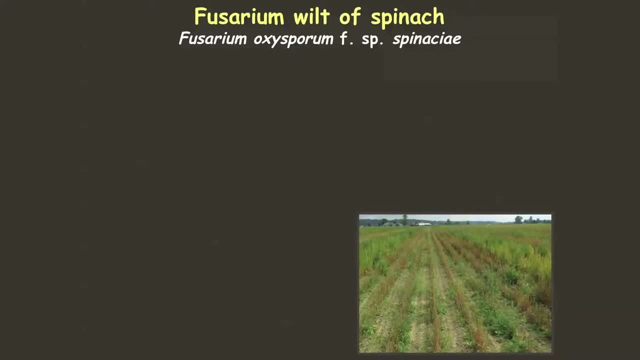 down to a 5- to 8-year rotation, which in essence doubles the capacity to produce spinach seed in the US. So that's been our goal in some of this research And I think we've come very close to achieving that by understanding what it is that makes our soils conducive. 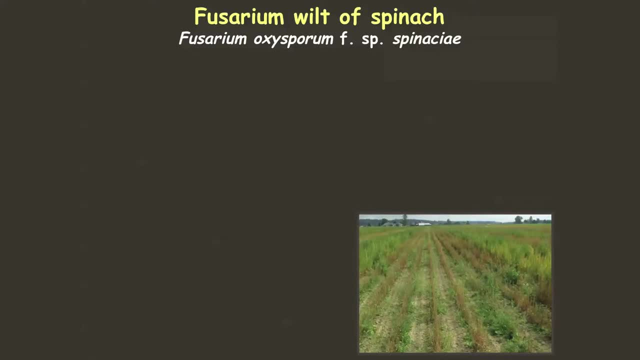 and what capacity we have to manipulate that soil towards a little less conducive, maybe even partially suppressive, And this is relevant to in the case in the Columbia Basin. almost all our soils are neutral or alkaline. by nature. It's a desert climate. 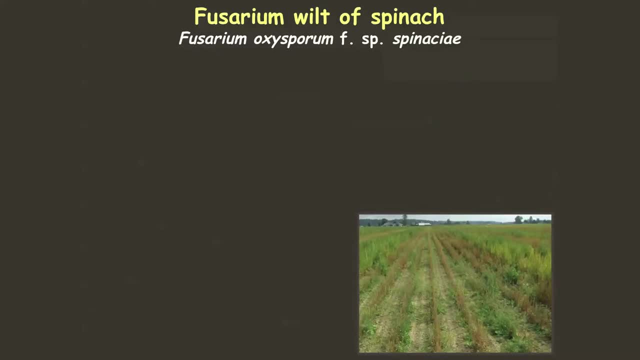 But there are parts of the Columbia Basin where 60-plus years of irrigated agriculture, with years and years of ammonium use, have shifted some soils towards acid, And I'll give you an illustration from the Columbia Basin. It's also a fusarium wilt. 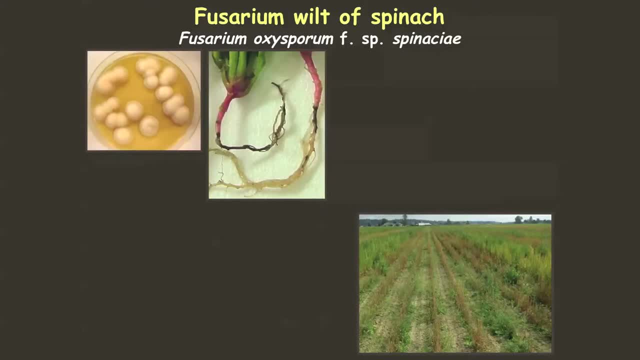 So this is a picture of the fungus growing in petri plates. It infects the roots, particularly young feeder roots, moves up into the vascular tissue. You can get wilts anywhere from young seedlings to mature plants. It turns the vascular tissue black. 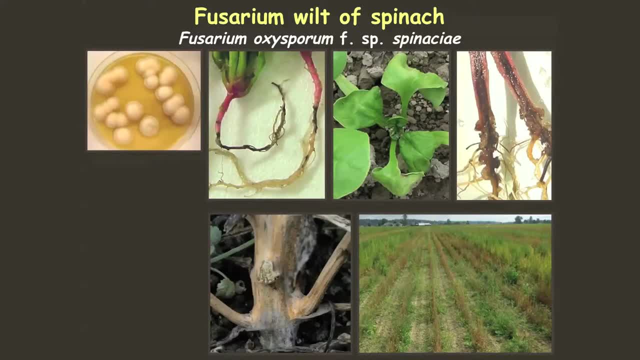 This picture in the bottom right-hand corner- sorry, find the marker. This is a hybrid seed crop. I'm not sure if you can see. all of the female rows are dead. Now in a hybrid production, if one of your parents dies, there's no crop. 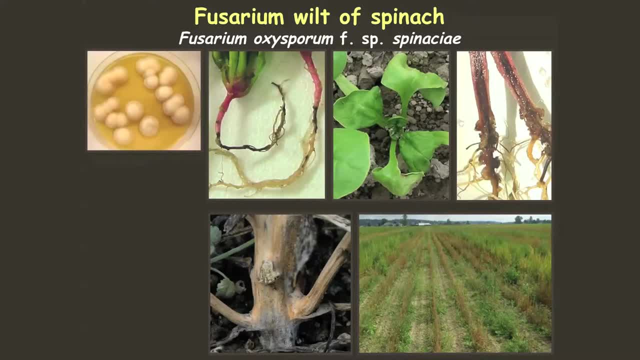 And this is what will happen if you go into a field when it's not when it's still in a has a high level of inoculum or disease pressure, And I've seen fields like this: 40-acre spinach seed crop hybrid. 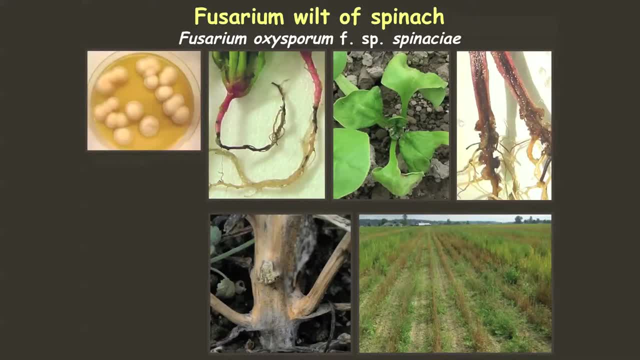 It had been out of spinach for 16 years and was completely wiped out by fusarium, And that's devastating Because it's a valuable crop both for the seed company and for the grower. So this is very intensely motivating to try and come up with a solution. 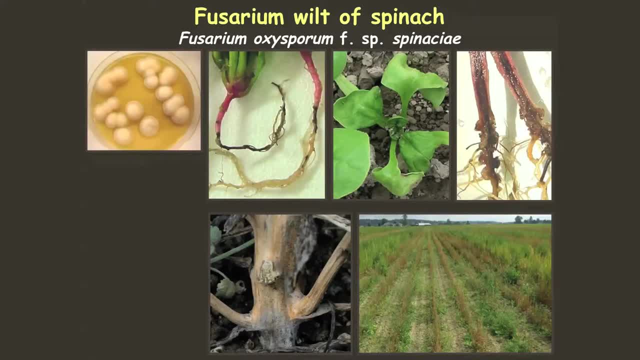 But when those plants die, I don't know if you can see in this picture- it's not very clear with the lighting, but there's an orange-salmon-colored appearance to the external stem. That stem is colonized extensively by fusarium. 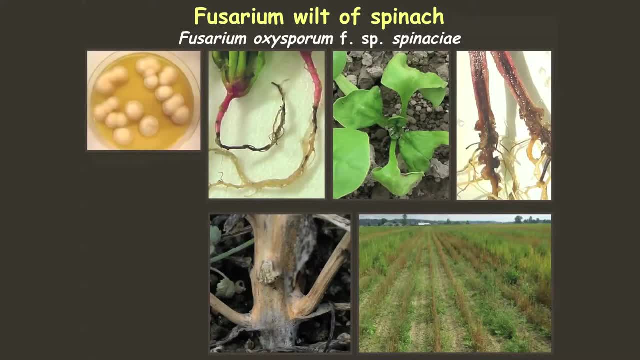 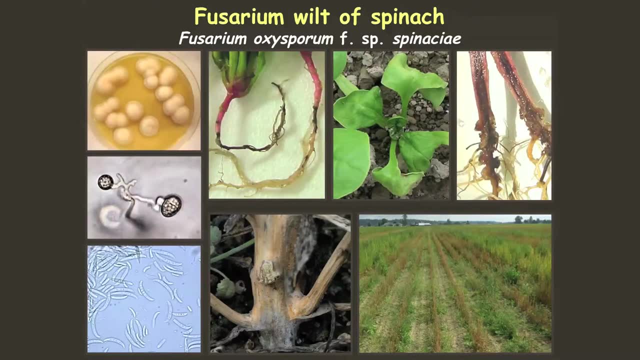 It's producing its inoculum on that dead tissue And you have to dry the plant out to get the seed, But unfortunately that favors the production of these spores and these. these are macrokinetic hair and chlamydospores. 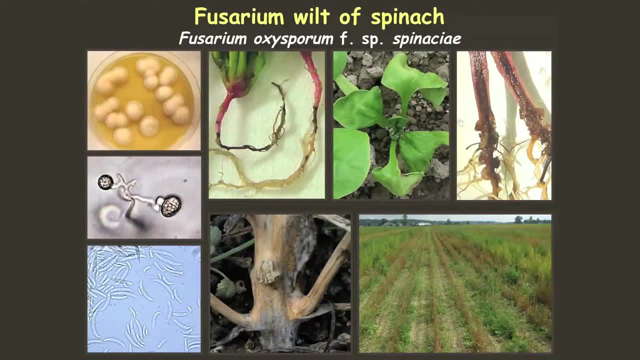 which are very, very persistent in soils. As I said, we've seen fields wiped out after 20 years And I've had a grower say: come and tell me, ask me to look at the field and say I would have planted across the road if I'd known this field was not ready yet. 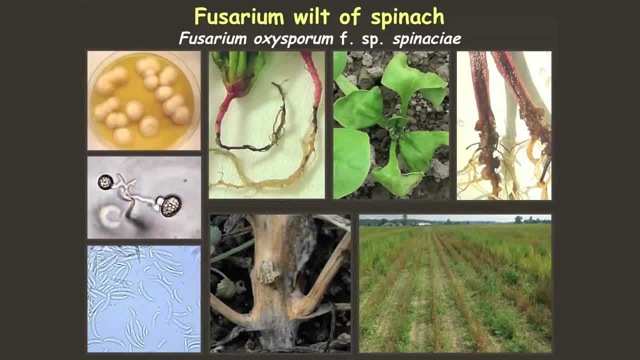 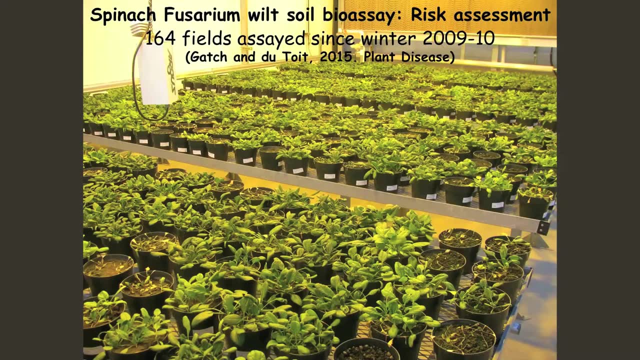 and 20 years should have been enough. Can you help us figure out how I can avoid these high-risk fields and look for the lower-risk fields? So, as part of a PhD student's project- she just graduated in 2013, and we part of her project- 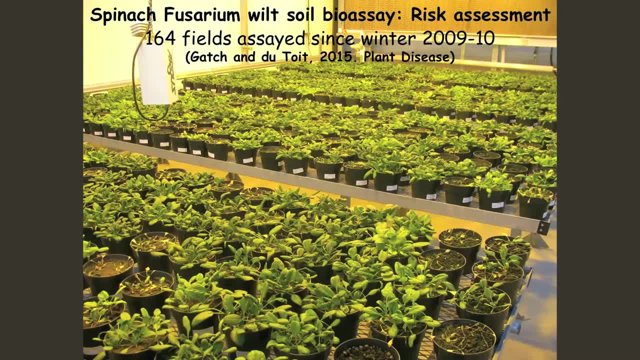 Part of her work will be published in Plant Disease next year if anyone would like a copy of this paper. But part of the subject was to try and develop a way of testing soils so growers could identify these really high-risk fields and not plant. 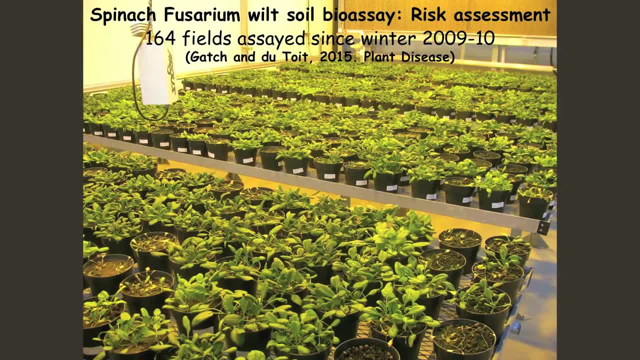 even though the rotation interval might say it's safe. So over the years we've tested about 164 fields from northwestern Washington that were going to be planted for spinach that spring. This is cumulatively now over five winters. We test them in winter because the growers get their contract in the winter. 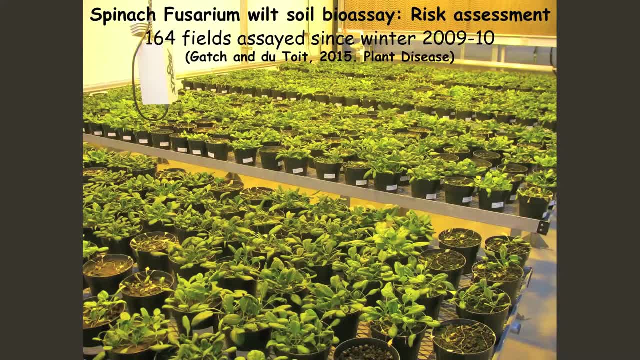 and they want to know by March 1st if the field is safe to go in or not, because March 1st is when they decide the isolation distances. because these are wind-pollinated crops And this is a picture of one of these years. 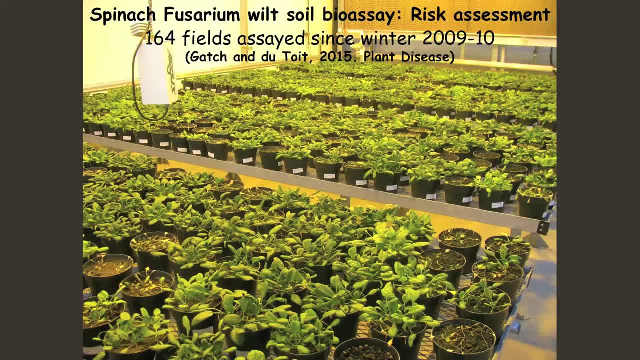 We had all the fields planted out. The growers bring us a five-gallon bucket of soil. They have to sample it randomly from their field. We plant it out in the greenhouse with parent lines that range from very, very susceptible to intermediate to partially resistant. 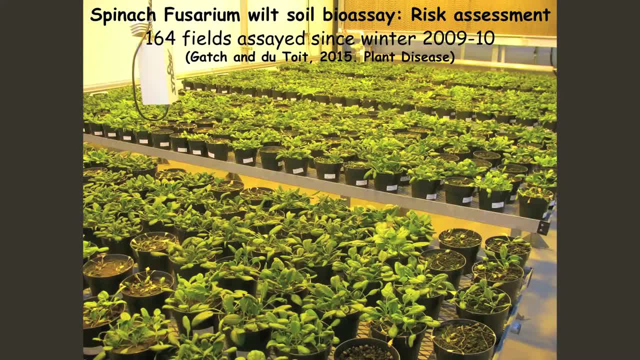 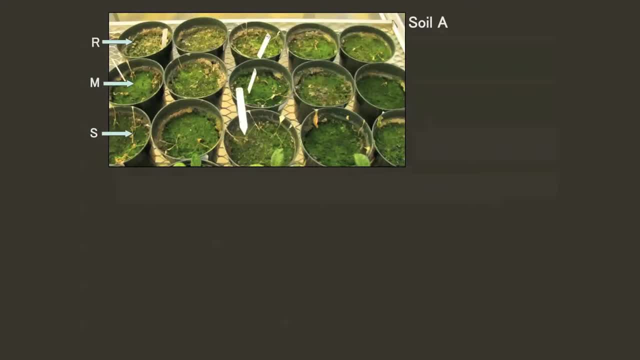 There's nothing immune, And they can come back after six weeks and take a look at the soil and see how the spinach is growing. This is an example of a field that clearly is high risk. This was 16 years out of spinach and nothing survived. 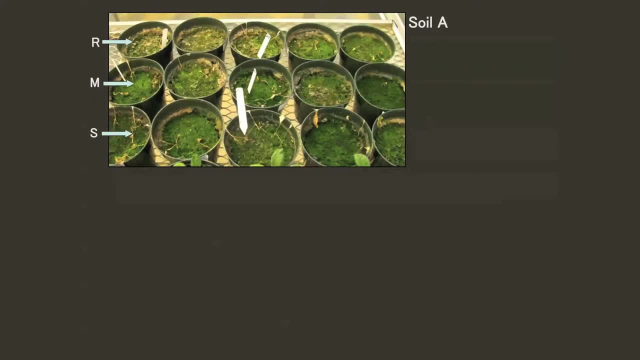 It doesn't matter how susceptible. There's a resistant female planted across the five reps. We unrandomized it to take these pictures at the end of the trial: the moderate female and the susceptible female. This is a field the grower was going to plant. 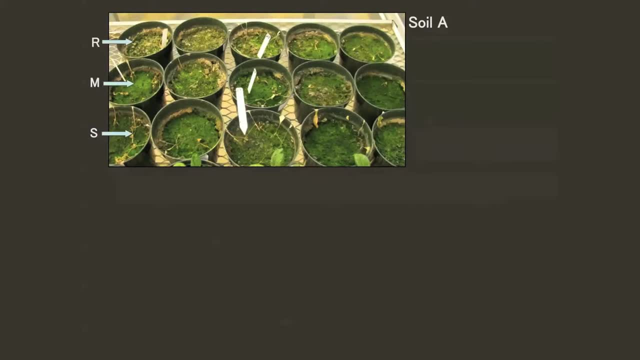 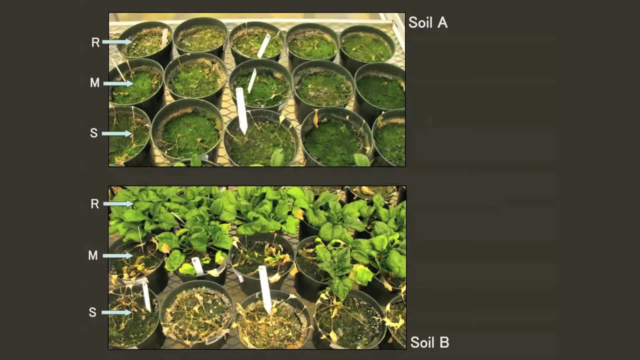 So it's turned out to be extremely useful bioassay. It's tedious, but it works. So this field, in contrast, is what we call an intermediate risk field, So the grower and the seed company that they might contract with. 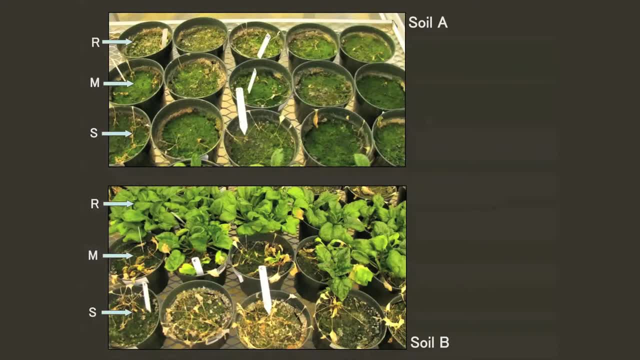 the rep will come to the greenhouse in late February and look at this and decide: okay, if the seed company understands the level of resistance of the parent line they're going to be contracting to that grower, they can assess whether this field might be safe to go to. 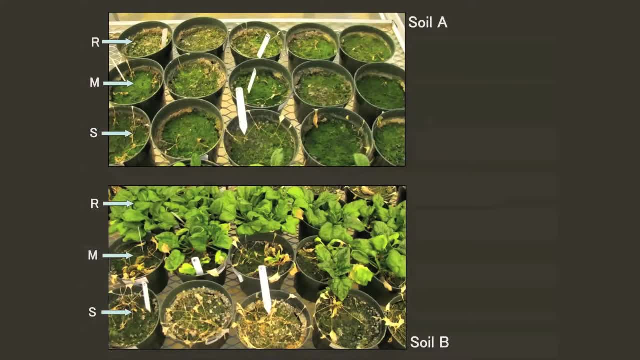 If it's a highly susceptible female, nothing's going to survive. If it's a moderate female, you're going to get some loss. If it's a resistant female, partially resistant, you might be safe to go back to that field, And then this is clearly a field that had no problems at all. 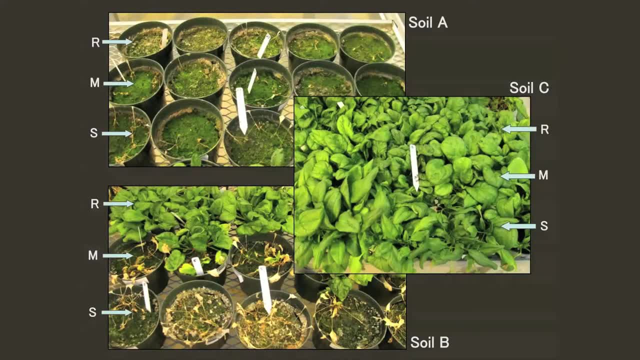 It didn't matter The susceptibility level of those parent lines. everything survived, everything looked good. That field was safe to go back to And it's surprising. The number of years alone is not adequate. Clearly it's important. If you're five years out, it's not going to be safe. 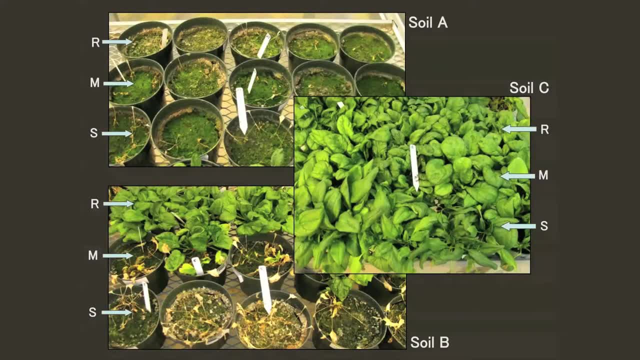 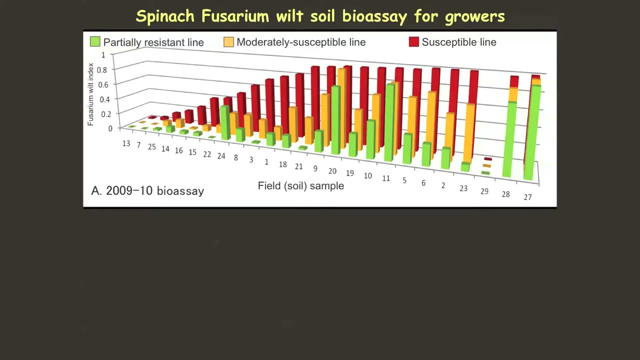 If you're ten years out. sometimes it is and sometimes it's not. So as we've tested these soils over the years, we've developed this database. This is an illustration from one year, 2009 to 2010.. You have the fields coded. 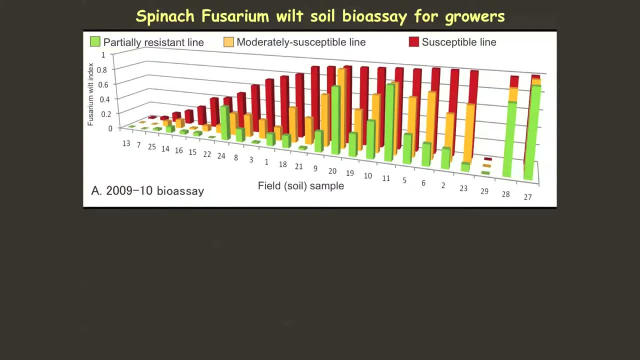 so growers don't know whose is what? organized in terms of least amount of risk to highest risk. The height of the bar represents the amount of disease we recorded. The green bars are for the partially resistant female line. The orange bars are for the moderately susceptible. 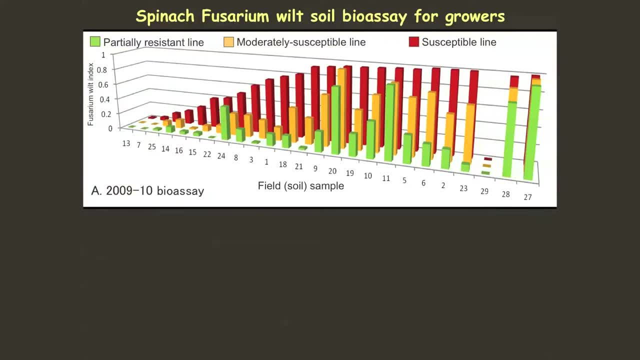 and the red bars are for the highly susceptible And, as I said, every one of these fields was being considered for planting that year. So you can see there's a lot of very high-risk fields. There's only a few that had no risk whatsoever. 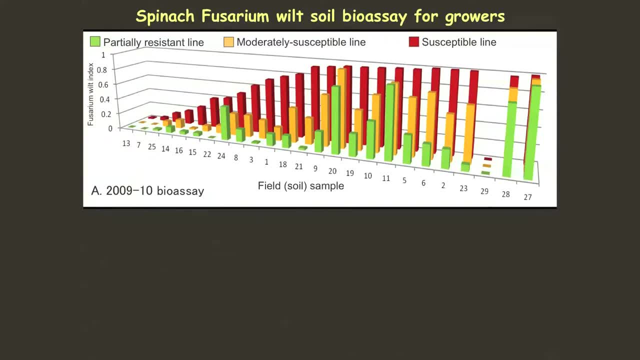 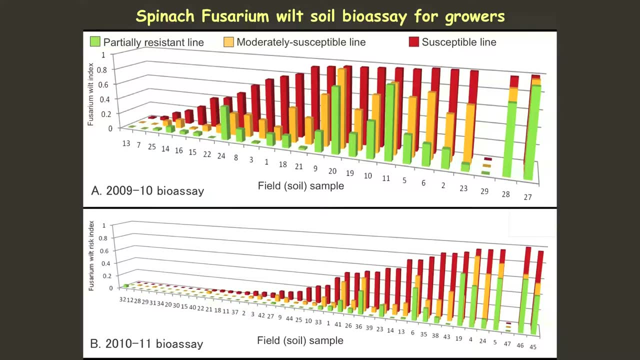 And these are our control soils on the end that we used to try and make sure we're testing under the right conditions. And this is another year just to illustrate. This was our first year of testing and, based on the success, you can see how many soils were submitted the next year. 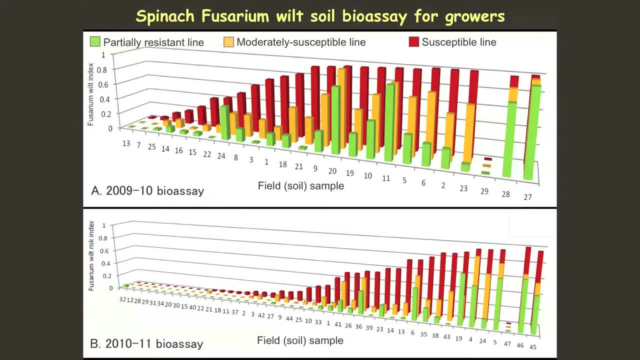 because they realized $150 for this test is cheap insurance for a quarter-million-dollar crop And you can see there were a lot of fields that were pretty safe that year that were submitted but we still had some very high-risk fields. What we try to do is look at all of the chemical and physical properties. 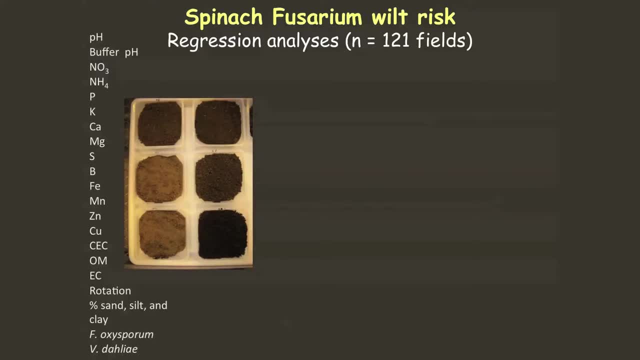 of these soils that we measured, every sample we tested. We also measured the amount of fusarium in the soil, measured the amount of verticillium, which is another world pathogen that can go to spinach, And we try to come up with. 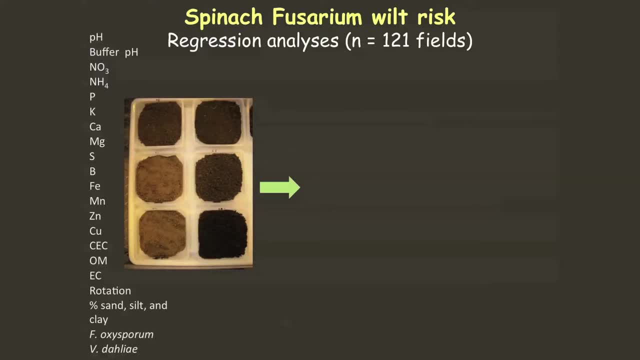 try to find out if we could use the existing physical and chemical properties of the soil to predict risk, as opposed to doing an eight-week bioassay, which is a lot of work. It would be a lot simpler if we could do that. The strongest relationships we could come up with. 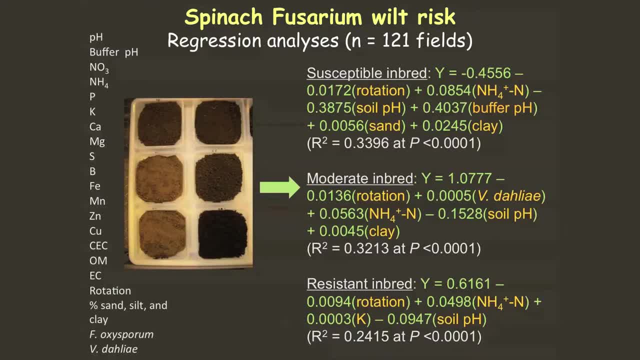 this is the susceptible, moderate and partially resistant female lines that we use And we looked at a regression relationship to see which of these variables most strongly predicted the level of risk. And you can see just if you look at this thing called an R squared. 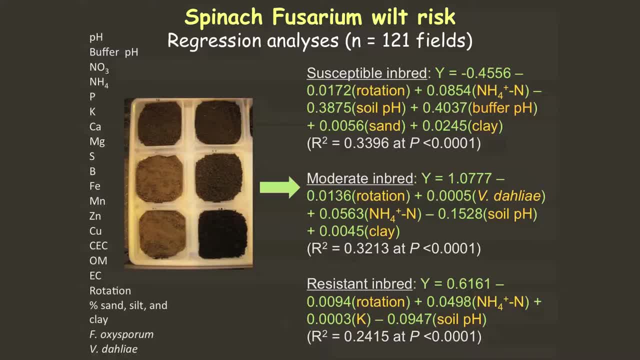 it's .3396, which tells you 34% of the variation in wilt could be accounted for. We're not even 50% accountable. With all those variables we measured, we still couldn't account for more than 34% of variation. 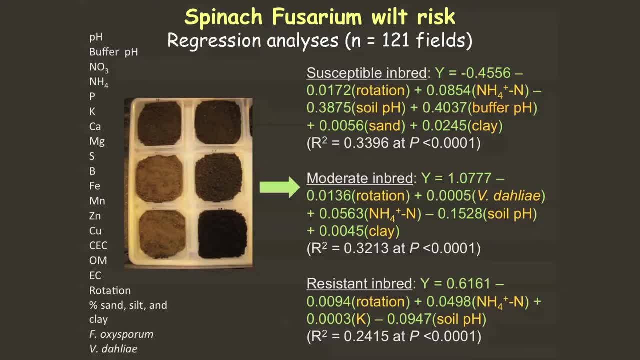 in the wilt. that was measured, which shows you we can't just rely on the chemical properties alone to predict risk And therefore we've continued to offer the bioassay. In fact, growers are bringing soils to our lab this month to get the bioassay set up in early January. 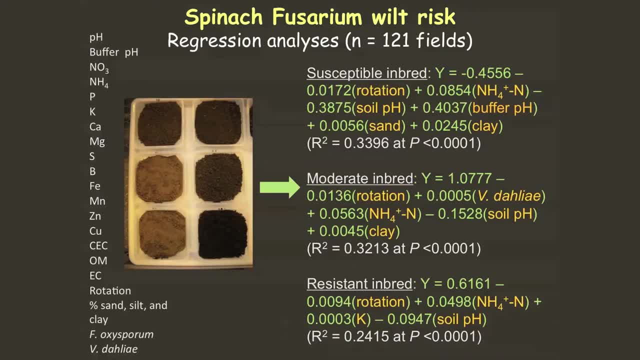 so they have the results by March 1st. And with the moderate parent, the strongest prediction we could get was 32% and the resistant was 24%, And you can see variables that seem to be most important, and all three was the number of years out of spinach. 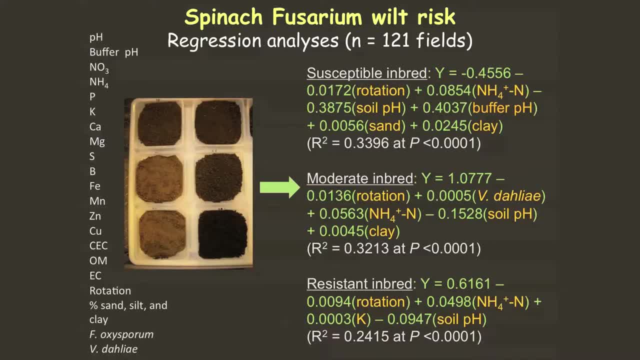 It's still an important predictor, but it's only making up a portion of that. 34% Ammonium levels. Physerum is promoted by acid conditions. Ammonium means high acidity, Hydrogen ions, high acid, Soil, pH, which is obviously all related. 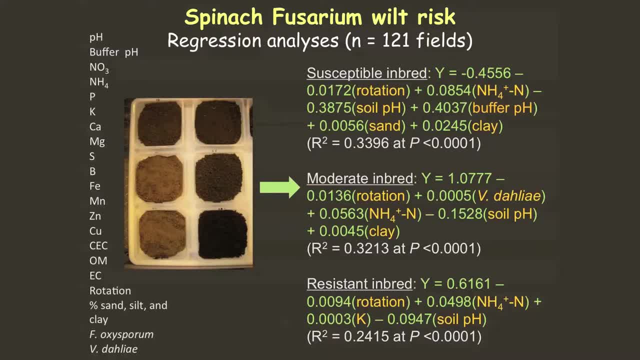 Buffer, pH And percent sand and clave. in the case of the susceptible And the moderate parent it varied a little bit. The incidence of verticillium came in because this parent happens to be susceptible to verticillium And that wilt kind of confounds the physerum ratings. 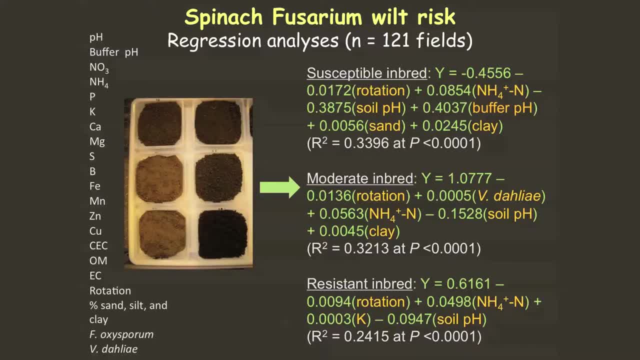 although we know we're not measuring verticillium because in spinach the disease doesn't develop. verticillium doesn't develop until after you initiate bolting flowering And we don't carry this through to flowering, We do it in the winter so it doesn't flower. 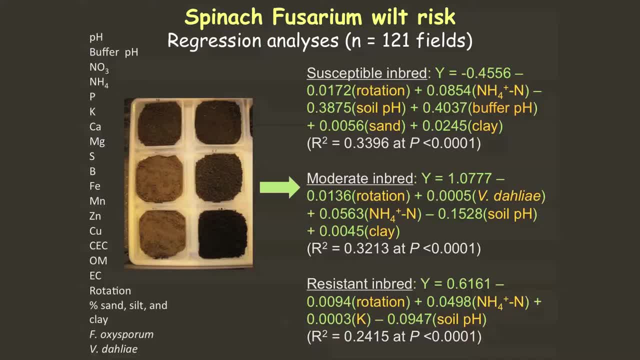 And we're only measuring physerum, not verticillium. In the case of the resistant, ammonium and potassium and soil pH were very important in addition to rotation, But even with all these variables we couldn't account for more than 34% of the variation. 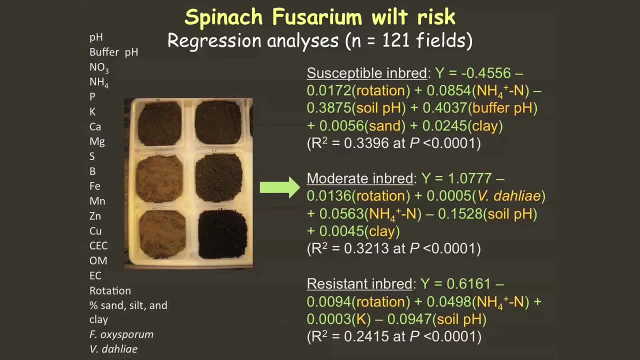 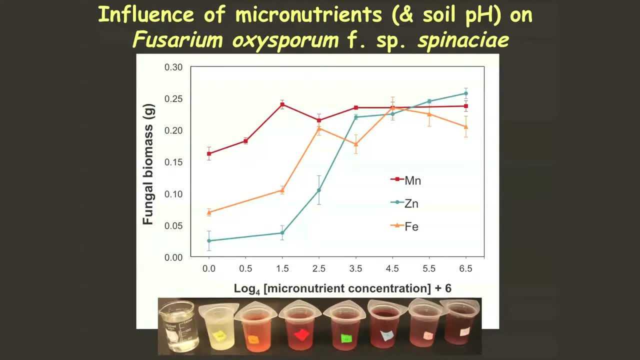 So we're going back to the old-fashioned way of testing soil as a bioassay, And it's been pretty effective. What is interesting is, as we monitored this as part of the PhD Students Project, is trying to figure out what is changing. 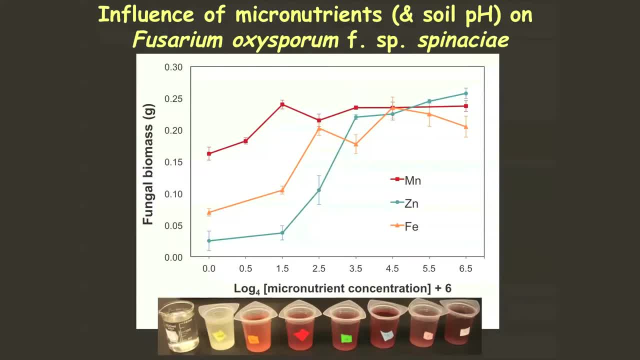 when we go from a conducive to a less conducive soil, what ends up changing? We know that as the soil pH rises, physerum wilt, tends to get less severe. It doesn't go away, but it gets less severe, And one of the things that happens as you raise soil pH. 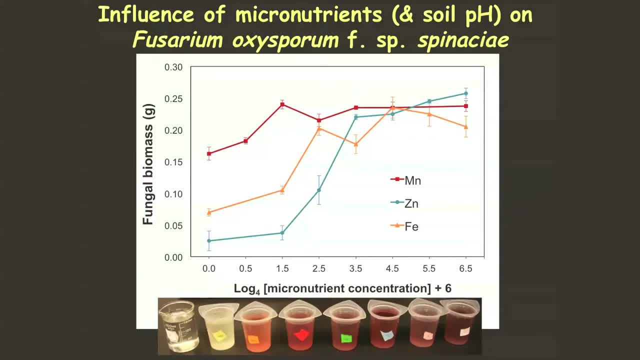 over the range that we might encounter is that manganese, zinc and iron change in availability. They become less available as you raise the pH And you can see this is the growth of the spinach physerum wilt fungus on the y-axis versus the concentration of these micronutrients. 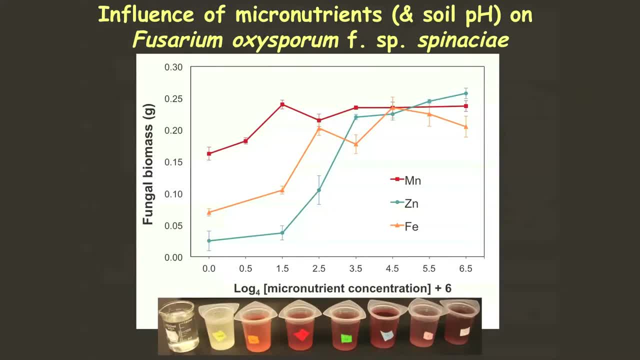 And you can see how rapidly the amount of growth that fungus increases as we increase the availability of these micronutrients And we've shown this repeatedly And it makes sense. We've monitored trials where we've put limestone out at different rates and we see this change in micronutrient availability. 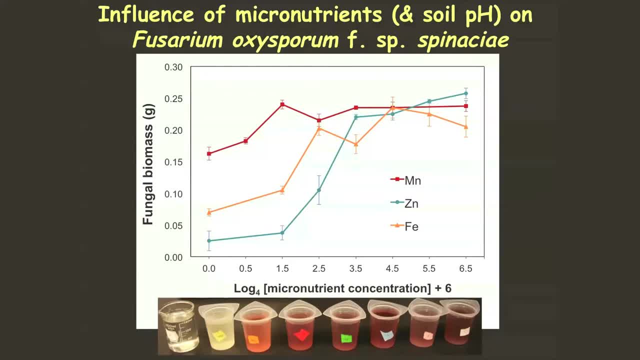 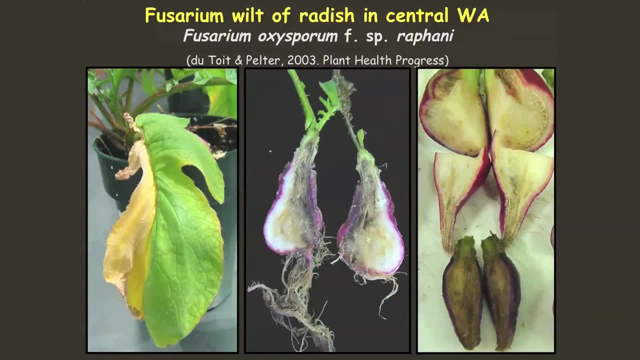 And these seem to be some of the driving factors behind the change from highly conducive to less conducive as we add things like limestone to soil. I wanted to bring this back to a crop that's maybe relevant on a small scale to the Columbia Basin. But in 2002, Gary Pelter, before he retired, 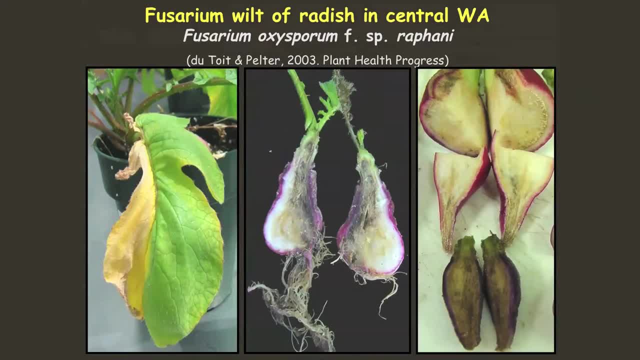 and I were asked to look at a radish seed crop that was just falling apart and happened to be physerum wilt, And we took some soil samples and the pH was 5.8.. This is in the Columbia Basin up towards the Quincy area. 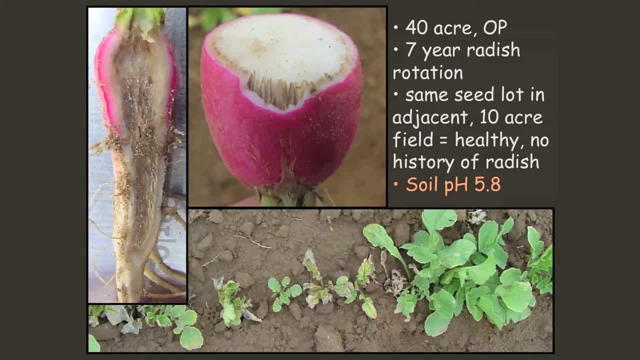 In 2008,. I was asked to look at another radish seed field- This is a picture taken in there- Completely wiped out by physerum. They disked the field out and they came back and planted beans- pH 5.8.. And it had a radish seed crop. 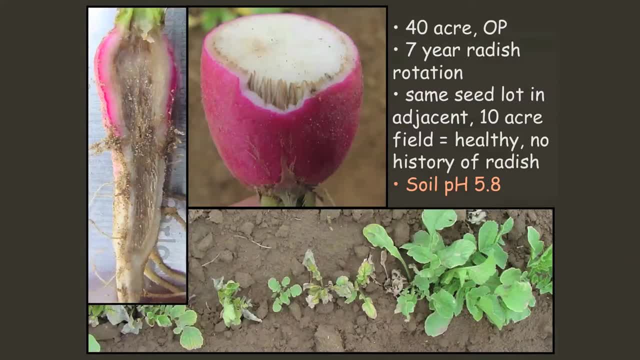 seven years prior, So we're talking about a seven-year rotation, acting exactly the same way we saw with physerum wilt on spinach on the west side. So, as soils in this area shift, as a result of long-term agriculture and ammonium use, towards 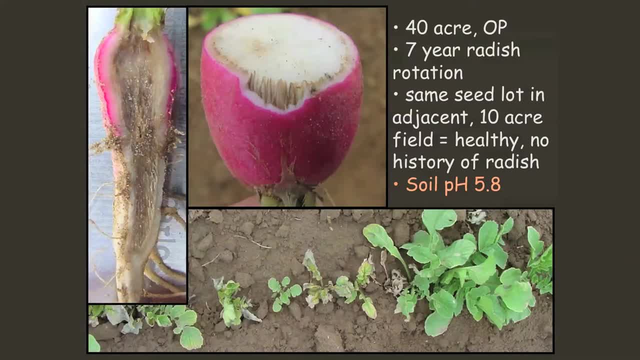 this kind of acid situation, we see a shift in which diseases become a problem, So now these soils are becoming conducive to these conditions. You normally don't see these diseases In Denmark, which is the biggest area of spinach seed production in the world. 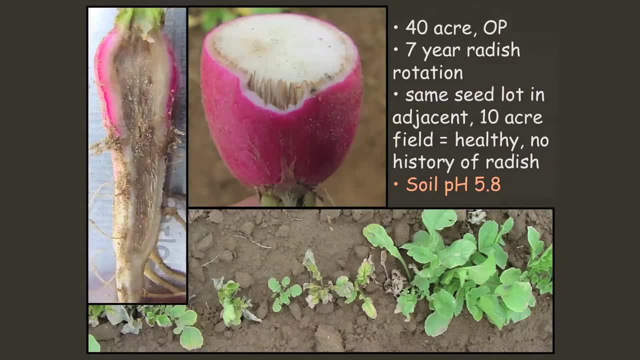 it has those unique climatic conditions that we have in western Washington. they can grow spinach on a five-year rotation and they don't see physerum wilt. Their pH is in the high sevens- low eights because they have extensive limestone deposits. 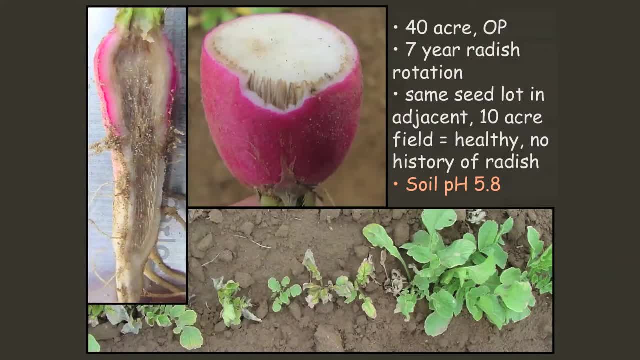 beneath the soil. So they have high calcium levels and high pH which is very suppressive to physerum wilt, naturally suppressive. So we're trying to see if we can shift our soils a little bit towards neutral, Get away from naturally reverting to acid. 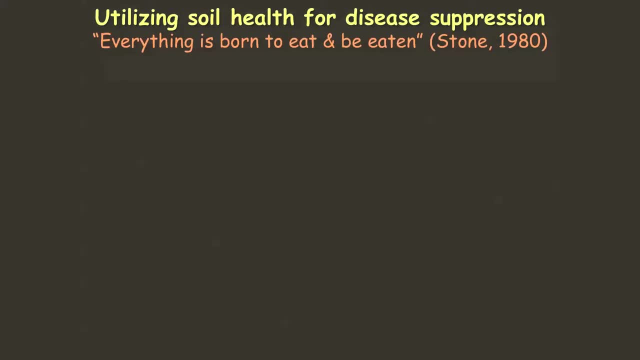 because of all the rain. Okay, and just how to utilize these understandings of soil health to look at disease suppression and enhance our ability to suppress some of these diseases? I like this quote from Stone in 1980.. Everything is born to eat or be eaten. 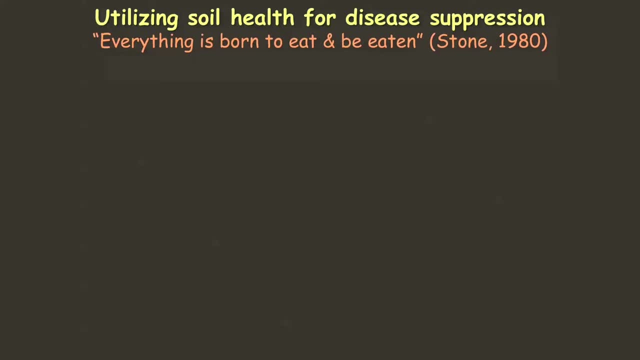 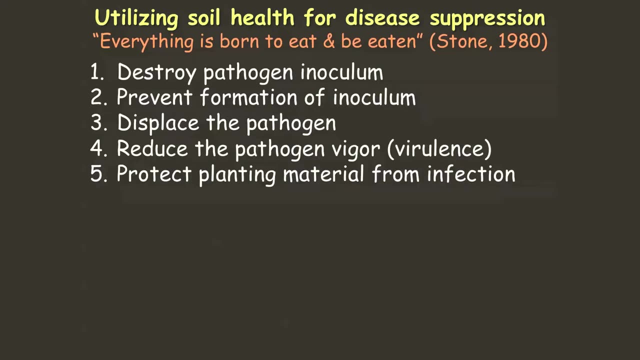 and be eaten. And this applies too in the soil environment with this complex interaction of microbes. And there's five principles of using soil health to suppress diseases. One is: you use soil health to destroy the pathogen inoculum and we'll go through. 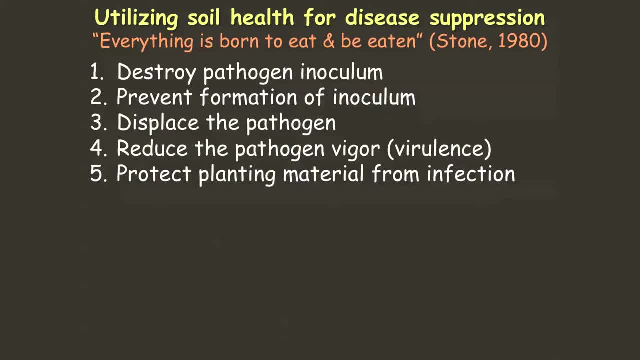 some examples: Or to prevent formation of inoculum, Or to displace the pathogen. if it is there, so it doesn't colonize the roots Or reduce the vigor of the pathogens. The pathogen is there, but it is less able to cause disease. 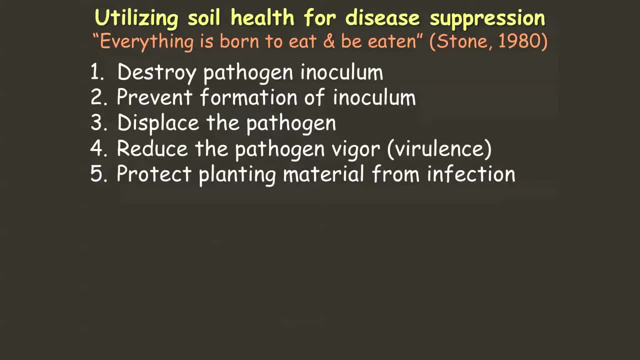 And we know that, for example, in spinach and physerum wilt, as you decrease the availability of these micronutrients, the pathogen is still there, but it's less virulent, less able to cause as much disease, And we've shown that. 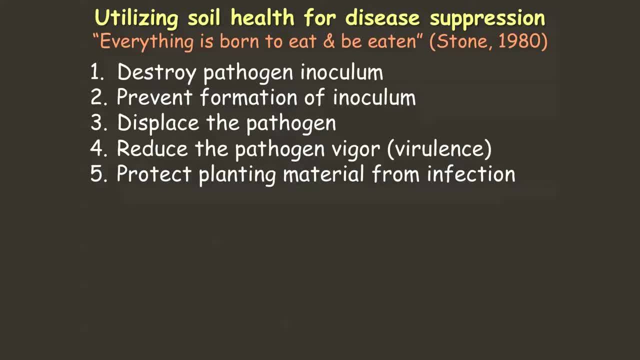 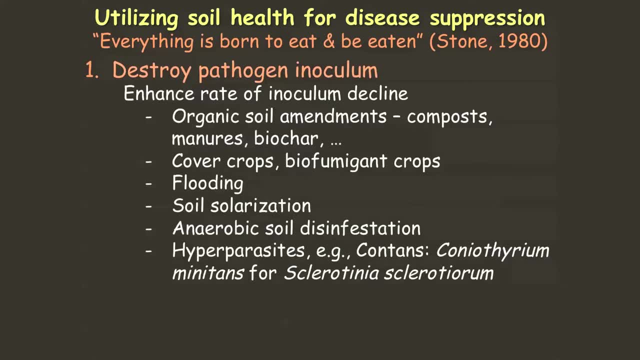 as part of Emily's PhD project, And then protecting your material from infection if you know you're planting into infected soil. So let's go through a few examples of these. The first is destroying pathogen inoculum In soils, even with pathogens that tend to sit around for a while. 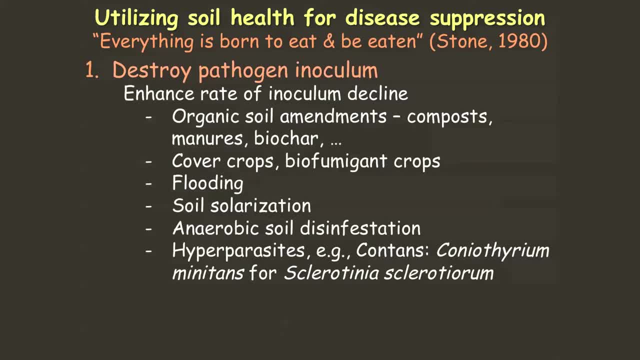 in the soil. that inoculum does tend to decay over time, decline over time. Some of them will grow much faster than others. Things like verticillium will persist in sclerotinia longer than for fungi that don't, for example, have. 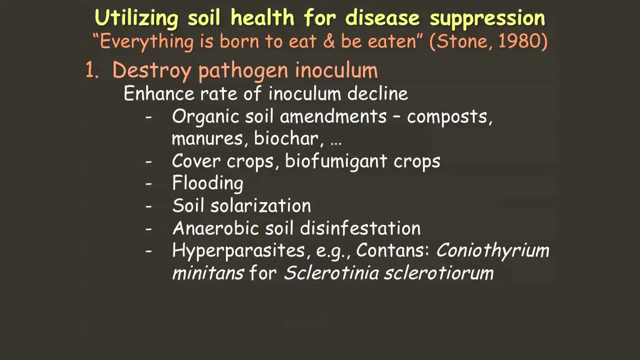 really hardy, dormant resting structures. Ways that you can enhance that rate of inoculum decline focused on soil health include many of these organic soil amendments that Dave and Andy mentioned during the survey earlier, such as the compost amendments, manures and biochar. 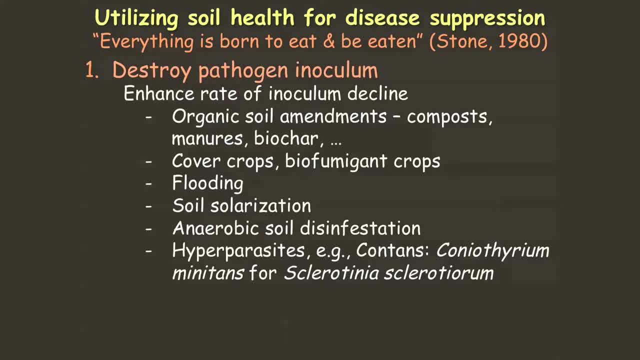 Those amendments are stimulating microbes in the soil that naturally will colonize those dormant structures of the pathogens, start to feed them and break them down. Same thing with cover crops and biofumicant crops. A lot of these are basically ways of promoting 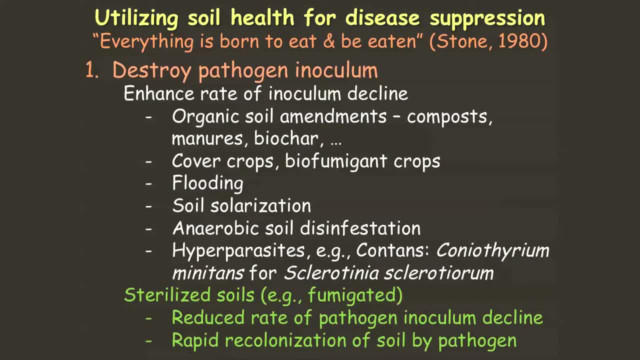 a shift in the microflora in the soil to antagonize those dormant structures. Flooding has been shown in some cases to help decay. I had a meeting at 9.45 yesterday. I need to change my watch. Soil solarization which? 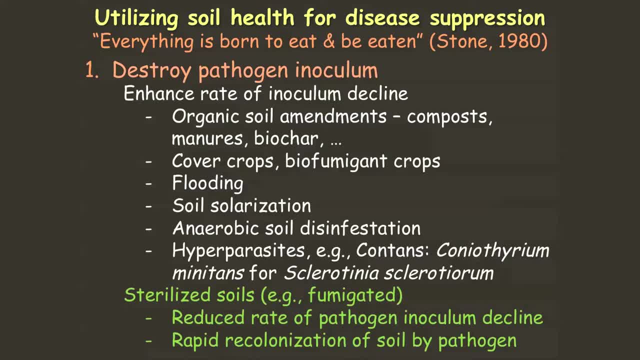 tends not to work as well in our environment. even though we have hot summers, it's not a long enough period. but places like California and Israel that flooding and solarization can be used very effectively. Anaerobic soil disinfestation is a new. 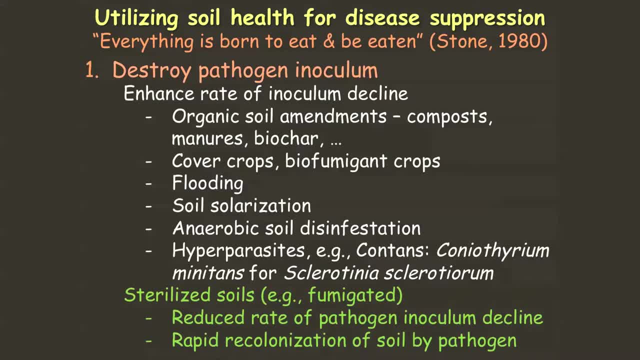 method that's being checked out fairly carefully for places where you can flood and keep the soil- the wet saturated soil- covered so it turns anaerobic Again. you're shifting the microflora towards microbes that survive well in anaerobic conditions and most 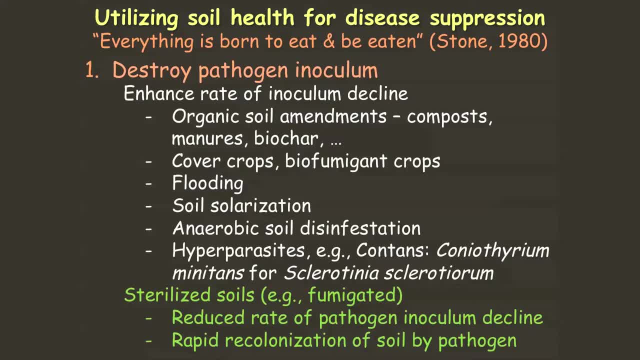 plant pathogens. don't You get more antagonists building up? You also get products that are hyperparasites, microbes that feed on other microbes. A good example that is used widely in the Columbia Basin is the fungicide contans, which contains. 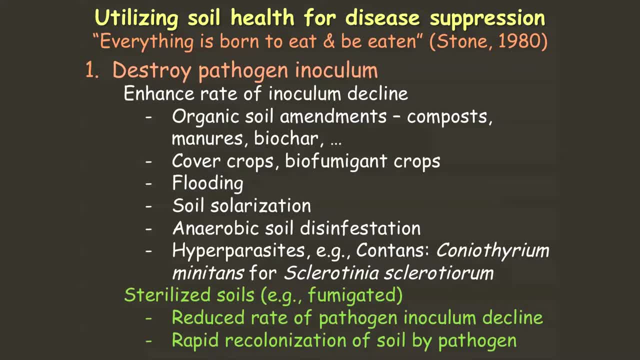 the fungus coniothera minotans- hence the name contans- and it's a fungus that feeds on the white mold sclerotia. You're all familiar with the sclerotinia fungus that produces white mold sclerotia, little rat-toad-like structures in the soil. 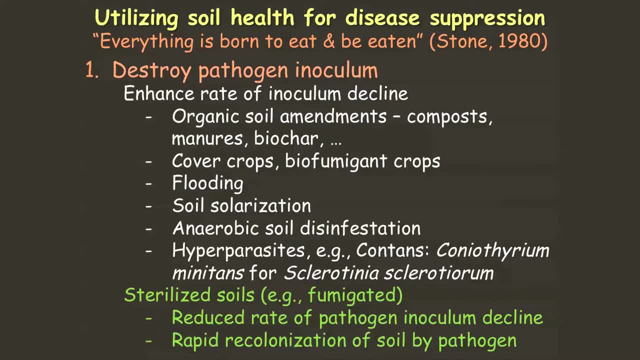 It affects potatoes, peas, beans, sunflower, you name it. It goes to a lot of crops. Contans will feed on those sclerotia and it's being used fairly widely in the Columbia Basin to help reduce inoculum levels in fields when you have had a white 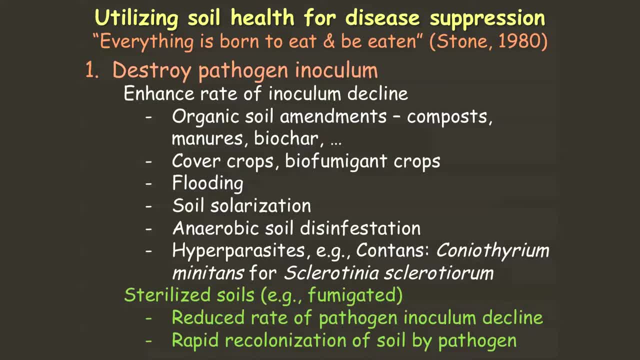 mold outbreak. I put in green here two very important things that we have to deal with. in agriculture, particularly in the Columbia Basin, There is widespread use of soil fumigation. This has potentially a very adverse effect on building soil health. It's a reality we have to deal with. 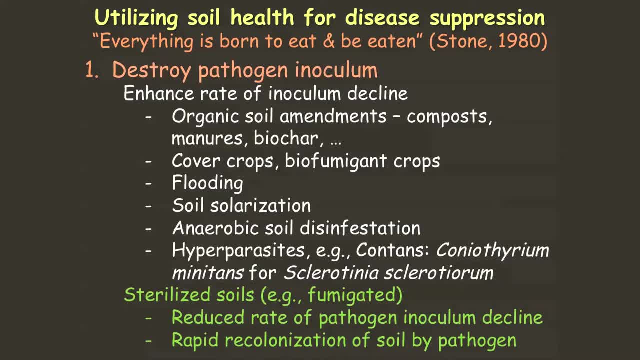 and it's part of the reason we've taken on certain projects in my program- is to help growers look at where they are using fumigation. are there ways you can help rebuild soils because fumigation will reduce the rate of pathogen inoculum decline. Some fumigants will. 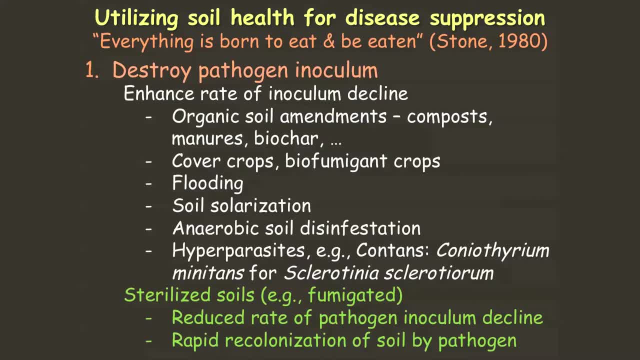 kill a pathogen, but you're not killing the pathogen throughout the soil profile. You might be killing it at the top 10 inches or a foot, whatever your depth of fumigation is, depending on the product, but you still typically have a low. 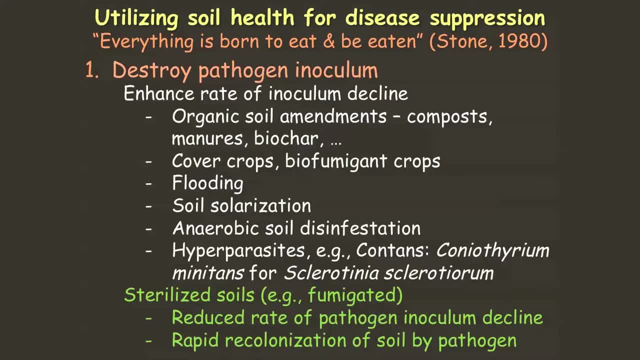 level of inoculum left. What can be worse? fumigation can exacerbate soil borne diseases because you've killed out the beneficials as well as the pathogens. You can get very rapid recolonization of that sterilized soil by pathogens if you aren't careful about. reintroducing beneficial microflora. I've seen this happen before where it resulted in a worse situation. Some of the crops, like potatoes and onions- there's fairly regular fumigation Which tends to prevent that, but it's at a cost when you start. 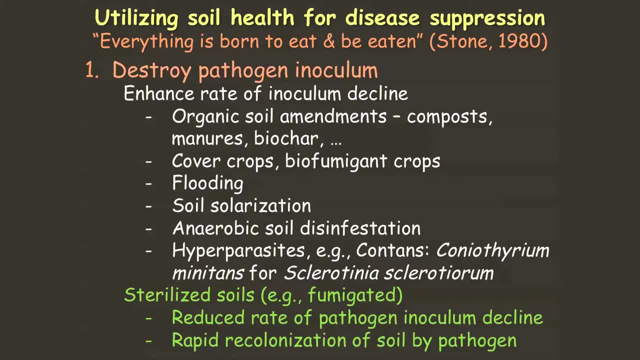 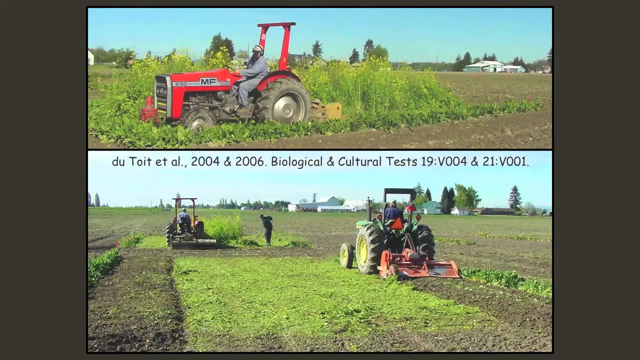 to repeatedly destroy the beneficials in your soil as well as the bad guys. Andy, this is just a picture from one of our trials, but Andy McGuire has done a lot of work on mustard by fumigant cover. crop type of situations. 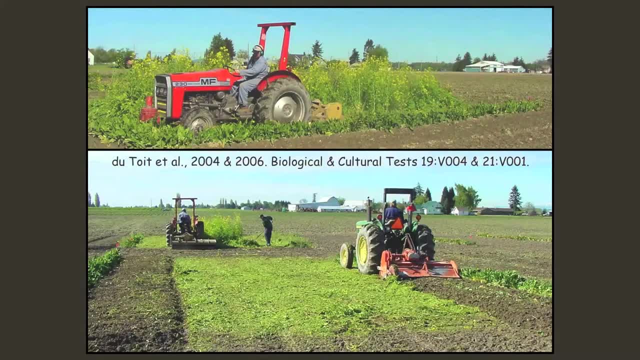 We tested this to try and control on spinach seed production on the west side. It definitely does help and can make a big difference. I've been told, Andy- I'm not sure of the latest statistics- but at least 20,000 acres of mustard cover crops. 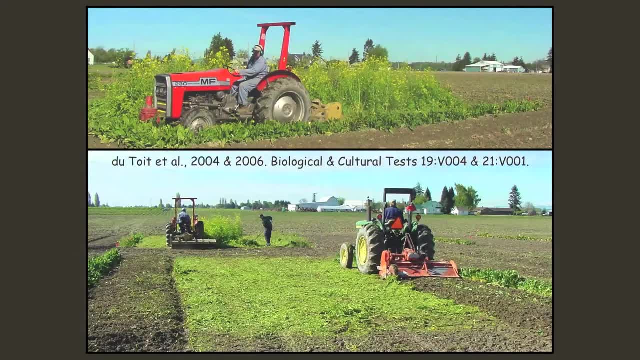 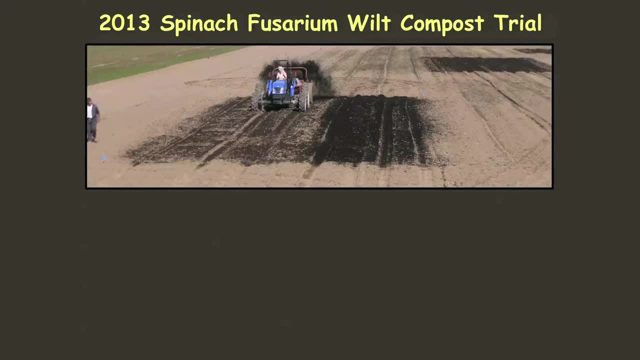 in the basin annually, So it's certainly playing a role in soil health development. We've also done quite a bit of work looking at composts to see if we can improve, enhance the suppression of fusarium oil to some degree using this kind of biological 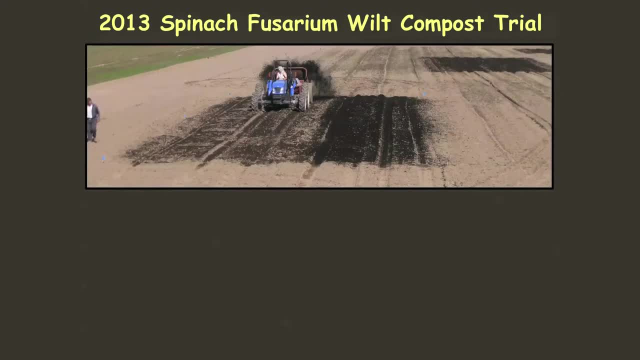 amendment. We have one of the town of Lacona in the Skagit Valley donated biosolids compost that they produce as a waste product And these seed crops are non-food, non-feed, So there's no issue with GAP. there's no issue. 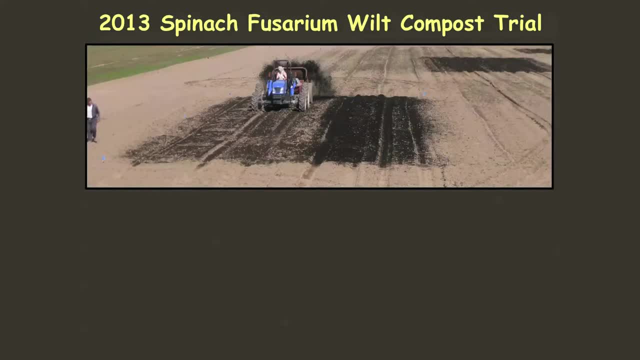 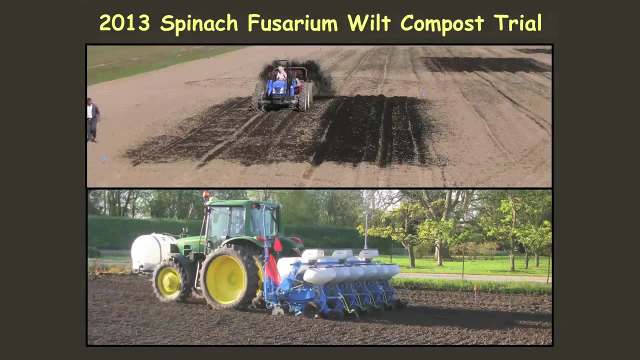 with food safety because you only harvest the seed. It's a non-food, non-feed crop. So we figured it's a product that's available in the valley, let's see if it works. And we planted a spinach seed crop after putting on about 20 tons per acre of 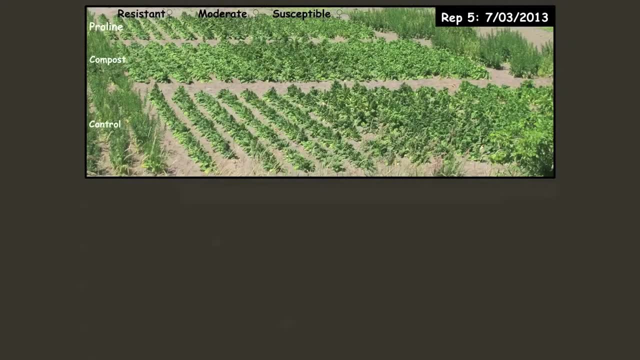 limestone in these very large replicated plots. This is a picture, a snapshot picture in early July of the field. I'm not sure if you can see, but across the six rows of the resistant female running all the way down the same resistant, moderate and susceptible. 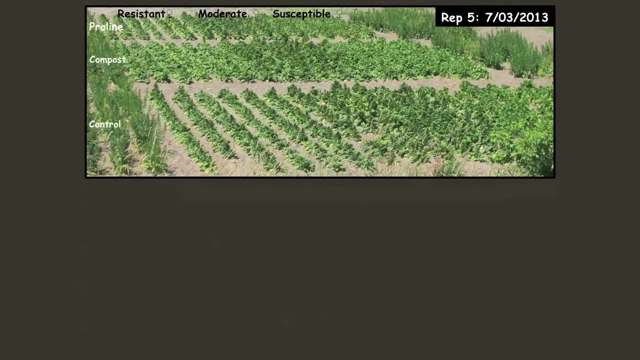 we use in the bioassay. Here's the six rows of the moderate and the susceptible. This is the control going across left to right in the front, the compost treated plot in the middle and a fungicide we were looking at in the back. 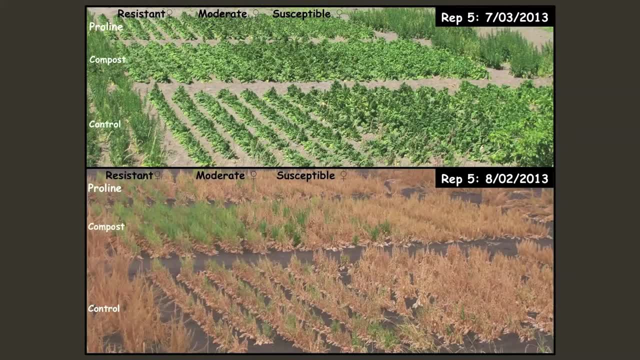 This is one rep of the trial And a month later, when you look at this plot and everything's senescing because you're letting the seed mature, you can see where those compost treated plots are. It was pretty distinct: A single application, six days. 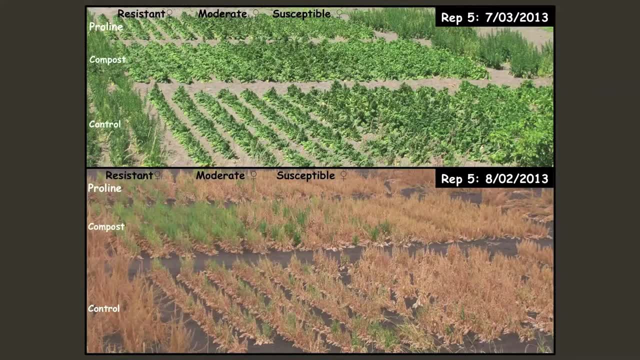 before planting. And this is a pretty heavy soil. Soils on the west side can range from a couple percent to seven, eight percent organic matter, depending where you are in the valley. So this was a fairly clayey soil And when we look at what it did to the disease, 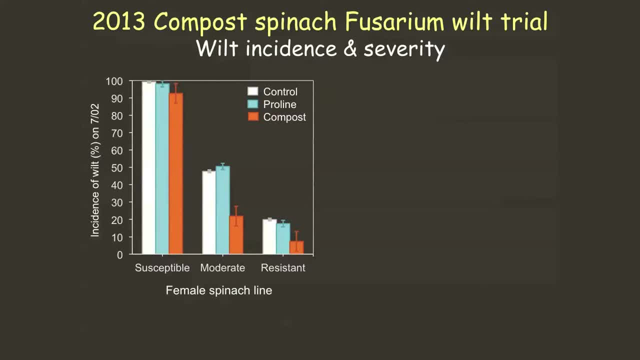 this is incidence of wilt in early July for the three females. the white bars are the control and the orange bars are the compost treated plots. It doesn't look like a huge drop in incidence of wilt on the susceptible female because it was so susceptible. there's so much disease. 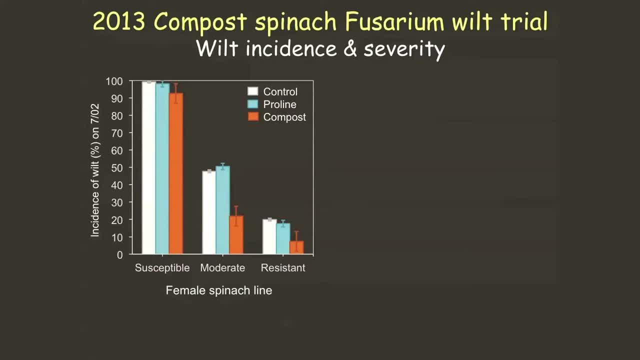 This is a six year rotation, You expect that amount of disease, But it dropped the amount of wilt on the moderate and resistant females by about 50 percent, which is very significant, And when we look at severity of wilt. so this is just whether 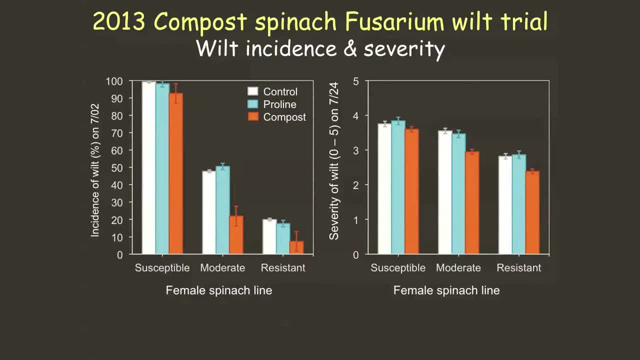 the plants wilted or not. that's incidence. Severity is how badly were they wilting? You can see by early July- sorry, July 24th, which is pretty late for this trial. compost was lowering the severity of wilt. It was much more significant earlier in the year. 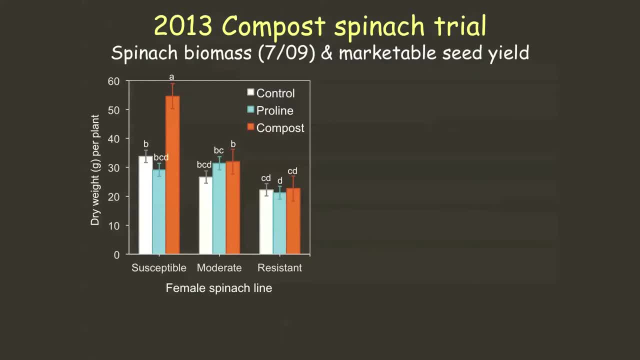 When we look at growth of the spinach, despite the fact that it didn't seem to reduce incidence. look at the growth of the spinach susceptible line in the presence of compost. We increased their growth by 50 percent. And then when we looked at seed yield, this is marketable seed. 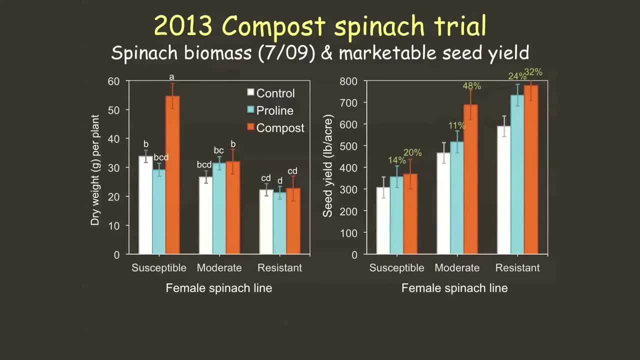 yield harvested from these plots. We got an increase in seed yield that ranged from the susceptible female of 20 percent- sorry for the susceptible- 48 percent for the moderate and 32 percent compared to the control plots, which is pretty significant for a seed grower. 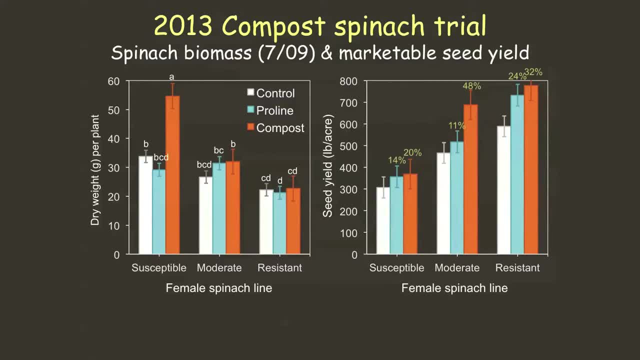 when you're paid on the seed. So we're pretty encouraged with this. We've done more trials both in table beet seed production and in spinach seed production, because we do have big issues with soil health problems. on the west side You think we have good soils because we have high organic. 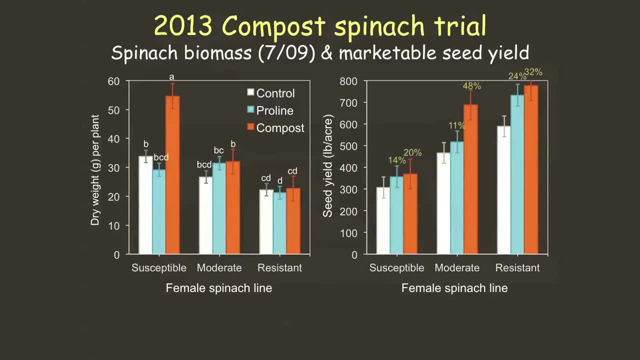 matter, but that's not an indicator of soil health alone. We have a lot of compaction. We have 15,000 acres of fresh market potatoes. They're often getting dug after the rains have started. We had about eight inches of rain in one month in October, right when 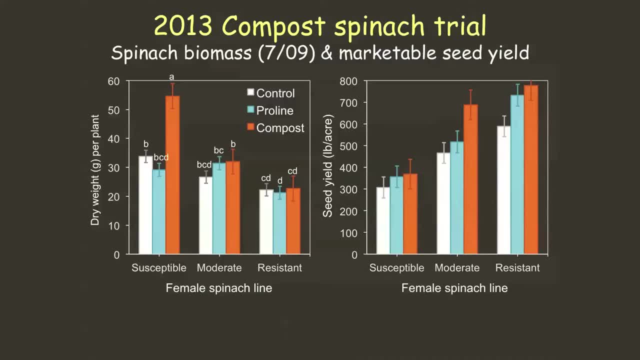 growers were harvesting potatoes. So they come in the field with those diggers and all the trucks with eight inches of rain on that soil And then you come back in the spring and wonder why you've got concrete and you're trying to grow spinach or table beets. So we 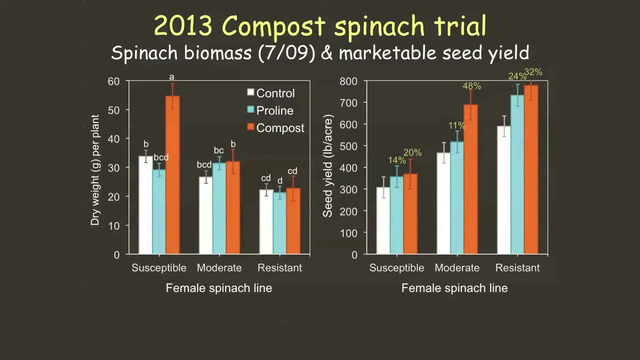 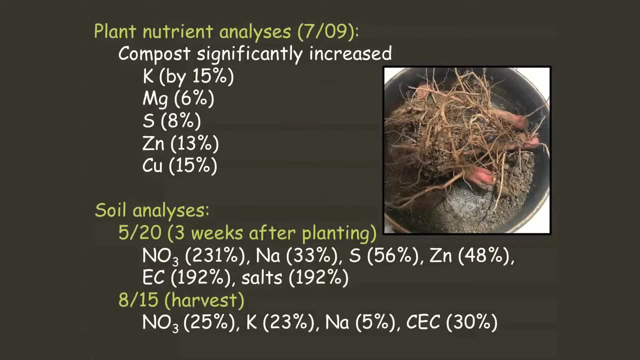 have huge problems with destruction of soil structure and soil health, And working with these kinds of practices to try and rebuild soil health has become quite critical. We looked at what was happening to these plants when we did the compost treatments and you can see there was quite a wide range of shift. 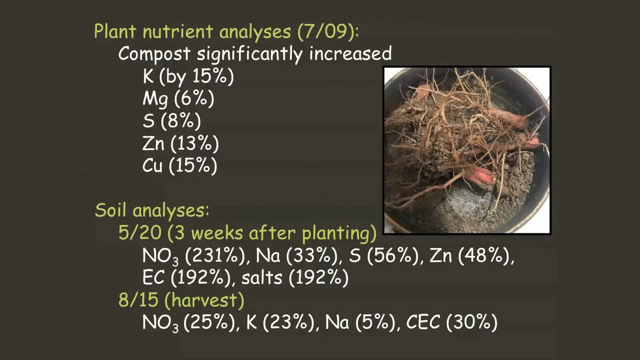 in the plant nutrient analysis An increase in potassium, magnesium, sulfur, zinc and copper. When we looked at the soil analyses by the end of the season, we still had 25% increase in nitrate, 23% in potassium. 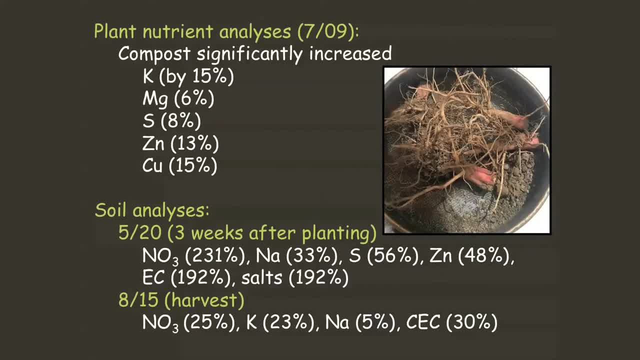 sodium and cation exchange capacity And I don't have a picture here, but the fine roots of those spinach plants were much more extensive in the compost treated plots Which really showed the benefit of that compost in helping rebuild soil structure and soil tilth. And we're seeing this. 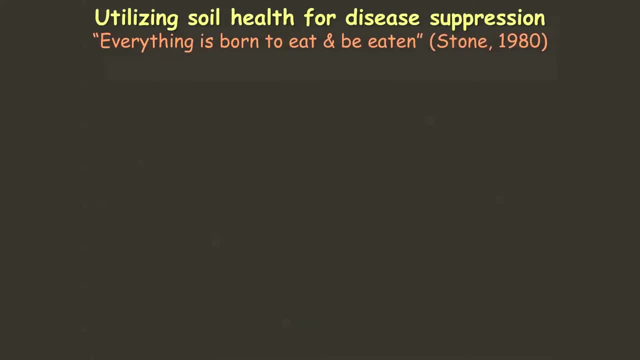 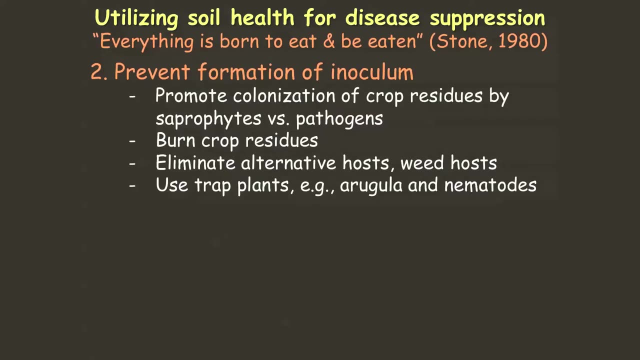 repeatedly when we carry these trials out with table beets and spinach. So getting onto the second protocol of using, trying to utilize soil health for disease suppression. second aspect is preventing formation of inoculums, So promoting colonization of the residues after harvest by competitors with 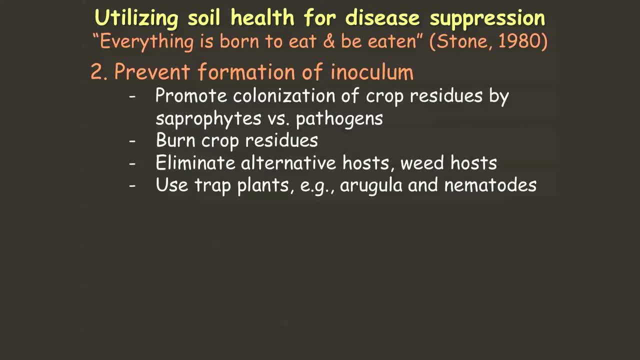 pathogens, in other words saprophytes. Burning crop residues has been one way that people have historically helped reduce disease: Eliminating alternative hosts, including weeds, and using things like trap plants in the case of nematodes, where they infect the plant but aren't. 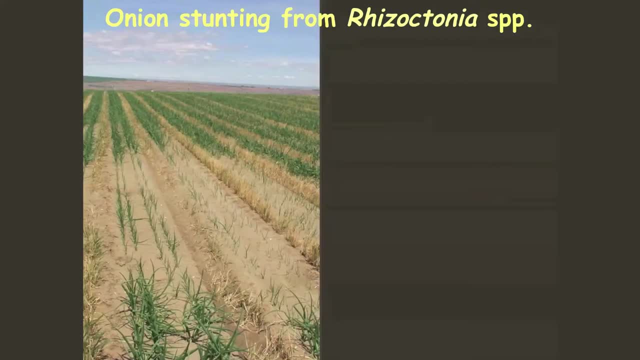 able to reproduce, And I'm going to use to illustrate this, a disease we've worked on in onions in the Columbia basin, which is called onion stunting. It's caused by Rhizoctonia species And it's only a problem on the very. 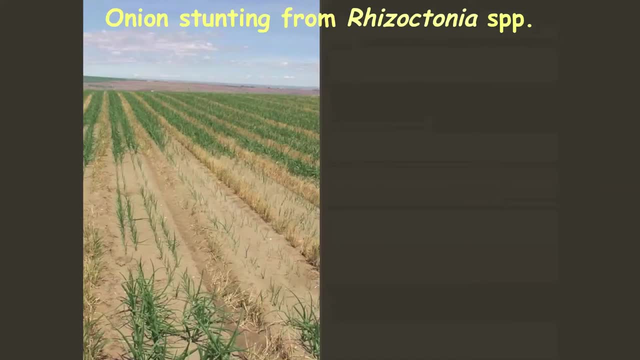 coarse sandy soils, mostly in the south basin, but also some areas in the Black Sands area up here, Where, you know, in windy conditions the sandblasting that can occur on the onions has now necessitated the use of these cereal cover crops. 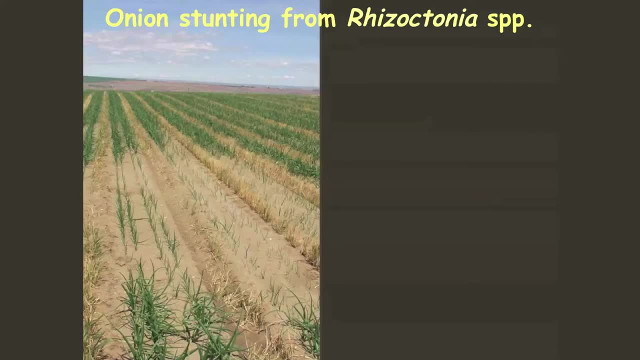 winter cereal cover crops. They're then sprayed with herbicides and onions are planted directly after that. Unfortunately, in these very coarse, sandy soils, organic matter is very, very low And if you have Rhizoctonia present, there's no competition. 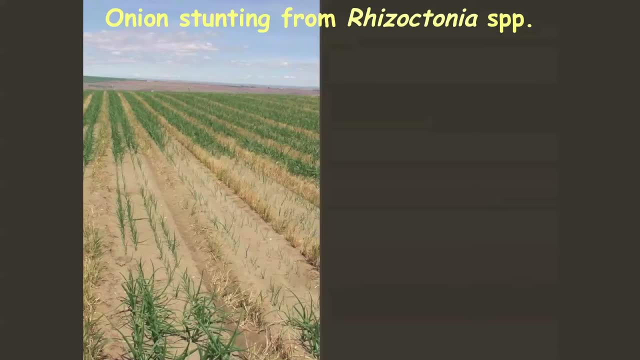 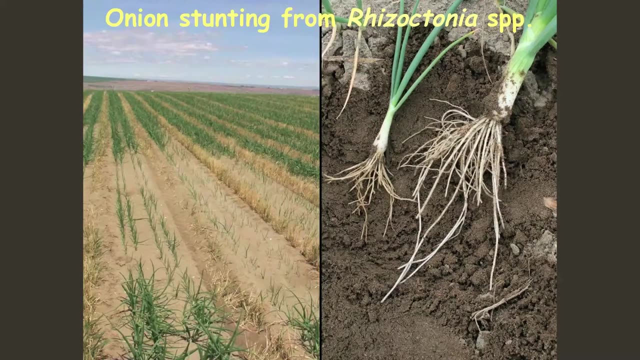 Because there's not a lot of other fungal flora And Rhizoctonia is a very rapidly growing fungus And you end up with these stunted patches. Here's a picture of a stunted seedling next to a healthy seedling or onion plant. 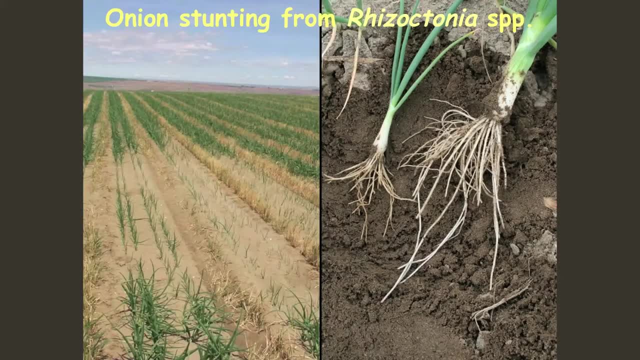 And the Rhizoctonia nibbles away on these roots because it's got no competition at rapidly colonizing the cereal roots that you've just killed with a herbicide. There's no resistance there, It doesn't matter how tolerant that cereal might have been. 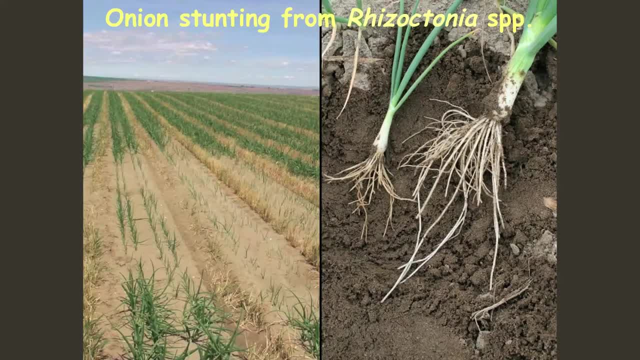 Once you kill it with a herbicide it just goes crazy and colonizes And then you see a shift as other microbes start to colonize that decaying material And what we've discovered from work down in the Palouse is that increase in Rhizoctonia. 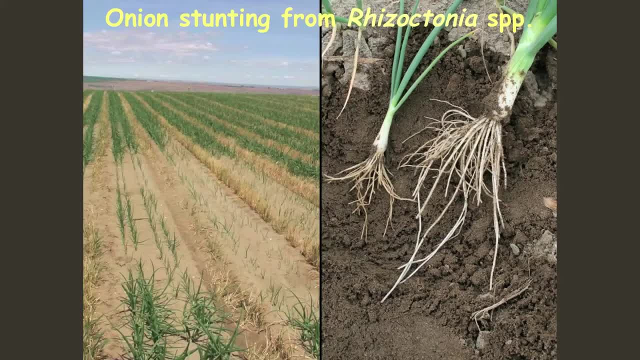 is very short. It's about a two to three week window. So understanding that has helped us figure out how can we utilize that information. We're not going to get away from having to do a cover crop preceding these, Otherwise we have to replant from all the. 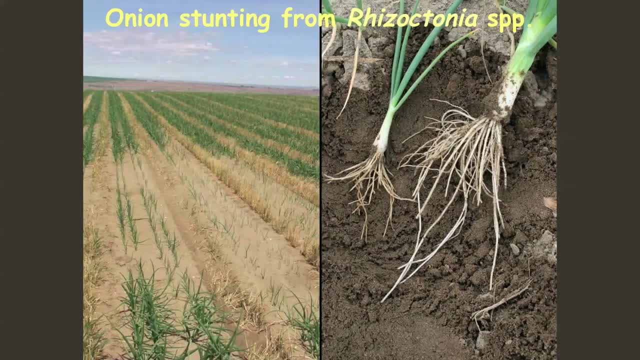 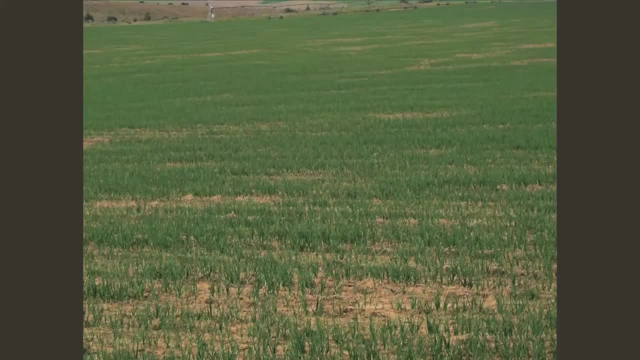 sandblasting. So how do we take advantage of this knowledge that the Rhizoctonia increase is very short term? It's a temporal peak that only lasts for two to three weeks. This is a picture of an onion field. I don't know if you can see all the 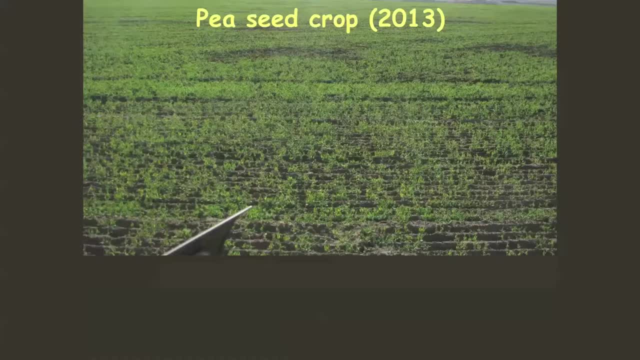 UFO landing black spots all over the field. This is a picture of the same problem in a pea seed crop I was asked to look at in 2013.. The grower had a winter wheat cash crop growing and was approached by a seed company and said: can you kill your wheat crop? 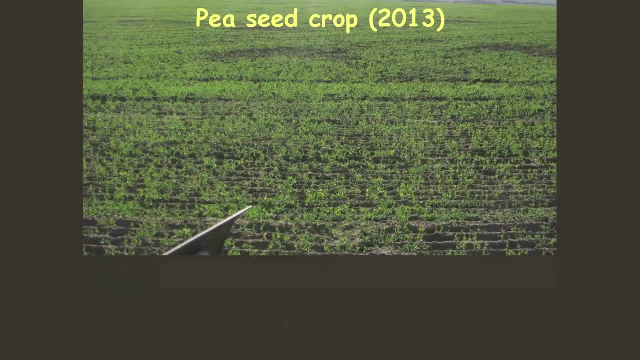 and we'll pay you to grow a pea seed crop. So he had this beautiful winter wheat crop that he killed out with a herbicide in the spring and two days later were incorporated and two days later came back and planted peas- Absolute, worst thing you can do for Rhizoctonia. 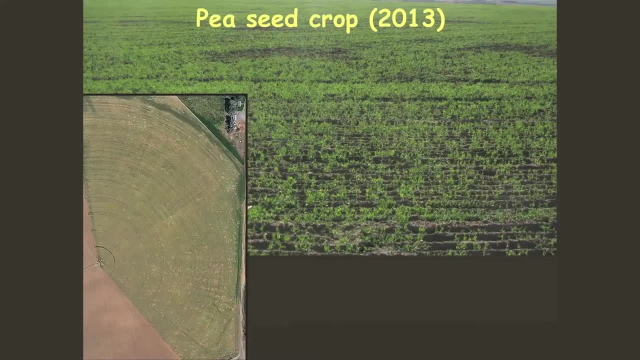 This is what the field looked like from an aerial image. I'm not sure if you can see all those little spots all over that field. All those little spots are patches that might be as much as 15-20 feet in diameter of stunted plants from Rhizoctonia. 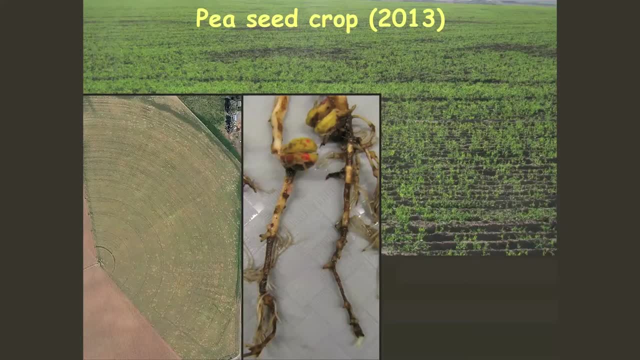 And this is what the roots look like. So you know we did everything you'd think. incorporating that organic material would be beneficial, but understanding what it does to the shift in microflora is really important. so we can avoid this kind of situation. If the grower had waited two weeks. 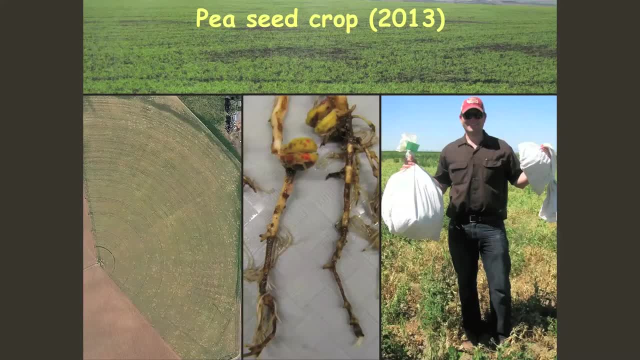 he probably would not have had this loss And this shows the pea seed that we harvested from inside a patch versus in a healthy area in that field. So very, very significant yield loss And really all related to that cover cropping system that in this case wasn't really a cover crop. 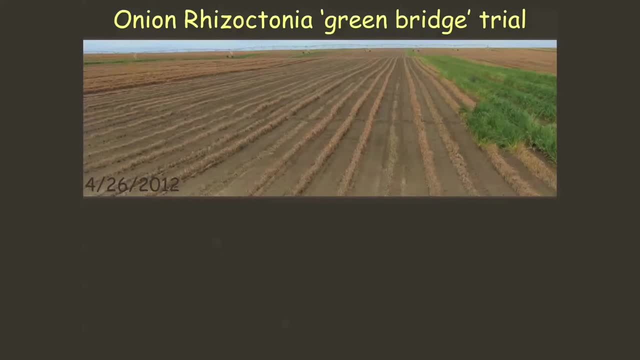 it turned out to be So. we did a trial with a farm down in the south basin, looking at what we call a green bridge trial- although I like to call it a brown bridge trial, but my collaborator doesn't like that word- Because we want to. 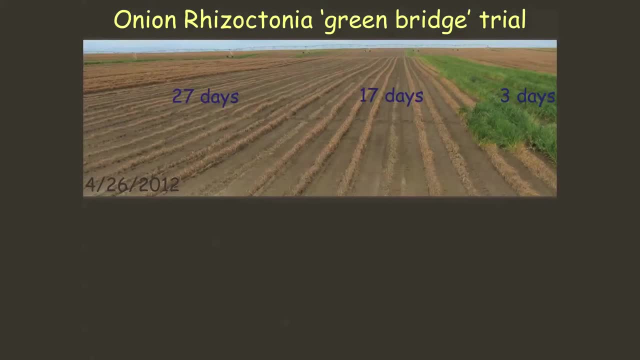 look at if we spray out the cover crop, say, four weeks before planting onions, or two weeks before planting onions, or just before planting onions, do we see a difference in the amount of disease? And this is just an illustration of one year of the trial. each plot was 12 beds. 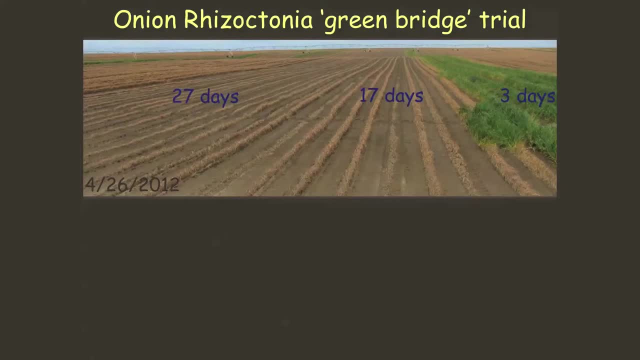 wide the entire diameter of 125 acres circle and there were six replications So we walked nine miles every time we raided the trial. because the disease is so scattered you have to have big plots to make sure you encounter the disease somewhere in there. So I told 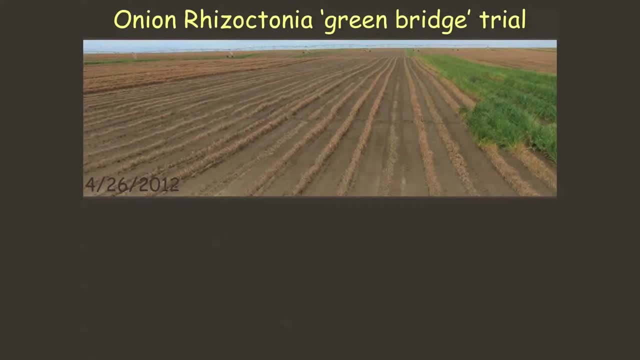 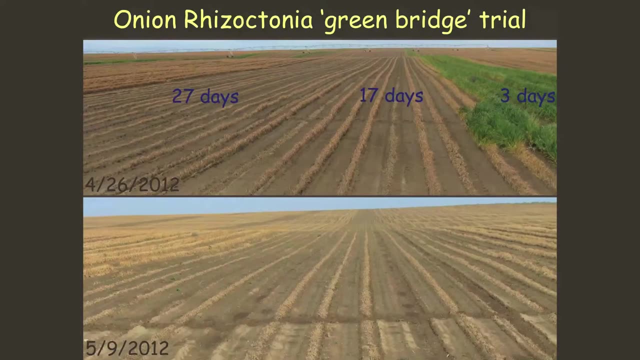 my workers and students. you don't need to join a gym. when you come and work in my program, We'll give you a workout. So there you can see the plots. this plot was sprayed out 27 days prior to planting onions, 17 days and 3 days, and this photo was 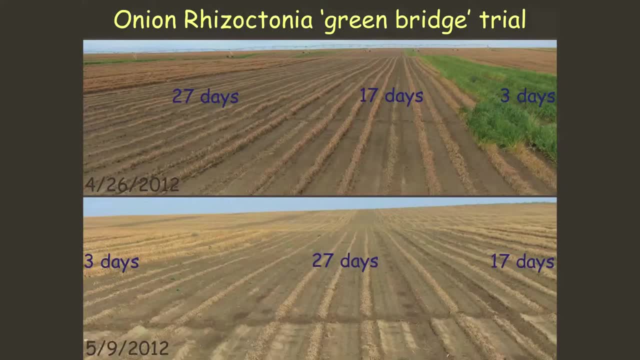 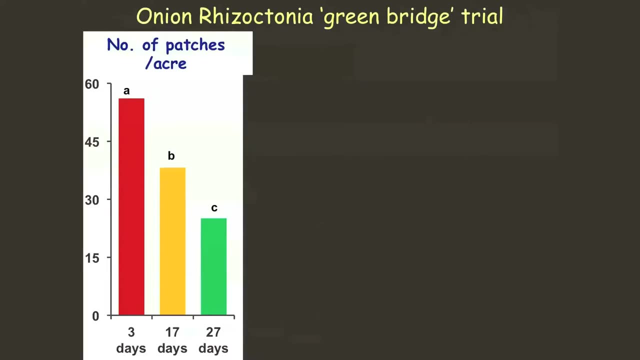 taken just after onions were planted, and then, about 10 days later, you can see the cover crop died back, and you can see the replicate strips of the different treatments across the field. And so what did we find? This first image shows, on the y-axis, the number of patches. 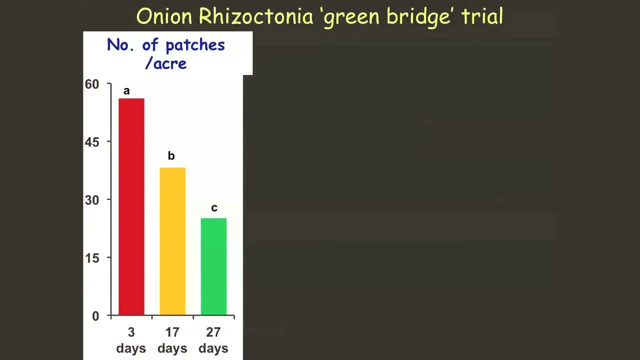 per acre that we measured in the plots that were sprayed out just before planting onions, or about 2 weeks before planting onions, or about 4 weeks before planting onions, and you see a very significant decline in the number of patches per acre just by waiting for that material to break down. 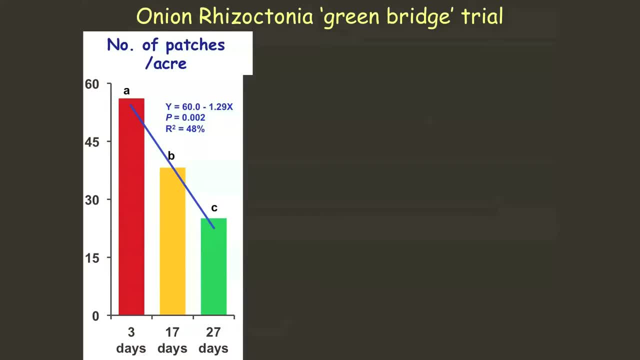 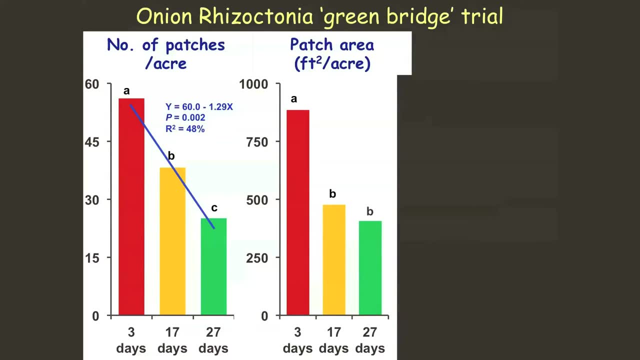 and the shift of a peak of rhizoctonia to go away and have the secondary microorganisms come in and replace that rhizoctonia. And likewise with the cumulative area of patching per acre, we got more than a 50% reduction in the area of 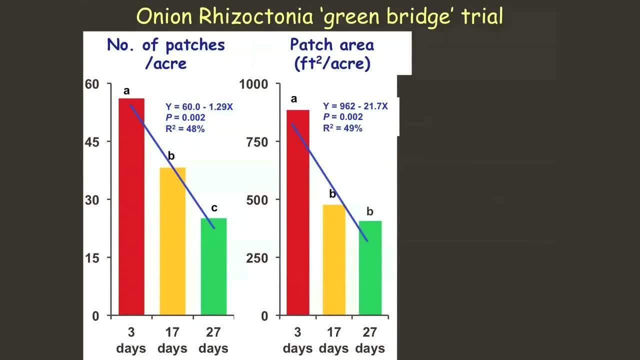 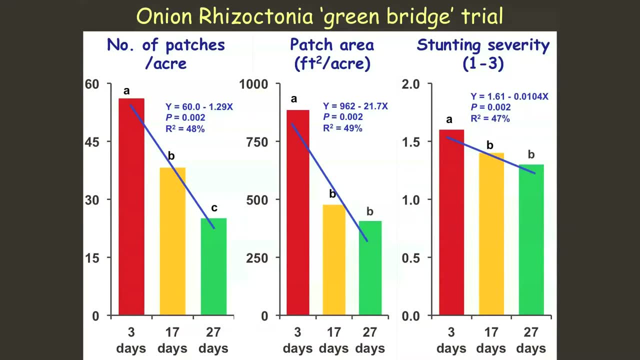 patching, just by waiting 2 weeks to 4 weeks before planting onion seed, And then with the severity of denting within those patches it also was reduced significantly. So I hope that kind of gives you an illustration of the complexity I'm trying to. 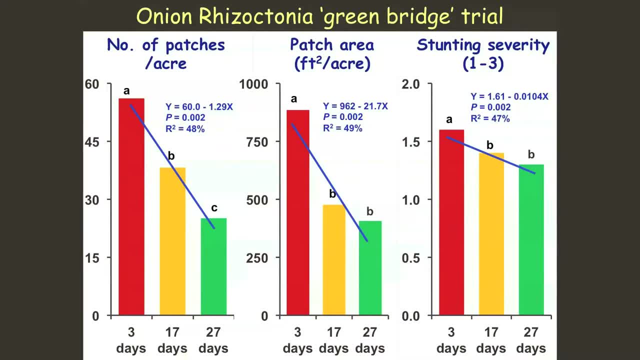 illustrate here of what we talk about when we mention soil health. Cover cropping is supposed to be very beneficial, but if you understand what it's doing to the microflora, you can try to avoid these kinds of high risk scenarios. Okay, the third aspect which is displacing. 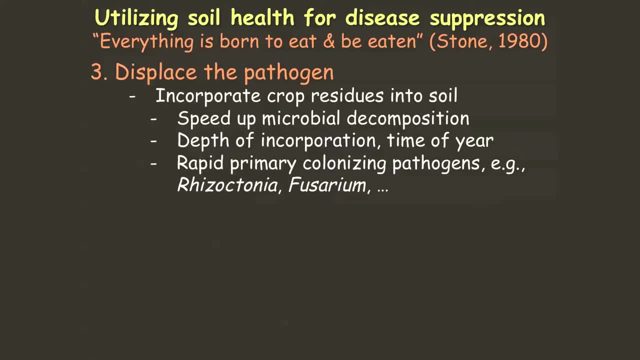 the pathogen. Things like incorporating the crop residues after harvest into the soil Instead of leaving them on the surface. now, This kind of contradicts the idea of no-till. But when it comes to soil borne pathogens, if residues are incorporated into the soil, 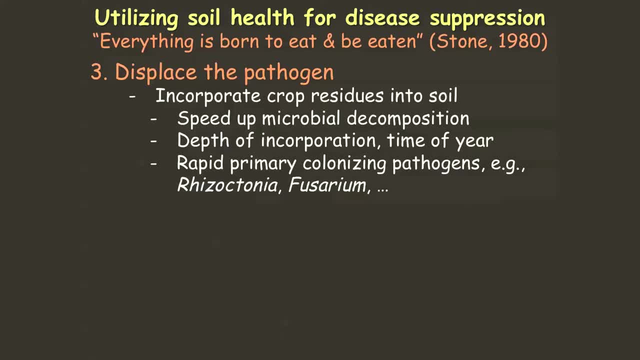 the soil microflora will break down those residues much quicker than if the residues are left on the surface. So in situations where you know you're dealing with a soil borne pathogen, this can be a beneficial move towards helping displace the pathogen and break down that. 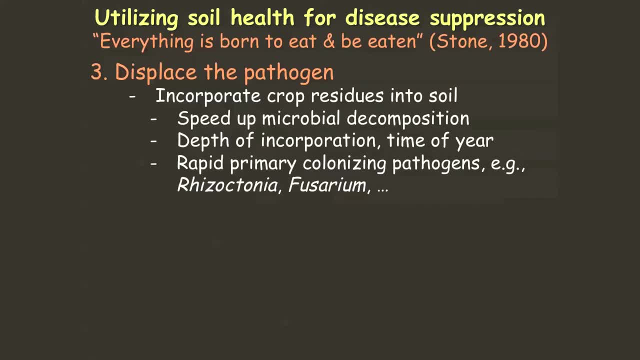 inoculum. Obviously, this is a conflict with the issue of reduced tillage, so this has to be held in balance with that achievement, if that's part of your plan. But that's why I recommend this. in situations where you know you have a pathogen, that this can be very effective. 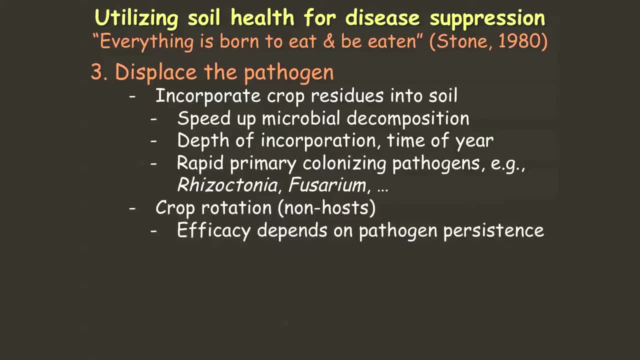 for reducing inoculum, That's. crop rotation is another example of how you can displace the pathogen. The length of that rotation is going to vary widely depending on how persistent that pathogen is. The spinach fusarium wilt is an extreme case. 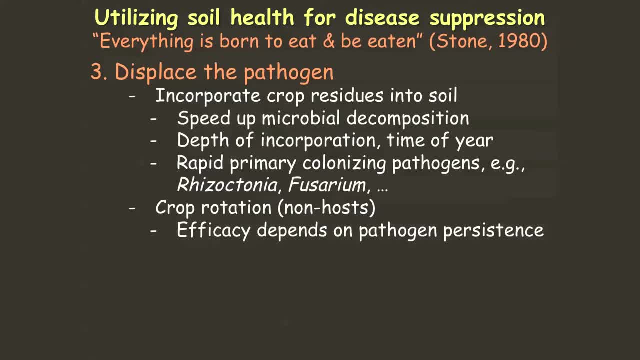 Onion white rot is another extreme case. You're talking 20-30 years. A number of like white mold in potatoes. you know four or five year rotation usually suffices because the sclerotia will break down unless you have a susceptible host in that rotation. 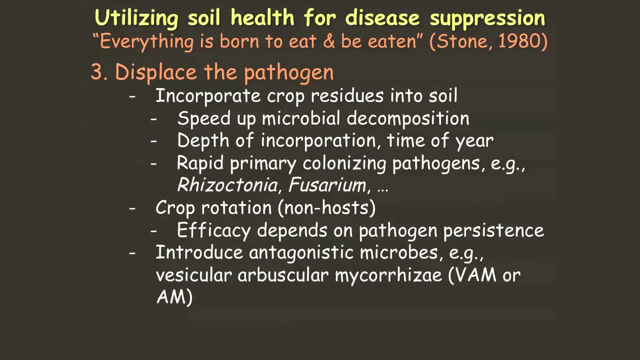 And then you can introduce antagonistic microbes that will help displace those pathogens, and I'm going to use an example here, which is the albascular mycorrhizae, or mycorrhizal associations with plants- Mycorrhizae most of you are probably. 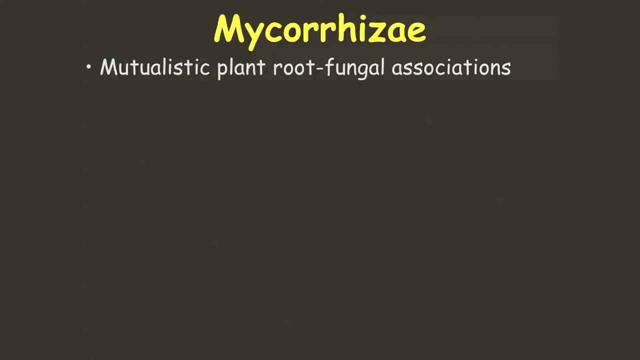 familiar with this. but just in case any of you aren't too familiar with mycorrhizae, they are a beneficial association between a fungus and the plant or multiple fungi and the plant roots, Mycorrhizae. the fungi are present in most soils. 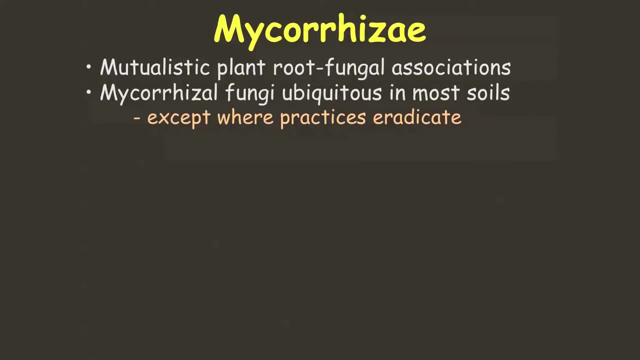 except where we've done things that kill them off, And agriculture can contribute to that, for example soil fumigation. Almost all plant species form mycorrhizae, except two very notable exceptions- Plants in the Caenoportyaceae sugar. 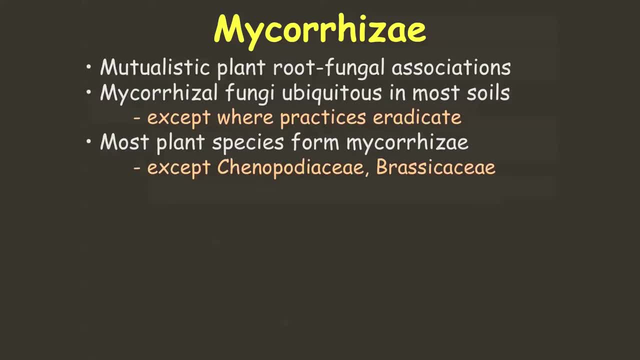 beets, table beets, spinach- they do not form mycorrhizae. And the brassica caseae- they do not form mycorrhizae. So unfortunately, mustard cover crops don't form mycorrhizae. So when you use a mustard, 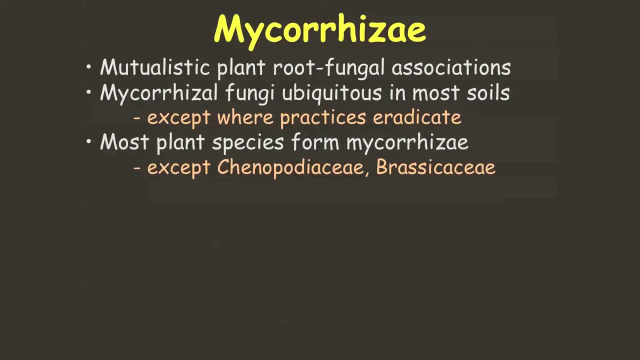 cover crop and you get that biofumigant effect. there's a huge benefit to it, but one benefit it doesn't provide is that it can actually reduce the amount of mycorrhizal inoculum in your soil because, A- it's a biofumigant and B- it doesn't form. 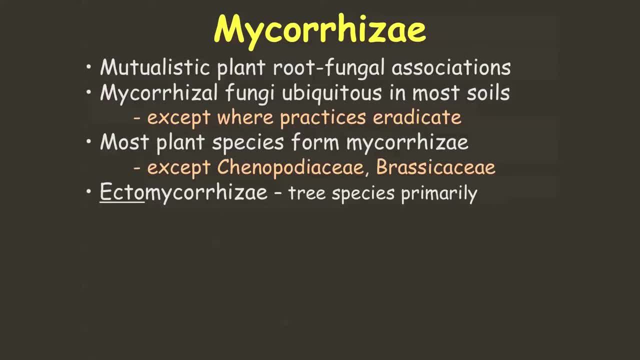 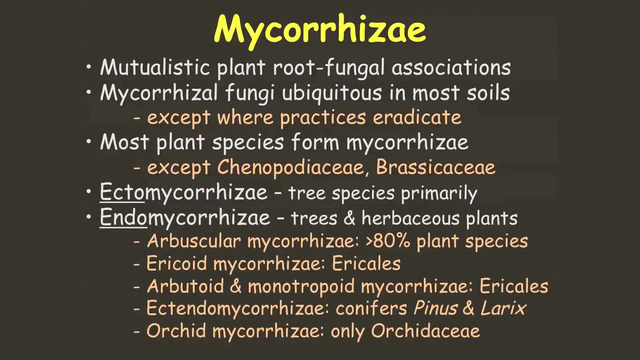 mycorrhizae. We have a lot of brassicas grown in the Columbia Basin And mycorrhizae divide into two categories: ecto and endo mycorrhizae, The ones we deal with in agriculture, unless you're dealing with tree species or 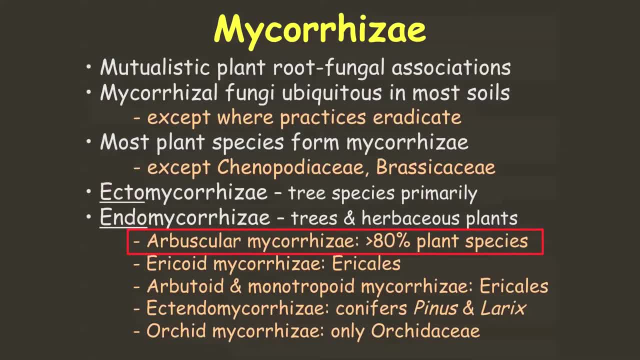 the endo mycorrhizae and, in particular, this group that we call the orbascular mycorrhizae, and I'll explain to you why they have that name. But more than 80% of plant species form associations with orbascular mycorrhizae. 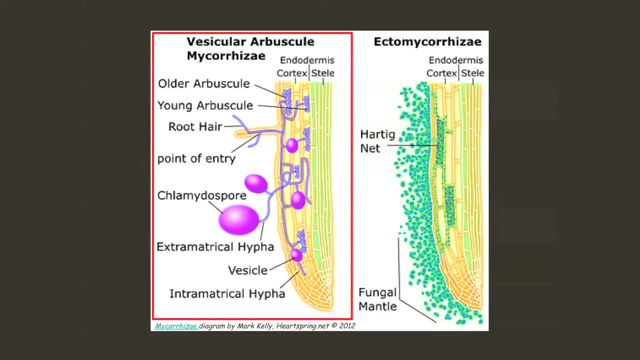 And just to illustrate this, I won't worry about the picture on the right because that's ecto mycorrhizae, which is not as relevant to cropping systems, but the vesicular orbascular mycorrhizae, the spores in the soil will. 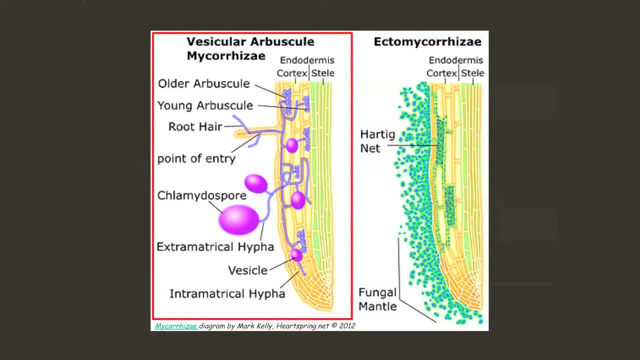 grow with hyphae and penetrate the root. hairs grow inside the root and they'll form these structures called. there's a small one and an older one, and this is the working end of these mycorrhizae. That's the structure that forms a very close association with the cell. 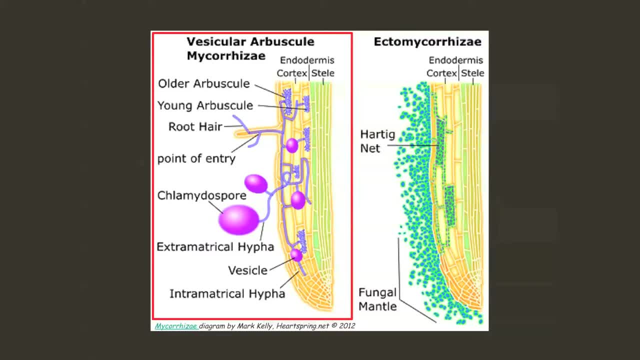 and absorbs photosynthates from the cell, from the plant. so it's taking its nutrients from the plant. But the hyphae that grow out into the soil increase the ability for that plant to take up water and nutrients. So you have a huge increase in the absorptive surface area. 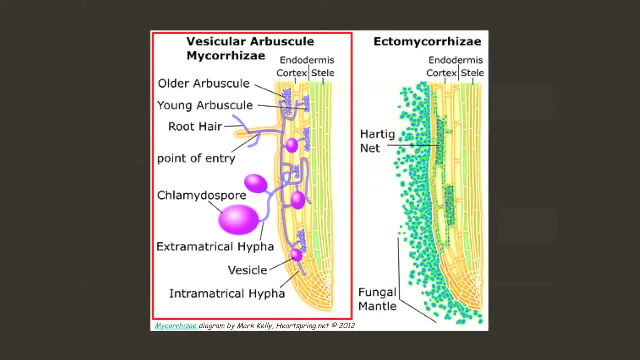 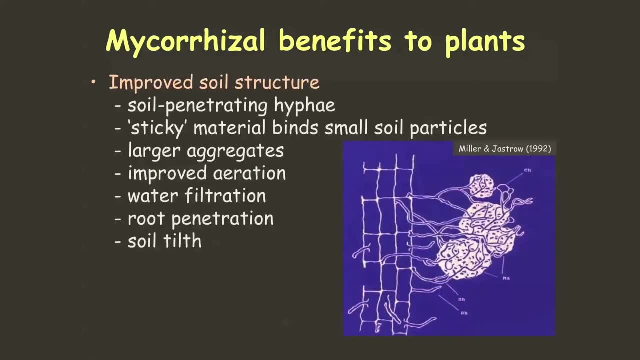 of the root system of a plant as a result of those hyphae that grow out into the soil. So it's a mutual exchange of benefits between these two. How does this benefit plants? Well, one of the very obvious features is it does improve soil structure. 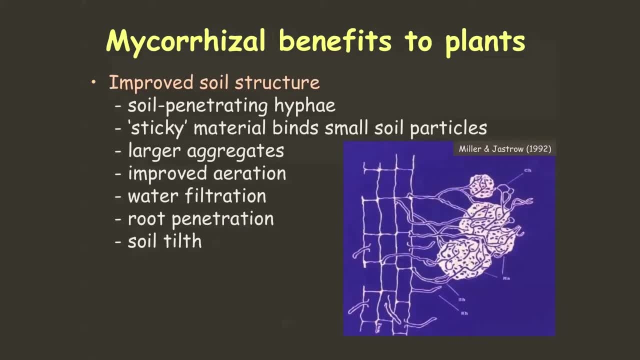 The soil penetrating hyphae release a sticky type of matrix that binds the smaller soil particles, creates these aggregates. When you start getting aggregates, your soil structure improves, it improves aeration, improves water filtration. that was one of the priority issues that we talked about the need for these soil. 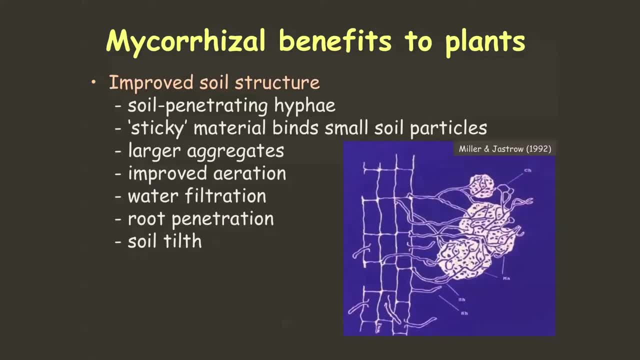 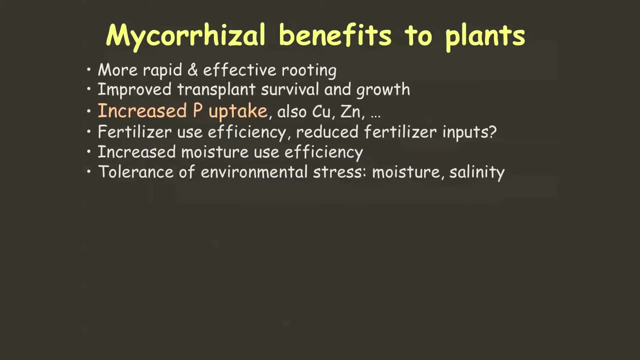 building practices. That improves root penetration, A very definite benefit of mycorrhizae. You can get more rapid and effective rooting because of that extensive hyphae system that goes out into the soil much faster than the plants roots themselves, And this can really improve. 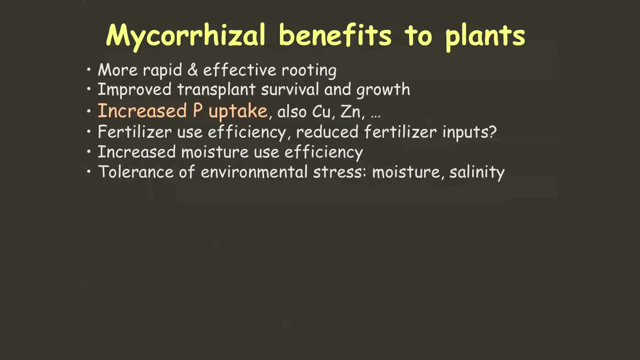 if you're doing transplanting, improve transplant survival and growth if you're dealing with those kinds of crops. It also one of the very well known benefits of mycorrhizae is increasing phosphorus uptake, Because it's able to scavenge phosphorus out of the soil. 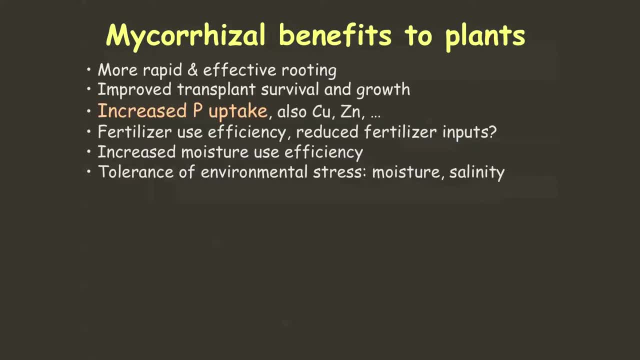 including from unavailable forms that the plant normally can't access- As well as other nutrients, And I've heard reports from growers- not necessarily here only, but that they've been able to reduce their phosphorus use significantly- 50-75%- by taking advantage of mycorrhizal. 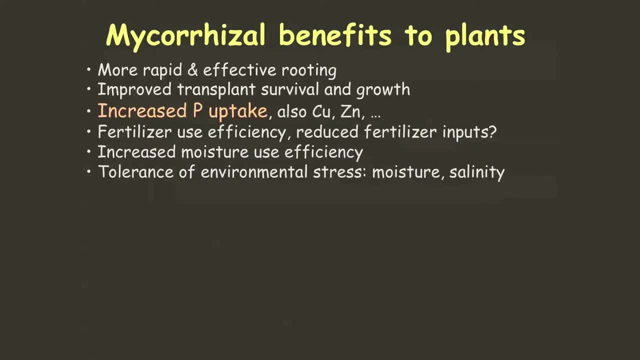 inoculants. That's anecdotal evidence, but that's the theory behind how these mycorrhizae in particular have a benefit. So you can get increased fertilizer use efficiency and potentially reduced fertilizer inputs and increased moisture use efficiency because of those hyphae penetrating. 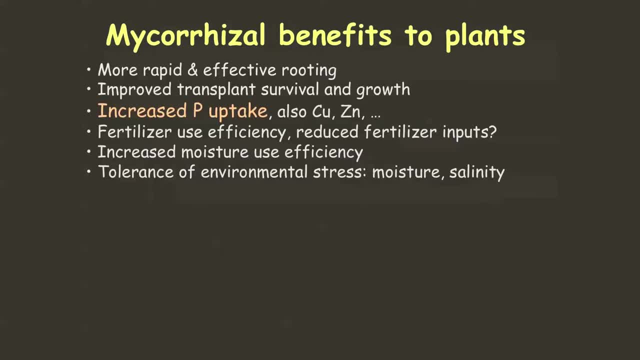 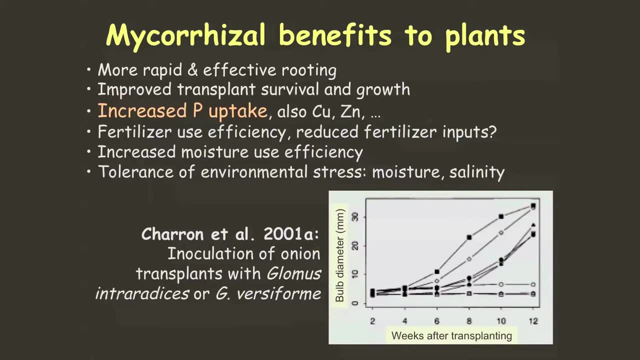 out into the soil, Which translates into a greater tolerance for environmental stresses. I'm just going to give you one paper that I- there's a lot of papers on mycorrhizae in agriculture- but one I used in a presentation I gave last week at the National Allium. 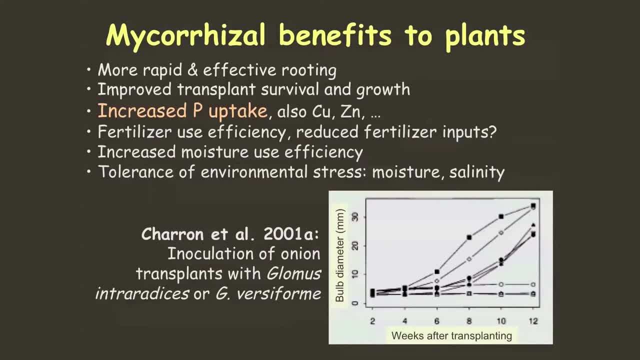 Conference A study that was done in early 2000, where they inoculated onion transplants with two different species of mycorrhizae, Glomus centroradices and Glomus versiforme, And they looked at the weeks to maturity after. 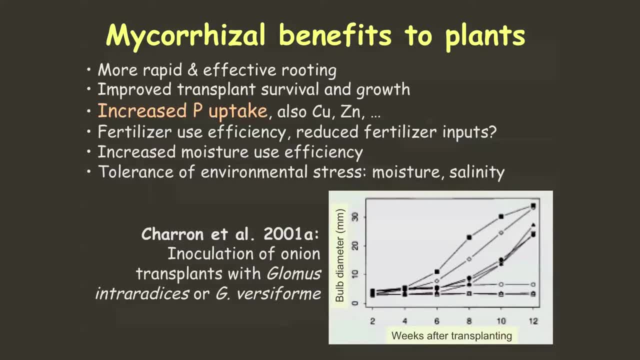 transplanting and bulb diameter, And I don't have a key here, but there's a lot of information about that. So the flat lines at the bottom are the non-inoculated, where they didn't put mycorrhizae out after transplanting. 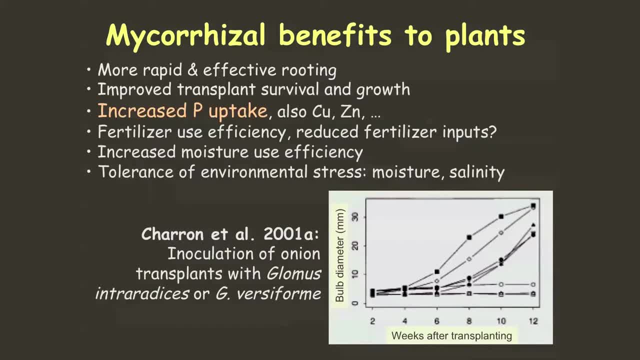 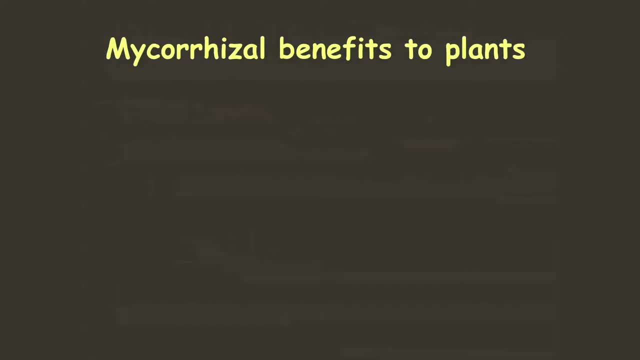 And the lines that go out quickly show you, in the presence of these mycorrhizae, how much quicker those onions matured and bulbed- And you know if you're an onion grower- the quicker you can get your crop to maturity, the better. 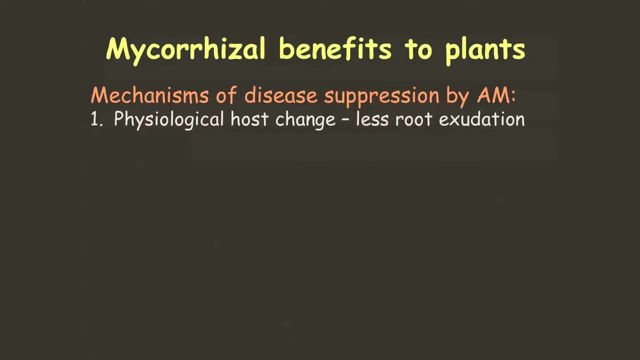 How do mycorrhizae help with disease suppression, since that's the topic of our presentation? They bring about a physiological change in the host. as a result of that association with the roots, You get a lot less exudation. Now, root exudates are. 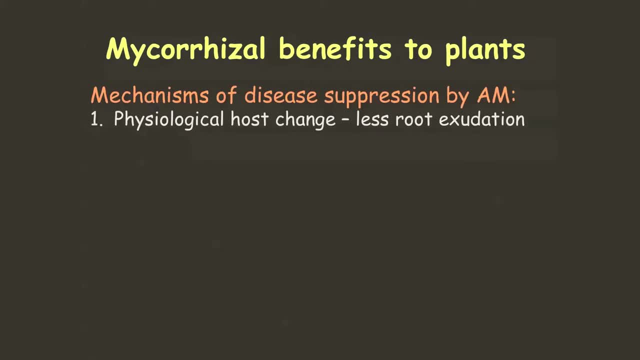 one of the key ways that pathogens are attracted to roots. The exudates that roots give out will attract things like pythium. Pythium spores in the soil will chemically sense those exudates and germinate and swim towards the root if it's. 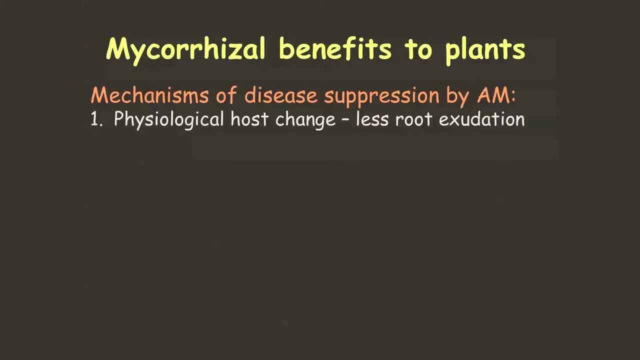 a pythium or other fungi like white rot in onions or sclerotinia will germinate in response to the presence of these root exudates. So mycorrhizae help reduce that. The mycorrhizae also shift the soil microbes. 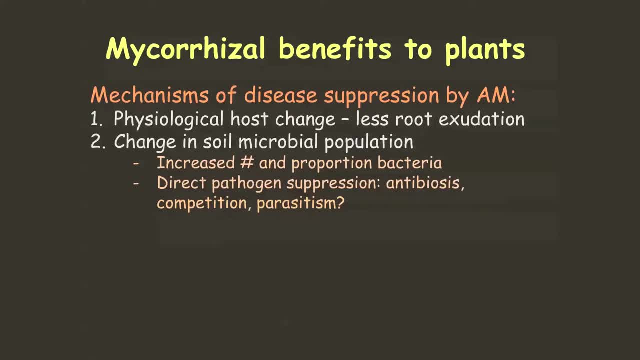 You tend to get an increase in the proportion of bacteria present in the soil and many of the antagonists of the plant- pathogenic fungi- are bacterial And you can get direct suppression as a result of these bacteria producing antibiotics or competing, or even parasitizing in the case of some. 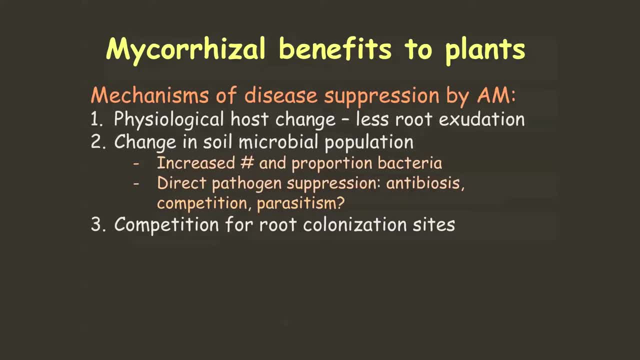 fungi, The mycorrhizae, colonize the roots and they compete with the pathogens for root colonization sites And we've got some really nice data showing, when we inoculated onions or grew onions in soil, that we added mycorrhizae to that. 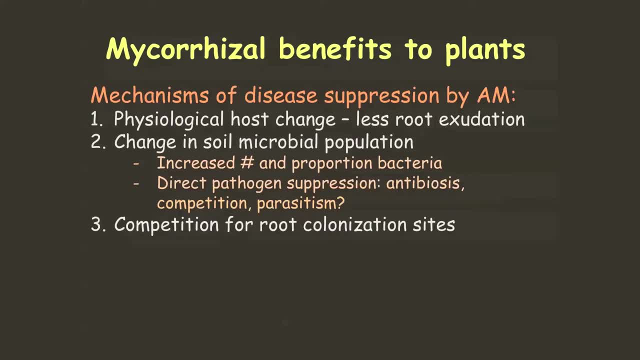 rhizoctonia wasn't able to cause the degree of loss that we'd seen without the presence of mycorrhizae, And this relationship between the fungus and the host apparently induces a defense response in the host. so when it is infected by a pathogen, 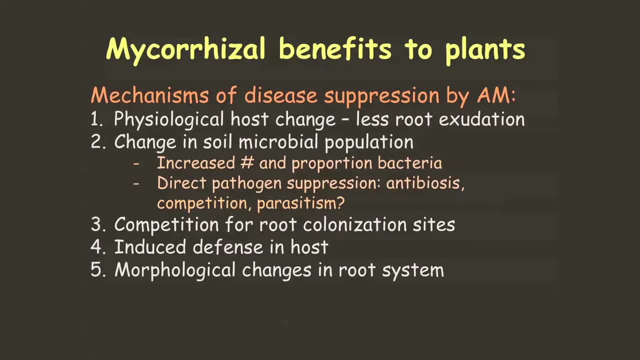 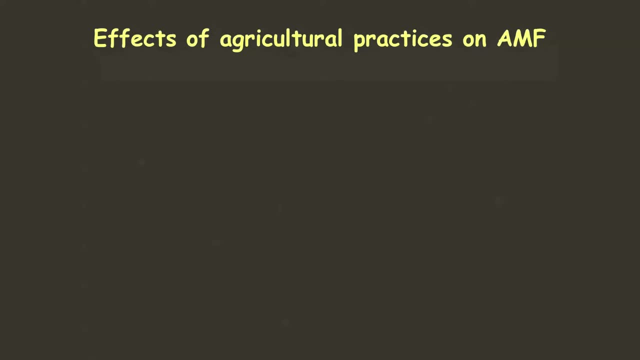 those defense responses are already triggered, Kind of like almost a vaccination, And there's morphological changes in the root system. that very extensive network going out into the soil helps the plant tolerate the stress of those pathogens and damage compensation. Now this is where we have to think hard. 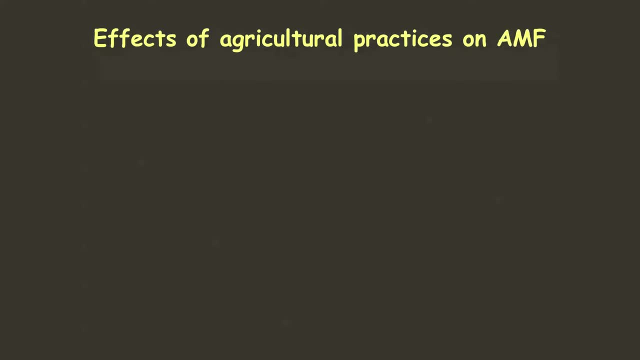 about mycorrhizae You'd think, well, that's a silver bullet. why don't we all use mycorrhizal inoculants? it solved all of our problems, But the reality is a lot of our agricultural practices can be have negative. 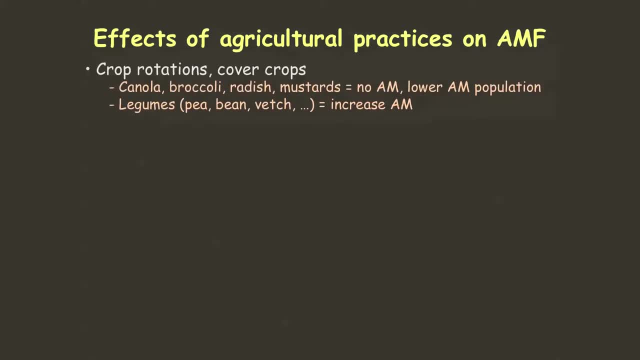 impacts on mycorrhizae, Crop rotations and cover crops can be beneficial or can have a negative impact. I mentioned that the brassicae do not form mycorrhizae. Some of them are by fumigant type crops and they will lower the mycorrhizal populations. 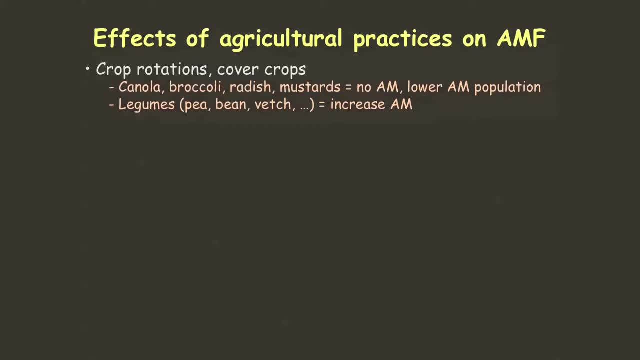 in soil And it was interesting when we started surveying onion crops, organic and conventional. I was expecting to see a lot less mycorrhizae in conventional onion crops because of all the fumigation that's done in onions and to see 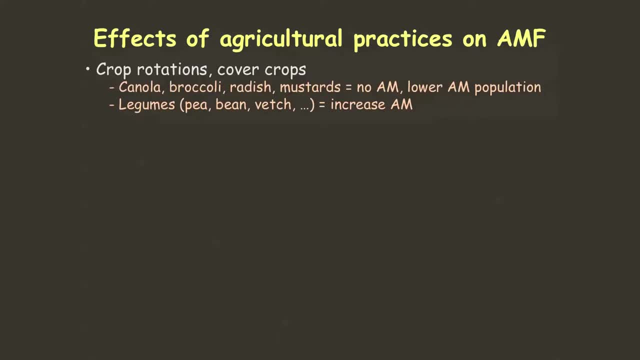 a much higher level in organic, But it turned out most of the organic onion growers are using these mustard cover crops, and so we actually don't see a difference in the amount of mycorrhizae in conventional versus organic. onion Legumes are very beneficial, so crops 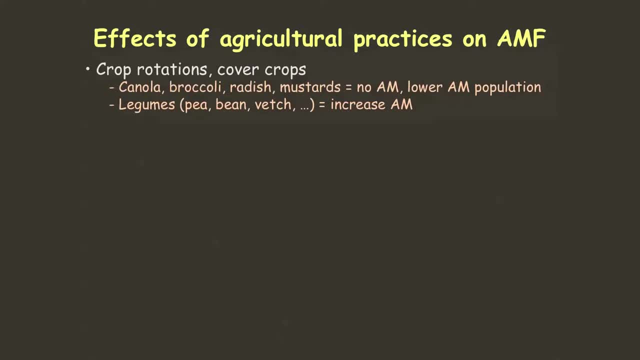 that do form mycorrhizae that also help introduce other beneficial microflora can play a major role in increasing mycorrhizae. The fertilizers we use in agriculture can have a big impact on mycorrhizae. Many species of 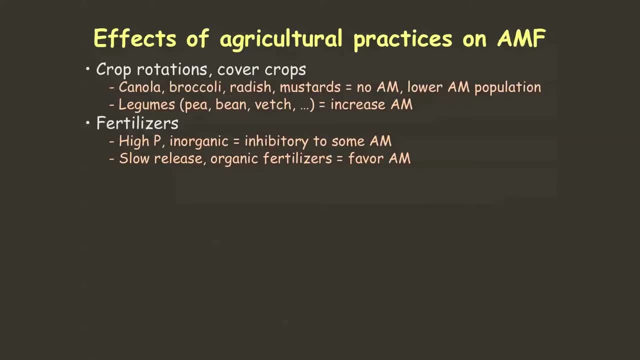 mycorrhizae are inhibited by high concentrations of phosphorus in the soil. Now, ultimately, that can be beneficial, because if you can establish good mycorrhizal populations, you don't need to use as much phosphorus, which is an important issue. 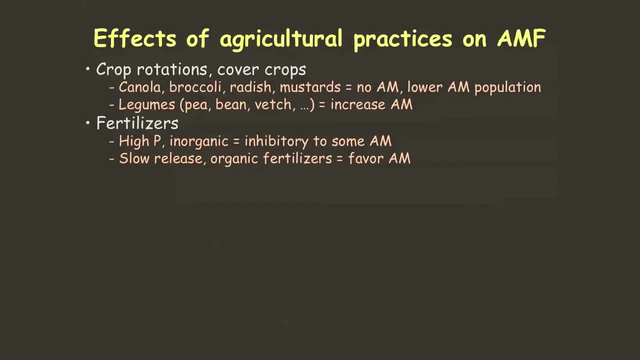 The slow release. organic type fertilizers do not seem to affect mycorrhizae adversely because they are slower release. There are mycorrhizae that can tolerate the presence of higher levels of phosphorus. Fortunately they're not all as effective, but that can be an issue. 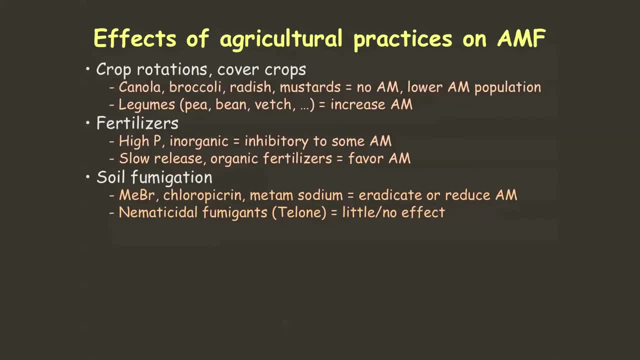 And of course the obvious soil fumigation, The very fungistatic or fungitoxic fumigants like methyl bromide, chloropicrin, methamisodium. they will kill mycorrhizae Again they might. 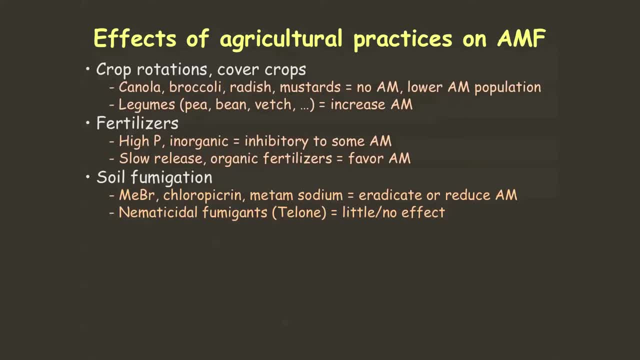 not kill them throughout this entire soil profile. so you'll get rapid recolonization of the soil as the new crop's roots reach beneath that fumigated zone, And nematicidal fumigants like telone are not going to have an effect on mycorrhizae. 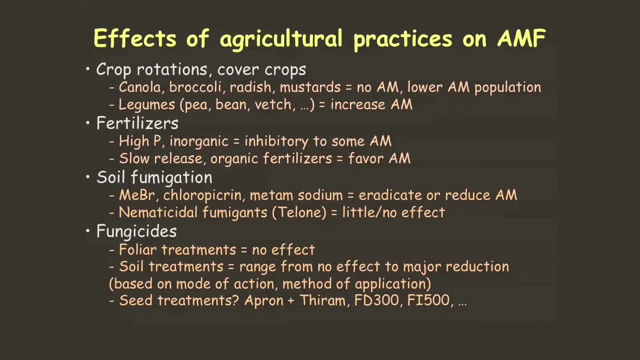 unless they have C17 or C13. Or C35 or something in there. A question that's come up a lot is fungicides. How might the fungicides we use in agriculture impact mycorrhizae And, looking through the literature, 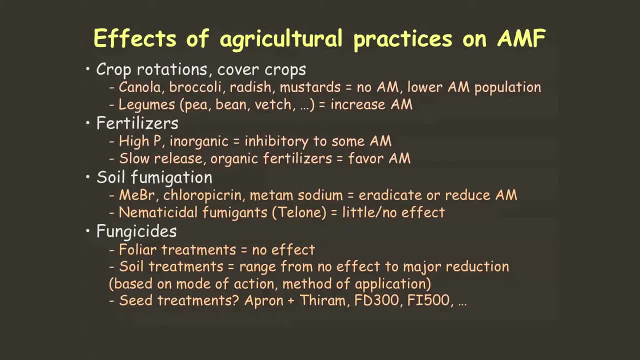 if you do fuller applications of fungicides you're not going to affect mycorrhizae because most fungicides are not truly systemic. They don't move in the flom down the plant, They move in the xylem one way. 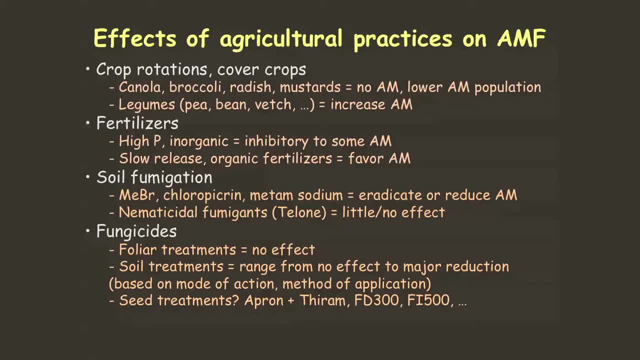 So if you apply them to the foliage, they go up, not down, And if you're applying the one that does move down, which is aliette, it's only specific to the oomycetes and mycorrhizae and not in that family of fungi. 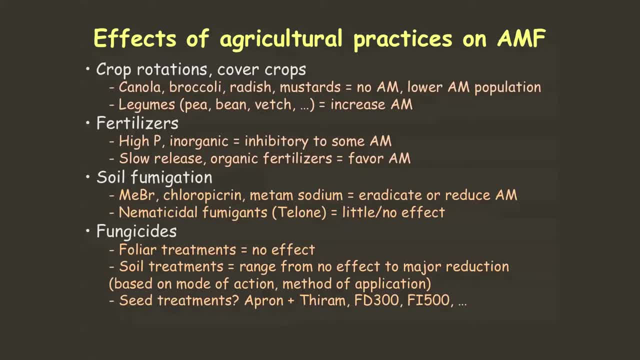 However, when it comes to soil treatments, you can have a range of effects, from no effect, depending on the mode of action of the fungicide, to very inhibitory effects, again depending on the mode of action, If you have these fungicides like the strobilurins. 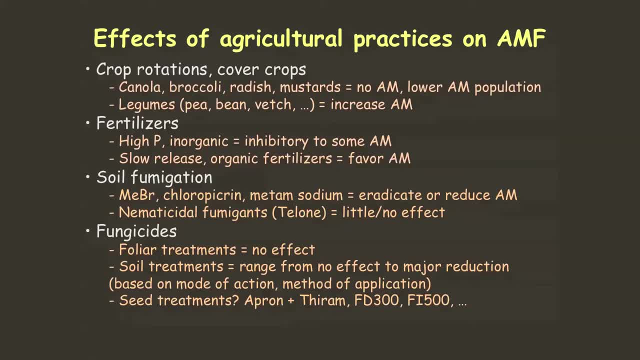 it's quite a concern. They're widely used. Quadris is used a lot in soil that it might have an adverse effect on mycorrhizae. So we're testing some of these treatments- Seed treatments In the case of onions I use because we're doing 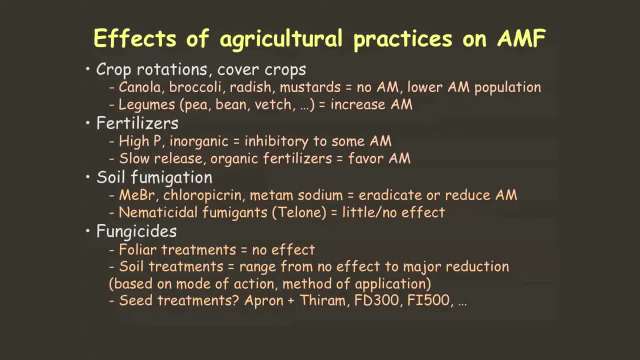 mycorrhizal evaluations in onions. FOMO D300 is very widely used, Now FOMO I500.. Are they inhibitory to mycorrhizae? Particularly many of these mycorrhizal inoculants you buy, you put. 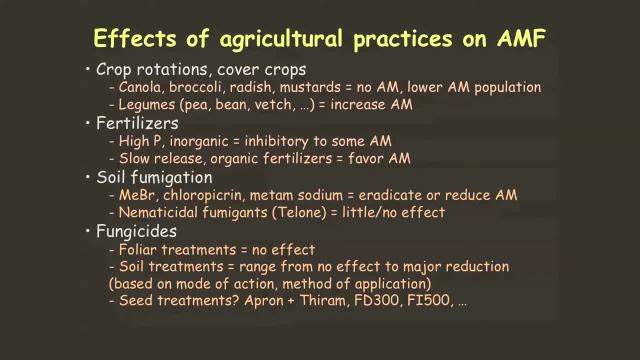 right in furrow or on the seed? What about those fungicides present? So we've been trying to take a look at that and I'll show you the data And cultivation. And you reminded me last time I talked about this, I left this important point off. 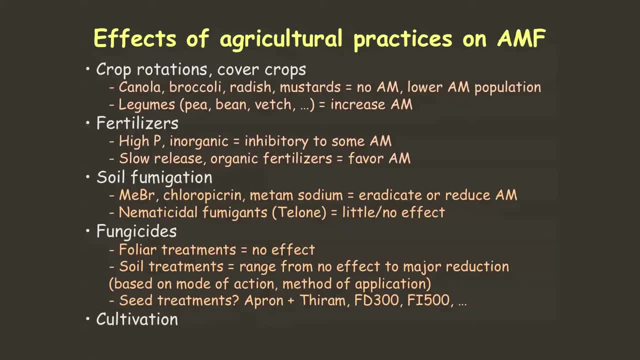 Anytime you disturb the soil you break up that extensive network of hyphae, of the mycorrhizae, and you do knock the population back. It will rebound quickly, but cultivation certainly does drop mycorrhizal populations. This is just a. 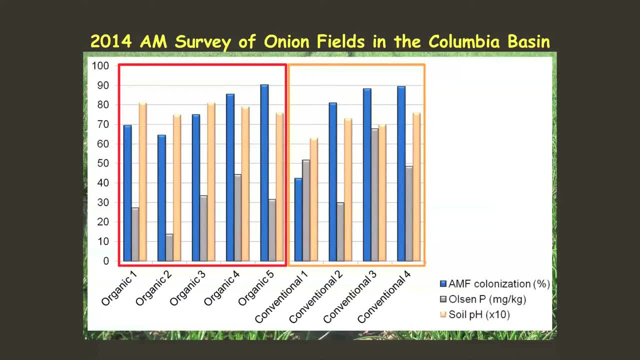 quick snapshot of some fields- organic and conventional onion fields that were going to be planted to onions. We surveyed for mycorrhizae- The blue bars represent the percent mycorrhizal colonization And we found it was widespread. I was very pleased. 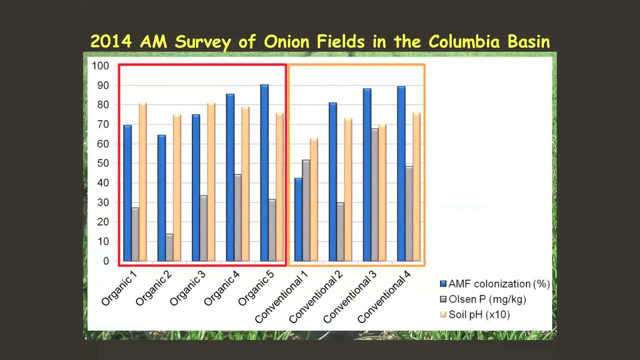 I was concerned that we'd find very little mycorrhizae because of how much fumigation is used in onion production. But this tells us mycorrhizae are pretty robust, They're good at bouncing back pretty quickly And the soil 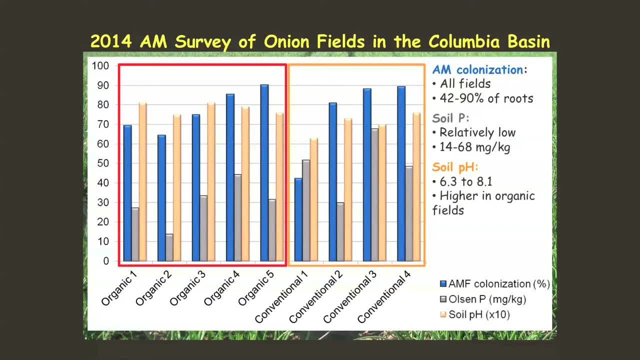 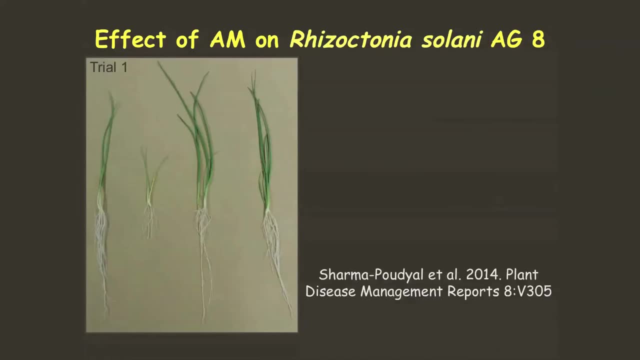 pH in these fields range from 6.3 to 8.1, the fields we surveyed. So even in the 6.3 field, which is a conventional two, we still got presence of pretty significant levels of mycorrhizae. Just to show you how: 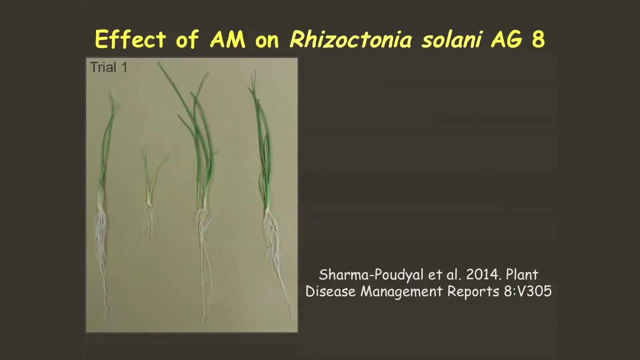 mycorrhizae can potentially affect a disease. this is a trial we did where we inoculated onions. The first onion on your left is control, no inoculation. The second one was grown in soil where Rhizoctonia was applied to the soil And you can see. 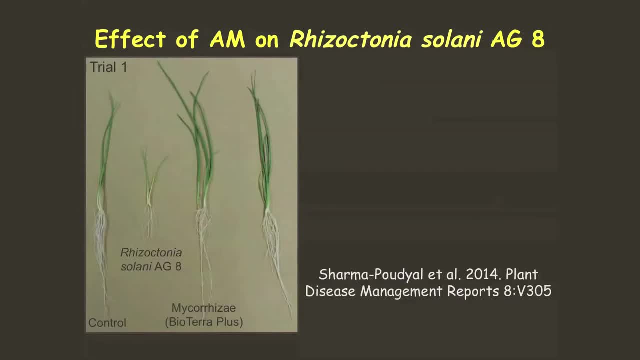 what it does. That's that stunting effect. When you add mycorrhizae to the soil in the absence of Rhizoctonia, you can see how the growth is enhanced compared to the control, And when you put Rhizoctonia. 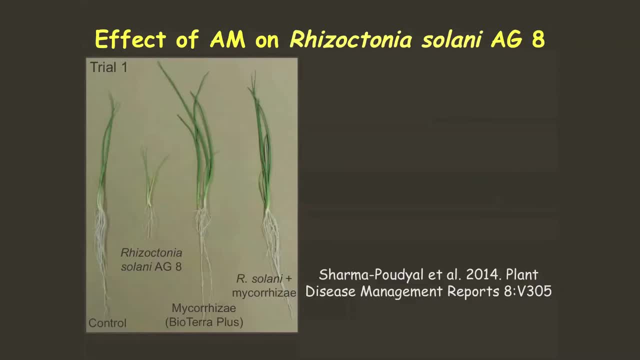 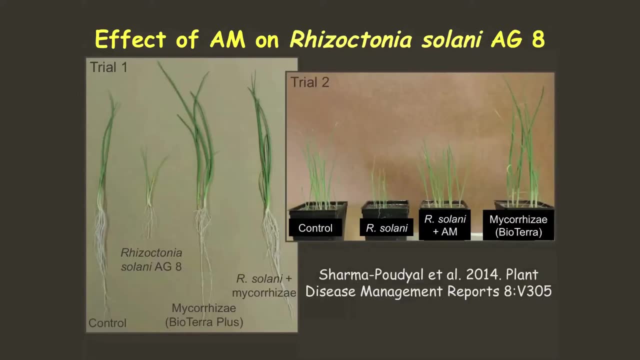 and mycorrhizae together. you have no stunting, And we've done this repeatedly in the greenhouse. Now we're trying to figure out how to get formulations of mycorrhizae that can be used by onion growers, And this just shows it again in a trial. 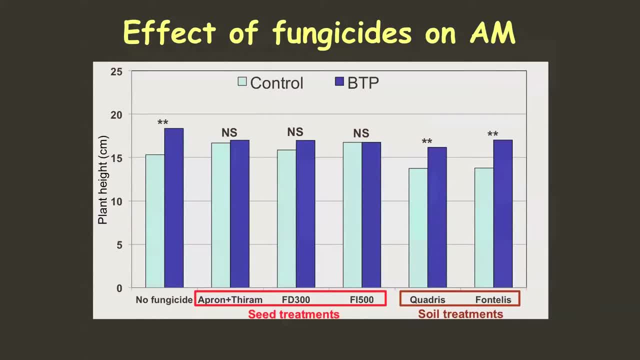 we repeated. I mentioned this issue of fungicides. So we planted onion seed in soil that we, where the seed was treated with Aprenthyrum or the FD300 or the Fi500. Or we treated the soil with Quadrus or with Fontalis, two products that are increasingly being used. 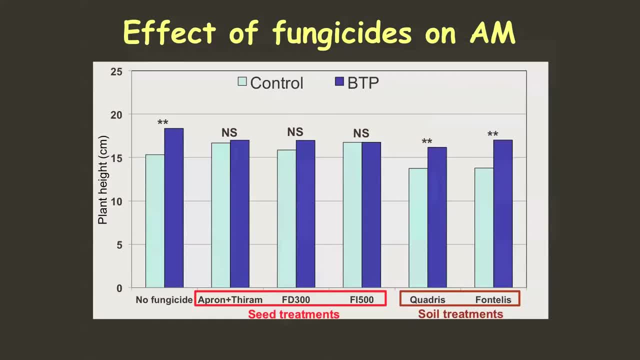 in onions And the control bars with no mycorrhizae were present in the soil of the light blue And this product, BioTerra Plus, was added to the soil. So in the absence of fungicides, you can see, we got about a 20% increase. 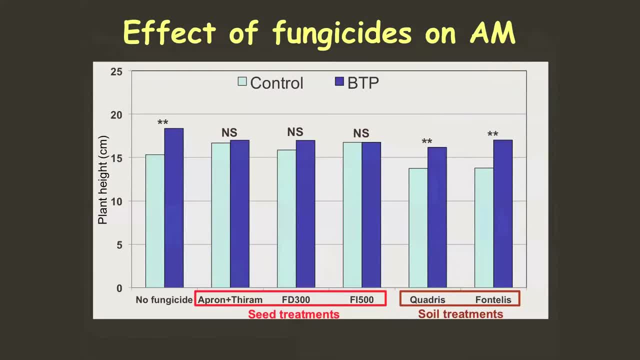 in growth of the onion seedlings. When we had seed treatments on the seed we negated that benefit of the mycorrhizae altogether. With Quadrus and Fontalis we still saw a benefit of the mycorrhizae When we 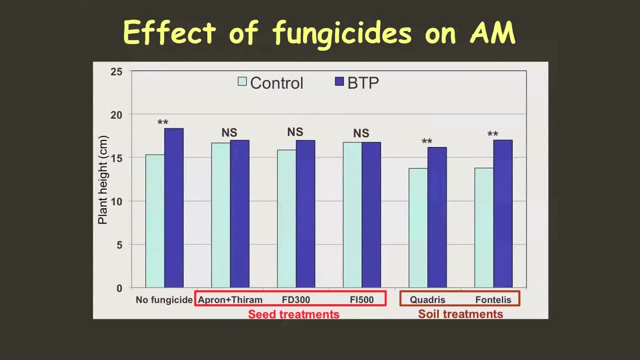 repeated this trial, we did see some inhibition of the mycorrhizae by Quadrus. So we need to take a closer look at this at the rates that are being used in agriculture. So I am quite concerned about how to address this issue. 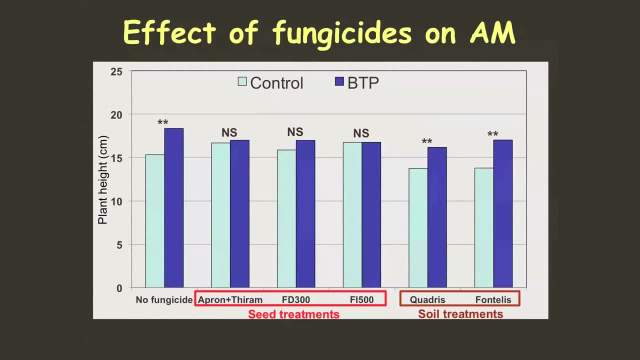 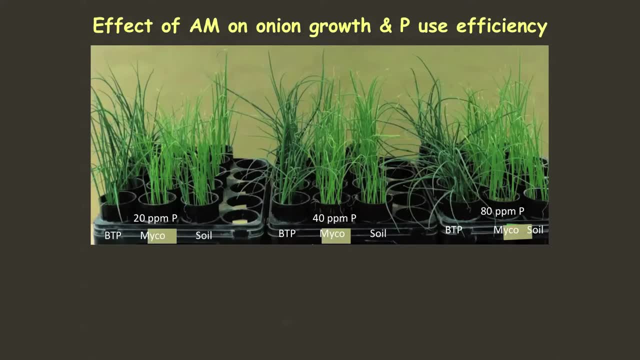 of seed treatments, which are critical for things like Pythium and so on and still maintain mycorrhizal benefit. And here's an illustration of onions growing and soil treated with a mycorrhizal product- a different mycorrhizal product- in the control. 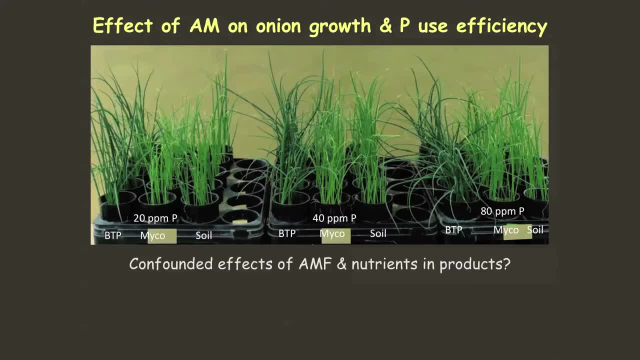 and you can see the big difference in growth of the onions. And I'm going to quickly go through this so I don't get behind. But here's a picture of a microscope from a microscope of the arbuscule in an onion root cell. 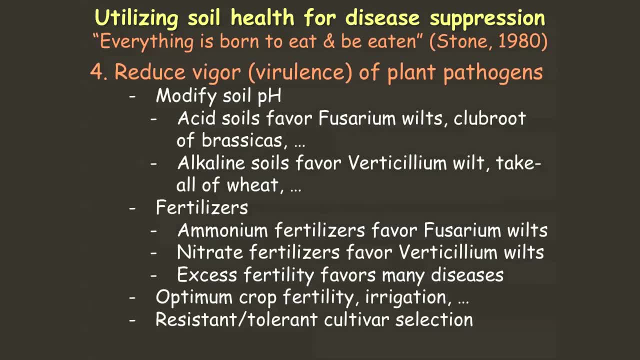 You can see it growing in there when we inoculated. Okay, the fourth category, reducing the vigor or the virulence of the pathogen through things like modifying soil pH I mentioned. we use limestone Acid. soils are very favorable for Fusarium wilts. 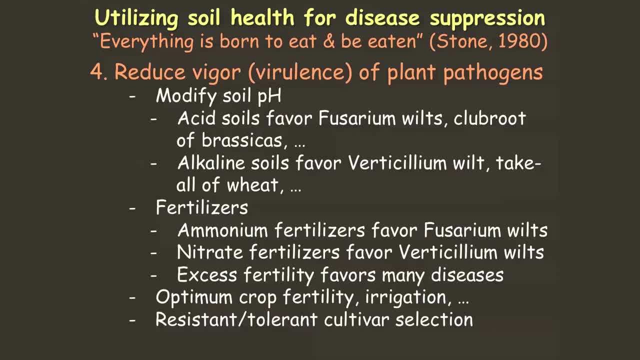 clubroot or brassicas, a number of other diseases. Unfortunately, alkaline soils favor Verticillium wilt, So it's a classic: mother nature tends to win out in the end. But understanding what diseases are prevalent in your area, what crops are? 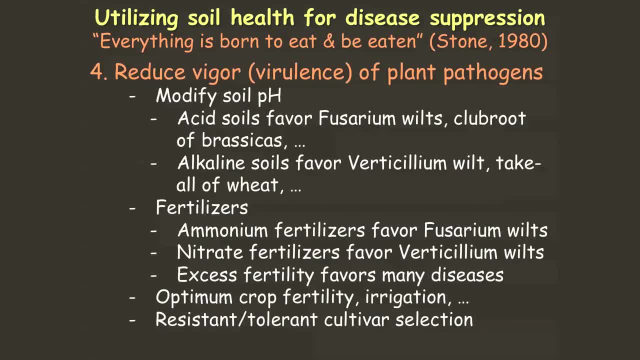 your major crops and what kind of soil conditions favor one versus the other is really important. Take all of wheat is favored by alkaline soils. Ammonium fertilizers favor Fusarium because of the acidification. Nitrate fertilizers favor Verticillium, That's. 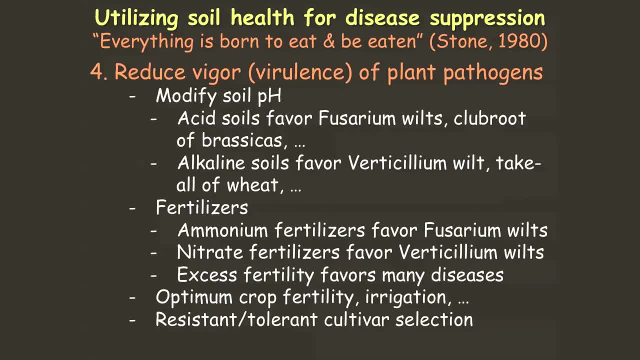 been shown repeatedly, Excess fertility favors many soil borne diseases. So optimum crop fertility, optimum irrigation, helping enhance that healthy status of the crop, is really important. And of course if you have access to resistant cultivars, that's again contributing to. 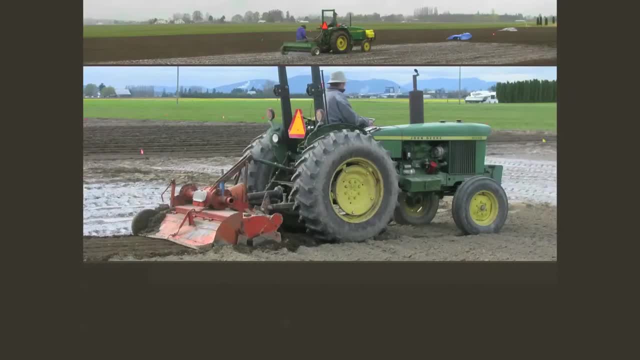 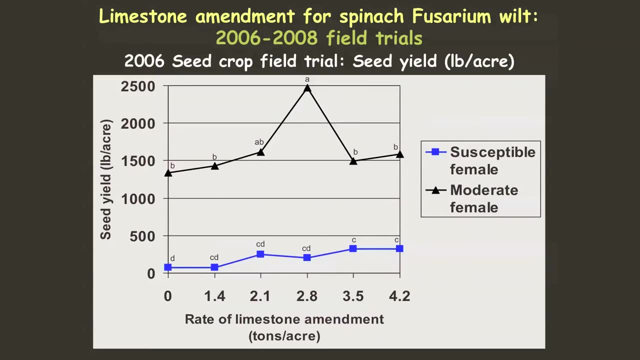 plant health. I mentioned that we've been looking at limestone amendments to control Fusarium And this is what happened when we put on rates of limestone from 0 to 4 tons- And look at this parent- It went from about 1200 pounds of seed. 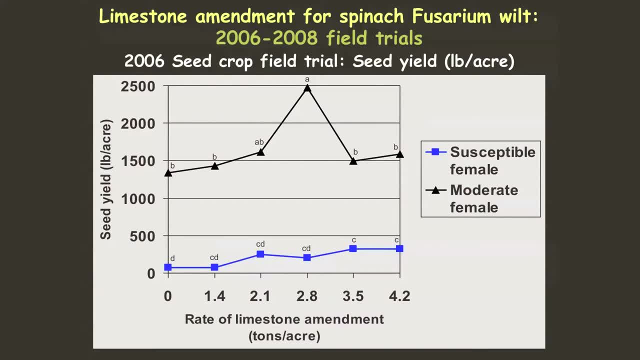 per acre to 2500 pounds of seed per acre by putting on about 2.5 tons of limestone And that's marketable seed yield. That's a pretty dramatic increase. This female is super susceptible down here. That actually represents a 300% increase. 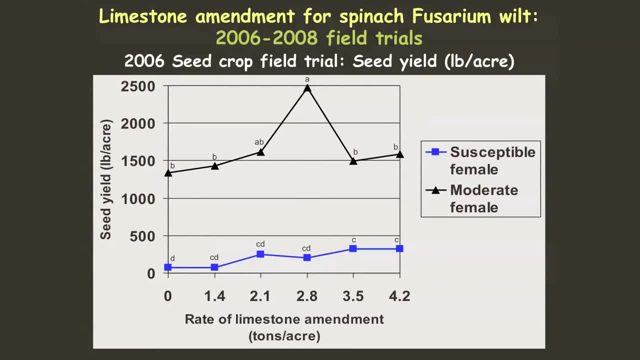 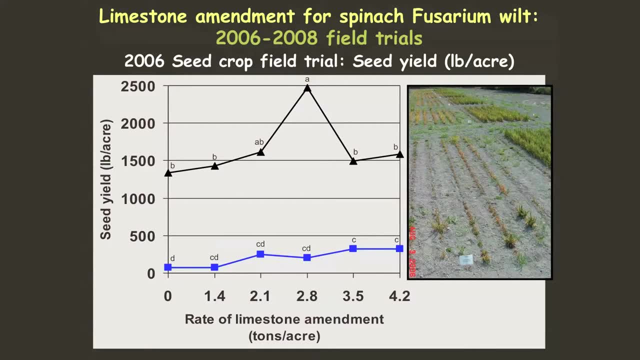 in yield, but it was so severely affected. Going from 0 to 100 makes a big difference, And this is what will happen if you grow a spinach seed crop on a 6-year rotation with no limestone. That's a susceptible female. 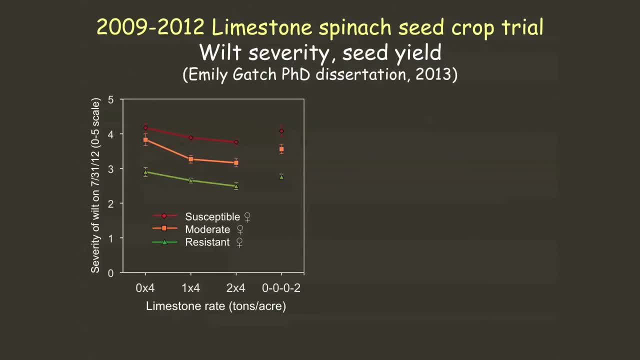 You just have nothing. We did this over a number of years looking at how limestone multiple applications can help shift our soil from very, very conducive to a little less conducive, And again you can see, over different rates of limestone, how the yield increases. 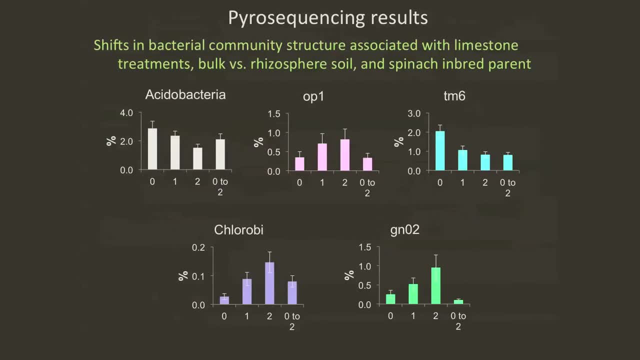 for the different parent lines. So we're working with growers. In looking at this limestone amendment to the soil, we also took a look at which bacteria are shifting in the soil as a result of putting on 0,. sorry, this mouse is hard to get. 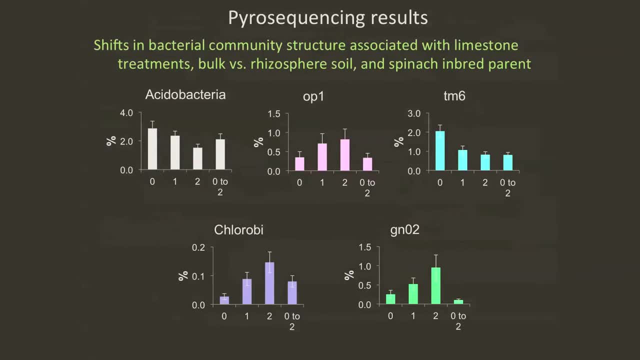 to work 0 limestone, 0 tons, 1 ton or 2 tons every year for several years. You can see some microbes become more prevalent, some become less prevalent and that's pretty well known that the bacterial shift is happening in response to this treatment. 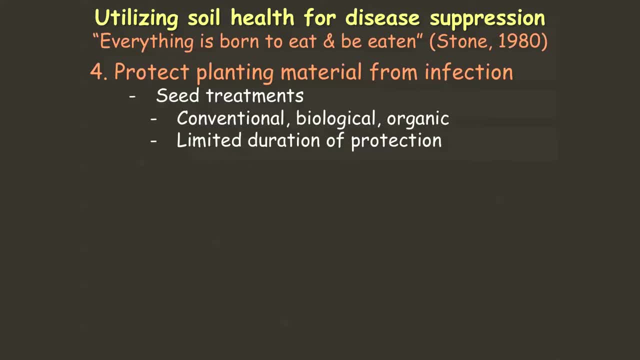 Okay, protecting plants from infection. Seed treatments: They can be very beneficial if you know you've got disease pressure in your soil- Conventional, biological, organic. They have a limited duration of protection and many of them aren't particularly efficacious. 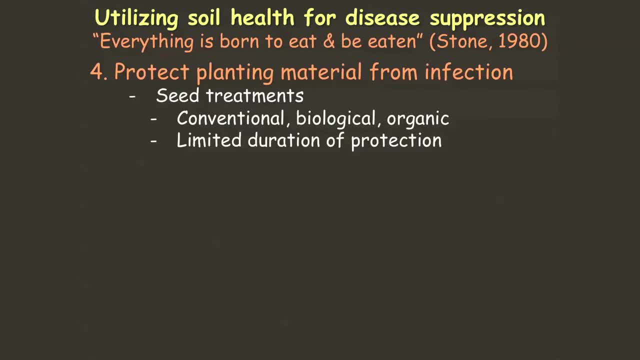 Unfortunately, particularly those organic treatments. We've done many years of trials and struggled to find highly effective organic seed treatments. Soil applications- Again, the range of products out there, range of methods of application. but recognize, any time you put a chemical in the soil you shift those microflora. 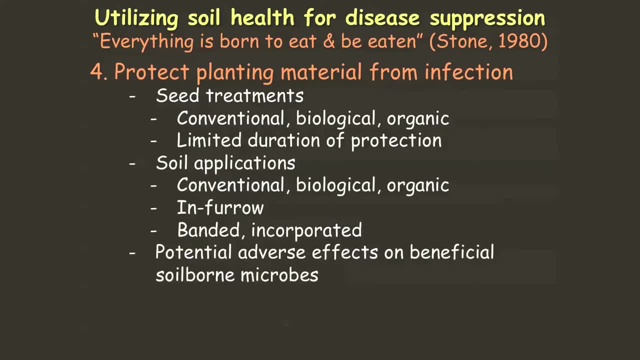 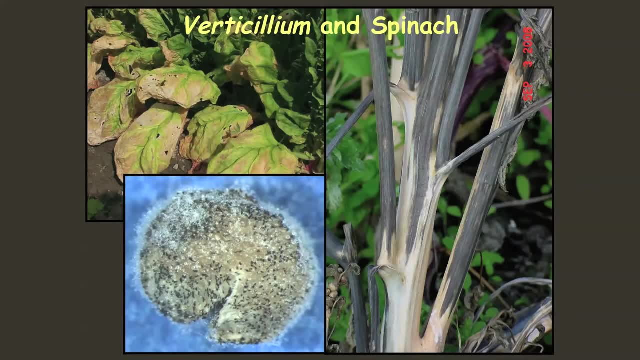 one way or the other, And so you can have potential adverse effects on beneficials like mycorrhizae- And I'll quickly finish up, Andy's going to kick me off here. One example we've been looking at is verticillium in spinach. It's very highly. 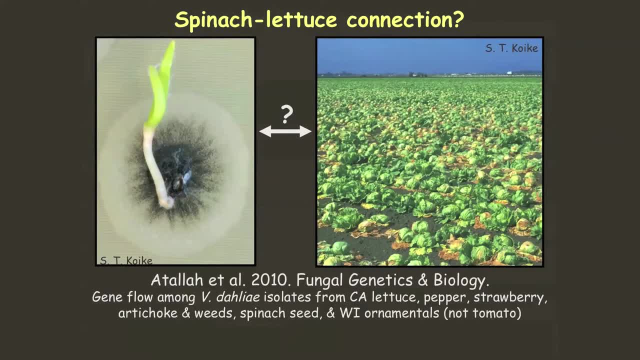 seed-borne in spinach and there's concern in California where a lot of the spinach seed produced in the Northwest gets sold, and spinach often precedes lettuce And the lettuce growers are blaming spinach seed as a source of inoculum that leads to these outbreaks of. 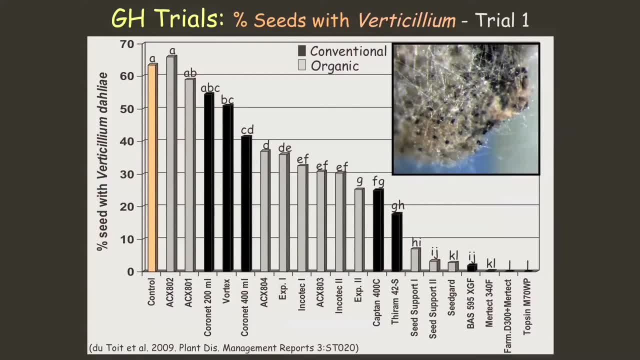 verticillium in lettuce, And so we've been looking at ways of treating seed. This is a level of infection, a natural infection in seed lots 64%. A wide range of products we've tested to see what can help reduce seed transmission. 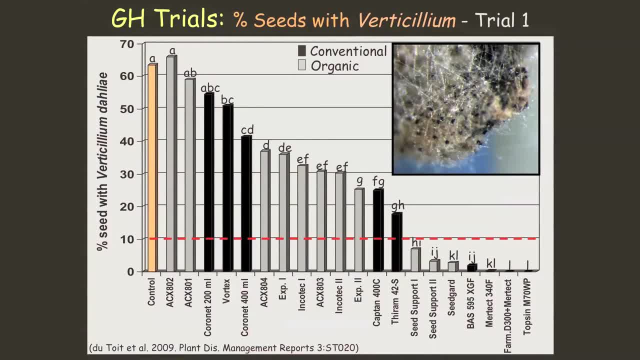 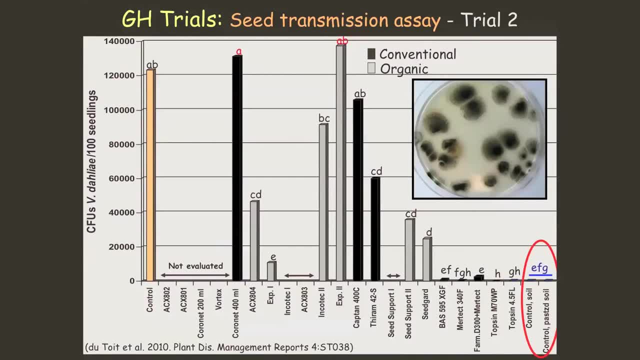 And you can see some very effective treatments down here that cut it down below the 10% threshold Mexico has for seed-borne verticillium. I want to mention that I'm going to skip through this because of time, but in doing this work with spinach seed, 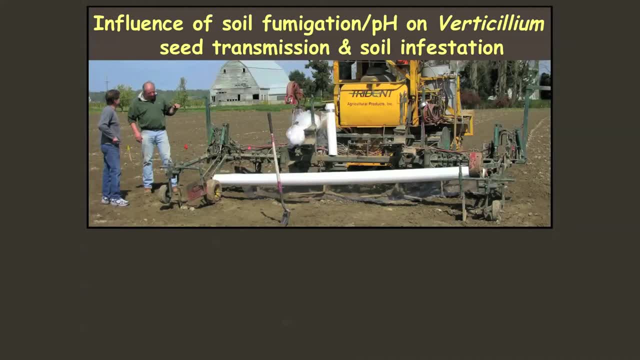 treatments in verticillium, we started to recognize that the soil microflora were playing a role in the rate of seed transmission. So we did a series of trials in Washington and California- baby leaf trials- where we fumigated or didn't fumigate strips of ground. 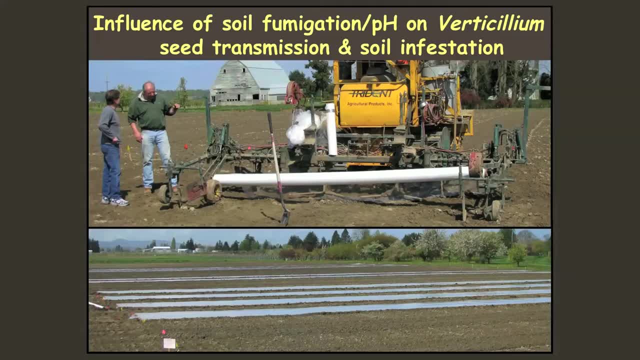 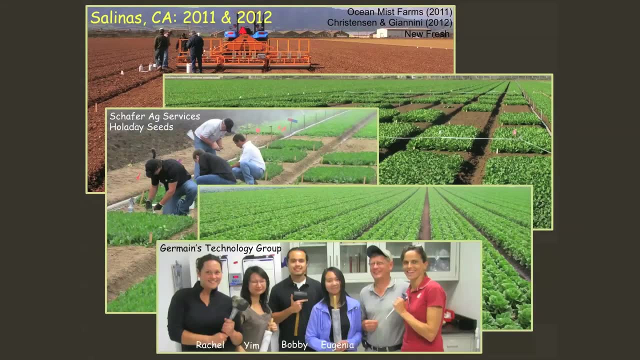 and planted out seed with these different treatments to see if fumigation might impact seed transmission. And this is a picture of our trials down in California where we were looking at spinach preceding testing for verticillium. And this is a snapshot of some data I want to show you. So this is 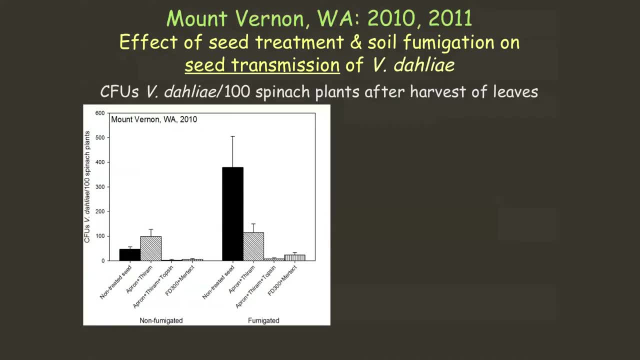 non-fumigated on the left and fumigated on the right with different seed treatments. If you look at the non-treated seed and the non-fumigated ground, we got about 40 colonies of verticillium per 100 spinach seedlings. 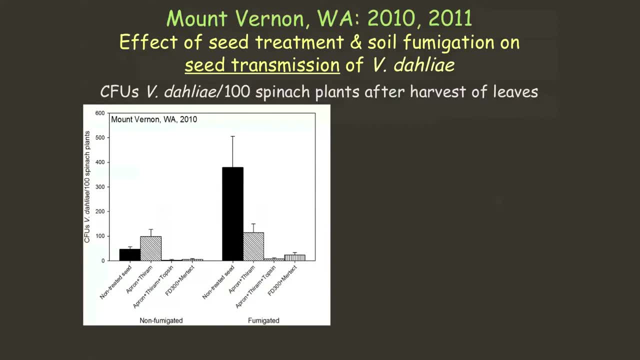 that seed transmission. Look what happened when we fumigated the ground: We got about a 5-plus fold increase in seed transmission rate when we put infected seed into fumigated ground, because you wipe out the competition And verticillium can establish very quickly. 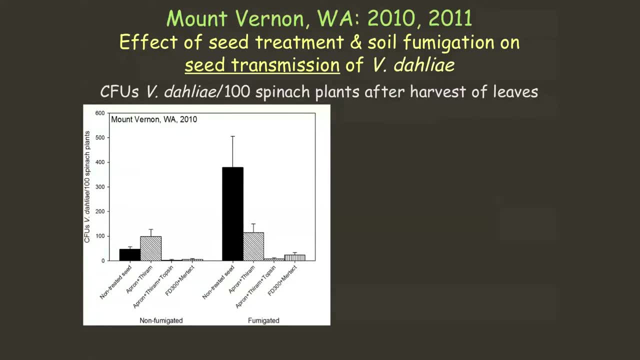 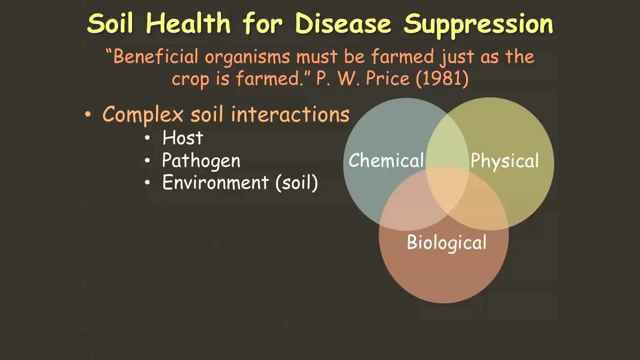 in the soil. So this is one of the negative aspects of fumigation you have to be careful about. I'm going to zip through because Andy's telling me This is my last slide. So thinking about soil health and disease suppression, it's complex, It's affecting. 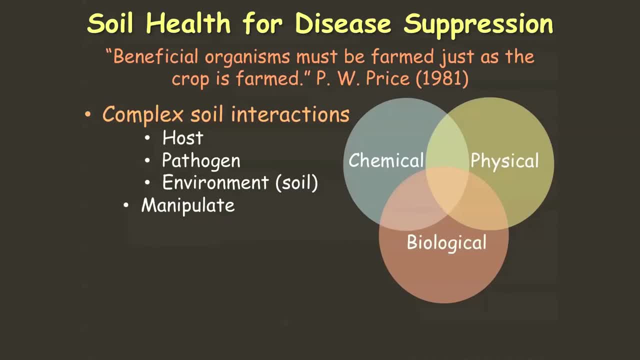 the host, It's affecting the pathogen, It's affecting the environment And it's important to try and understand the particular crops and diseases you're dealing with, to understand what can be manipulated, The specificity of that manipulation to your site and the potential double-edged sword. 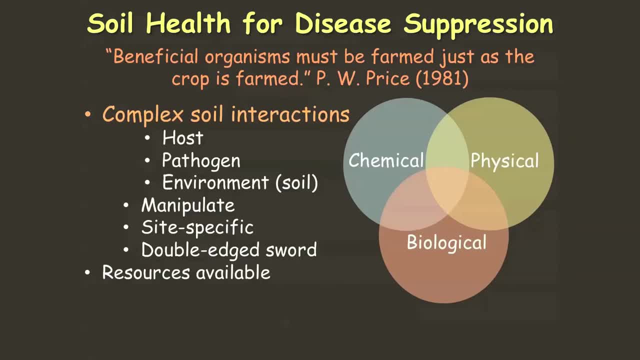 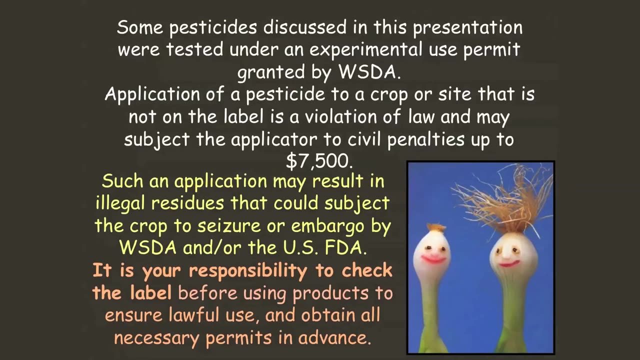 that we sometimes encounter with our practices and what resources are available to you. And the big question, as David said, is: is this all economically viable, these practices? That's still being addressed. Questions right now for Lindsay on her presentation. Any questions from the floor? 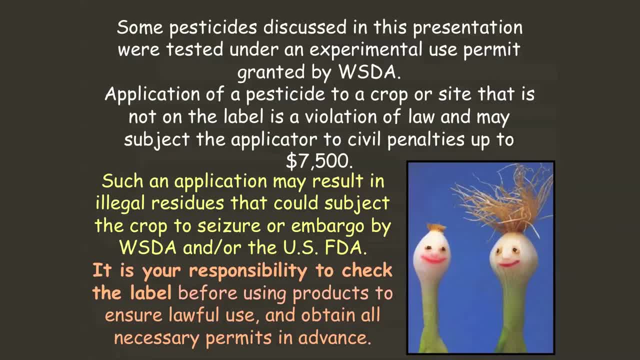 I've got some text questions but let's take them from the floor if anyone's got them first. Anyone have a question? Yeah, in those fumigation trials you were doing, had the thought crossed or maybe looking into the future doing an addition. 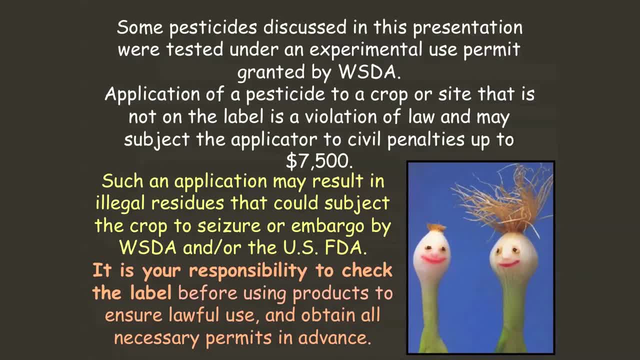 to adding some biological products quickly after that fumigation to help reintroduce some positive biology? Absolutely Yeah, It's a really good point And I think that's one of the beauties of a biofumigant type of crop- is you get that killing action? 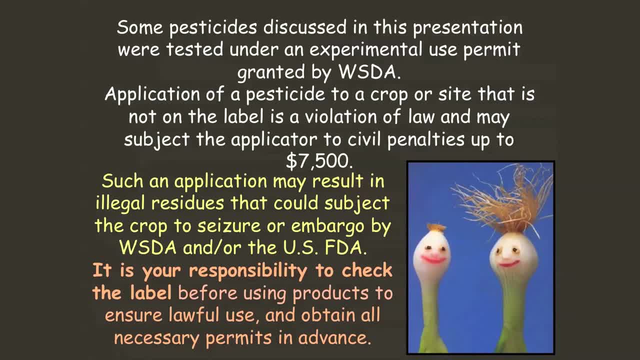 from, but you're also adding organic matter that really rapidly allows beneficials to colonize soil. Synthetic fumigants don't provide that organic matter, don't provide that benefit of quickly reintroducing things. So there is a lot of interest in looking at. 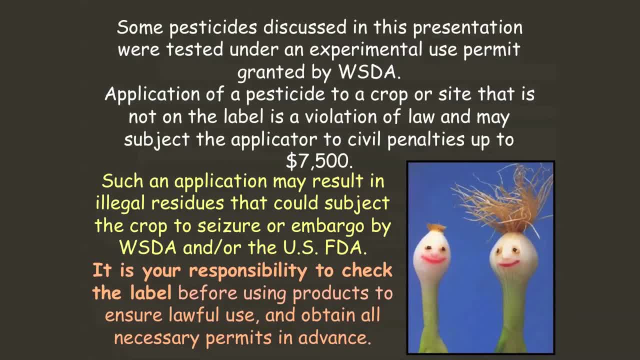 applying biologicals to the seed. So when you are in a fumigated, sterilized soil situation you introduce beneficials to rapidly establish in that soil and compete with the pathogen. So definitely that's a lot of what effort is going on into organic and biological. 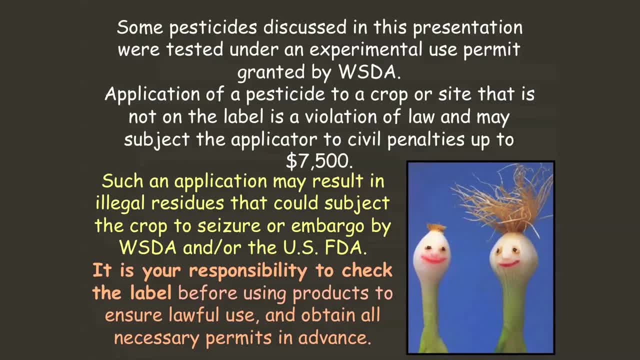 seed treatments. Okay, here's a text question. Will the spinach seed fields still work for spinach crop versus the seed crop, since the crop would be shorter days in the soil where the spinach would still be taken out with the fusarium? Absolutely, I understand the question and this is. 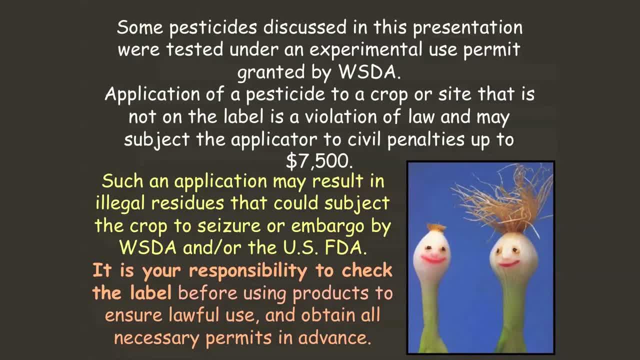 a huge controversial issue because when I started working on spinach and discovered verticillium was causing these losses, no one even recognizes it as a disease of spinach and yet we found it was present on 90% of the seed lots that we tested. 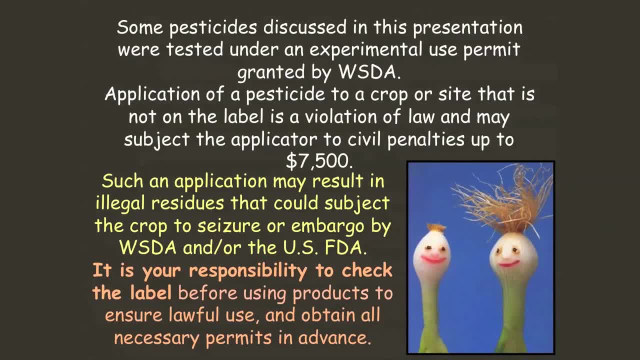 And part of the reason is when you plant that seed out for baby leaf crop or even a processing crop, it stays in its vegetative state and symptoms do not show until you initiate bolting. So no one who works with California or Texas or Arizona and spinach 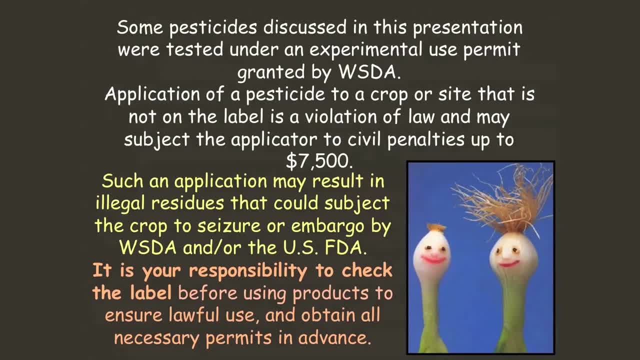 had ever heard of verticillium being an issue until they. if they let those plants go to flower- which normally you can't because the seed length is too short down there- symptoms will show immediately. But once we published this paper documenting how verticillium works in spinach- 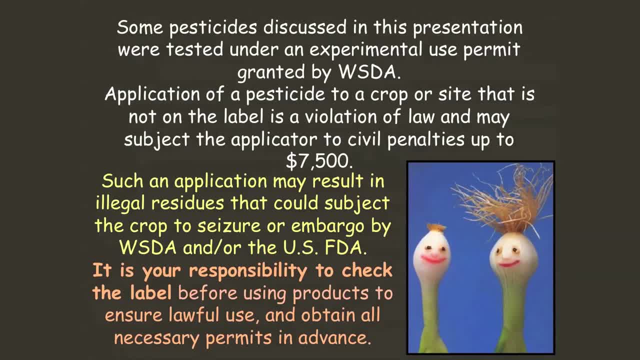 the California spinach industry read it and said: oh, you guys are the source of inoculum for our lettuce crop, because lettuce- head lettuce- right when you're harvesting it's bolting, It's going into that final shift to reproductive stage. So unfortunately, 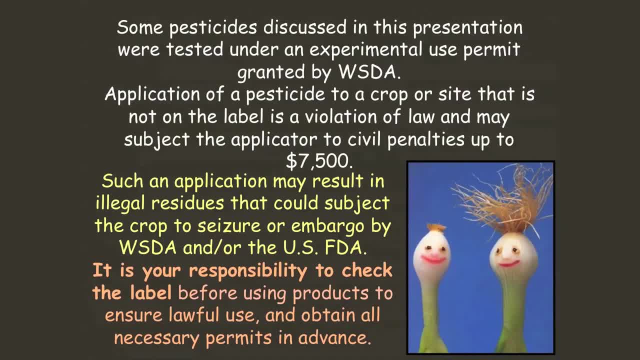 verticillium in lettuce shows up two weeks before harvest when it's bolting. And they started blaming everything on the spinach seed industry. So I've been playing really hard game trying to figure out how to help the spinach seed industry since I opened. 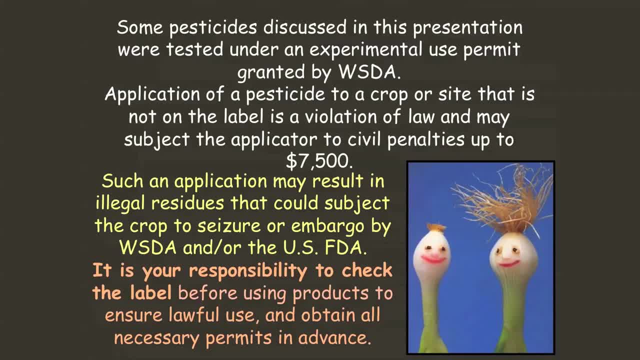 the can of worms in the first place? In your studies with the forzerum wilt and the spinach, did you see any difference between open pollinated and hybrid as far as the effects of the wilt? So you all had the question. obviously you have a microphone, but 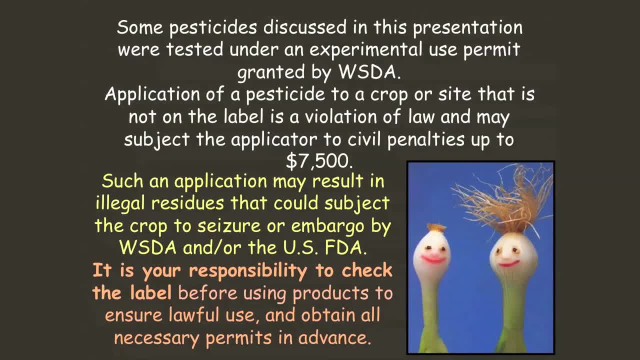 we see a wide range of differences in susceptibility of the parent lines, The OPs. some of them are very susceptible, some are not. It tends to not the inbred lines, because they're inbred when they're susceptible. they're horrendously susceptible. 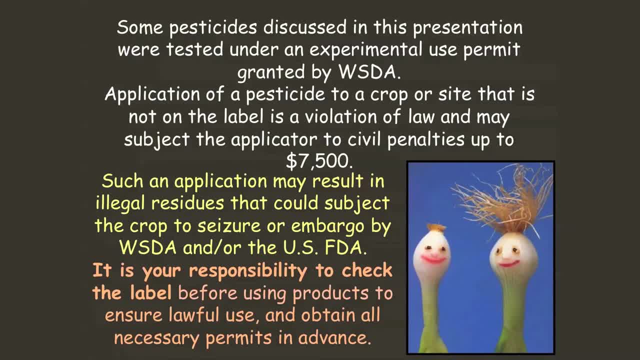 So we tend not to see quite that degree of susceptibility in the OPs. Most of the seed production is not OP. on the west side there's a little bit. They can still suffer from forzerum wilt, but you tend not to see that very. 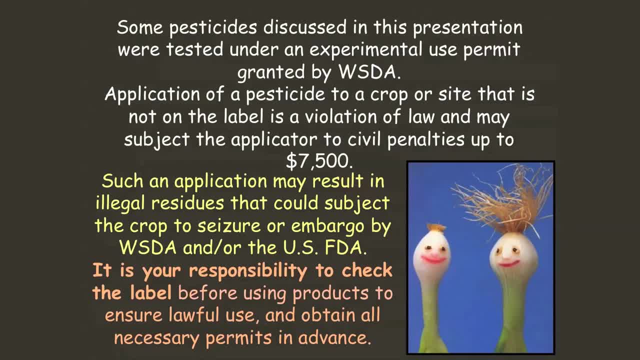 extreme degree of susceptibility that we see in the inbreds. Another text question: does the form of nitrogen, aluminum versus nitrate in the soil, aside from pH generally, influence disease? Kind of big picture. I'm wondering about nitrification inhibitors. 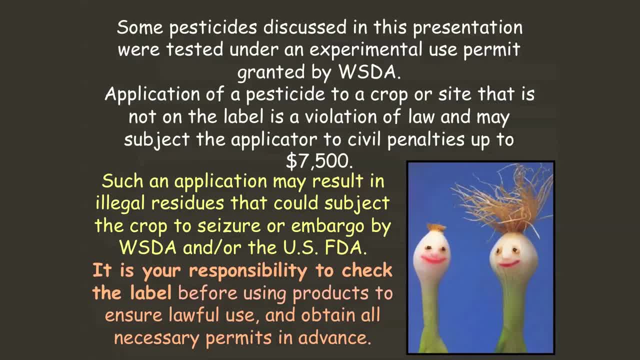 It definitely does and it depends on the pathogen. I mentioned that ammonium fertilizers are very conducive to forzerum wilts and nitrate fertilizers promote verticillium wilts And that's been shown on potatoes, it's been shown on tomatoes, it's been shown on 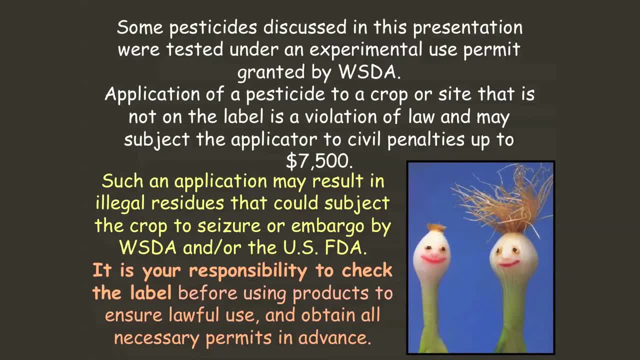 a range of crops that get both verticillium and forzerum. Alkaline soils tend to favor verticillium, as do nitrate fertilizers, And opposite for that was verticillium, opposite for forzerum. 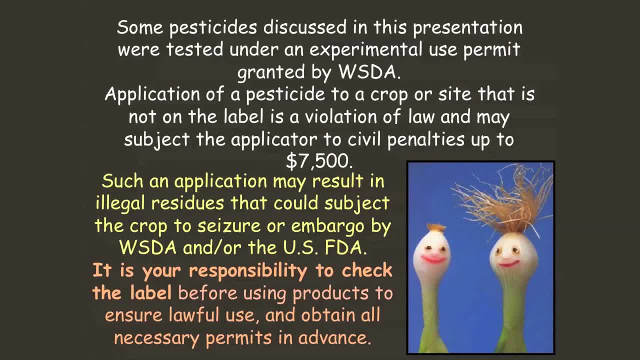 So form of nitrogen can be very, very important. We actually did a trial the first year of our PhD students. she tried looking at nitrate versus ammonium, because our growers use 1152-0, and she put out a comparison trial with a can 27,. 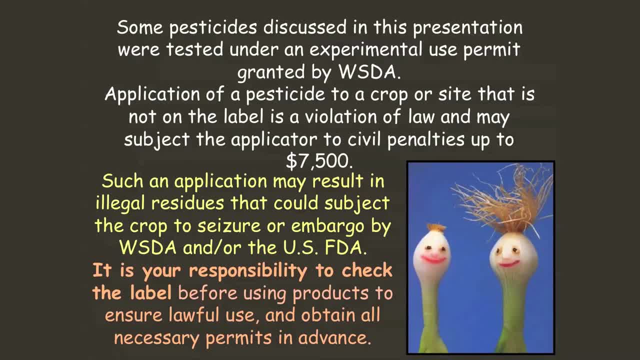 but we get, you know, inches of rain in the spring and everything leaches straight out And we realize it'll never be a solution for western Washington because nitrate leaches so quickly, But it definitely has an impact. Other questions on the floor? 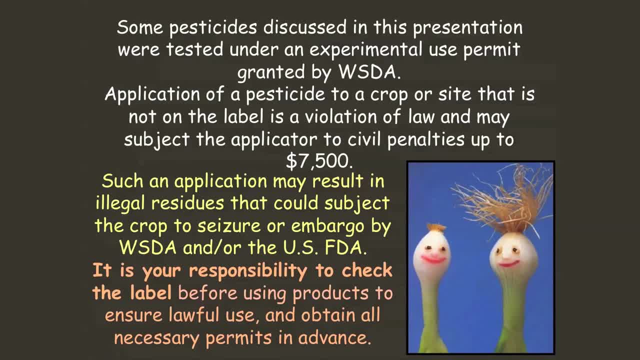 Got one more text question, Okay. This one is asking whether mycorrhizae testing is reliable. First of all, is it an available service for the average person and is it reliable? It's a really good question and I'm relatively new. 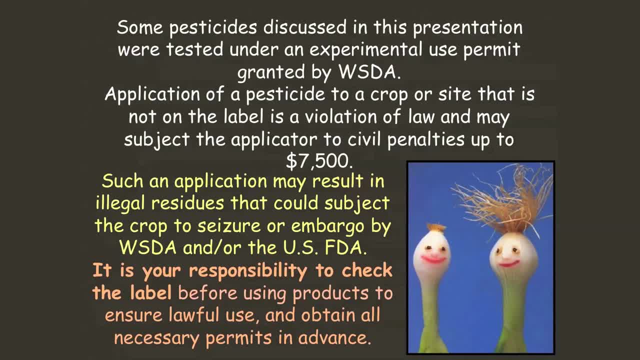 to mycorrhizae. but one of the difficulties of mycorrhizae is that it's a- it's what we call an obligate fungus or obligate fungi. They don't grow in a petri plate, so you can't take soil. 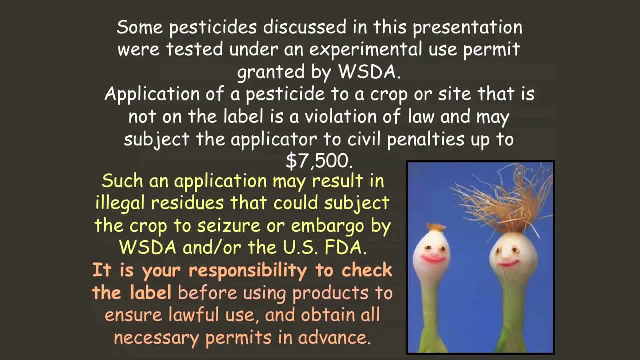 and plate it out. They won't grow. They can only grow on the host plant. So the way that we test soil for these mycorrhizae is: we take soil from the field, put it in the greenhouse and grow onions and then, when they get to a certain stage, 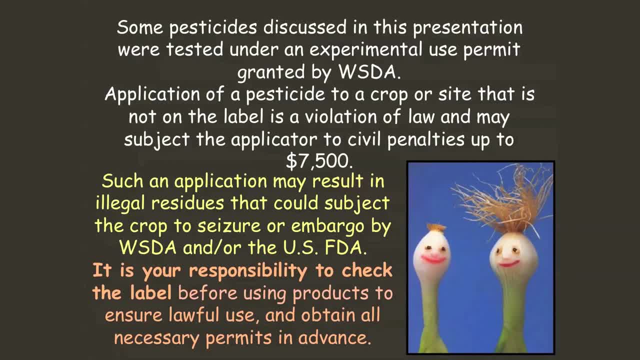 with enough roots. we take those onions and we stain the roots and look on the microscope to see the degree of colonization. You can also test for mycorrhizae using DNA, a DNA test, where they'll extract DNA from the soil and use specific 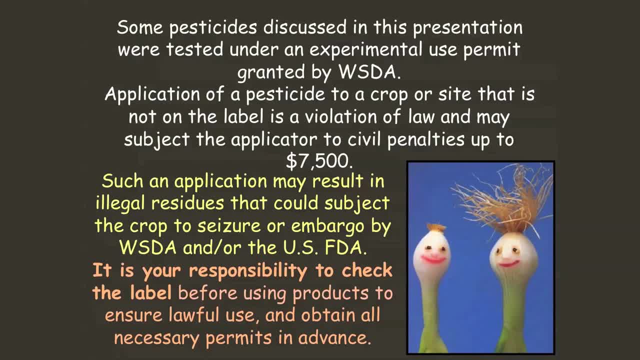 probes that are designed to the fingerprint of mycorrhizal fungi, So that's another way you can do it. I haven't heard about extensive testing services available for mycorrhizae, but I can look into that. David, I think that's an important point. 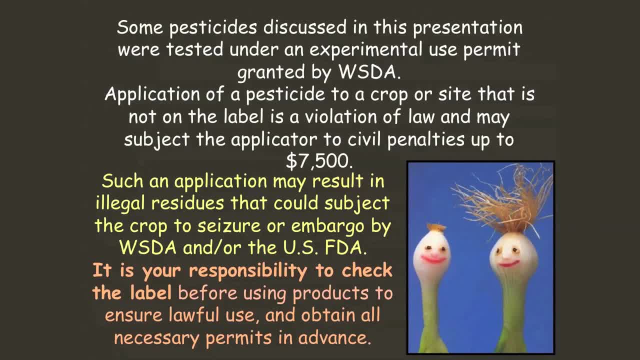 Could you dig a plant from your field and test those roots, for example? Yes, you can, So that instead of trying to inoculate your onions, You have to find a lab that can do. you can do DNA extraction from roots or from soil, or you can stain the roots.